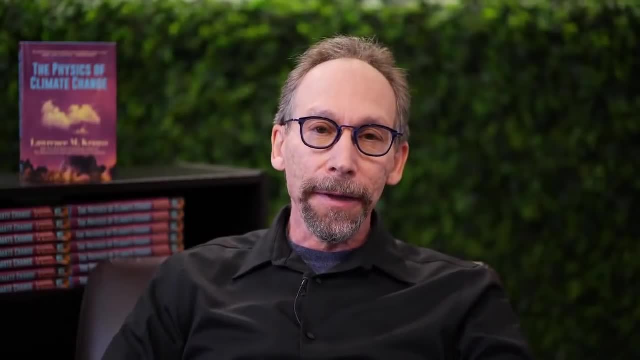 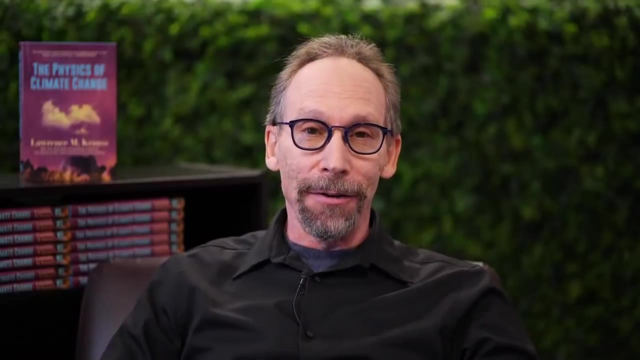 Hi, I want to thank first Susie Jamila and Think Inc for helping us get the word out about the Origins Project Foundation lecture that you're about to hear, And I want to welcome you now. I'm Lawrence Krauss and I want to welcome you to the very first Origins Project Foundation live interactive public lecture, which you're now watching. 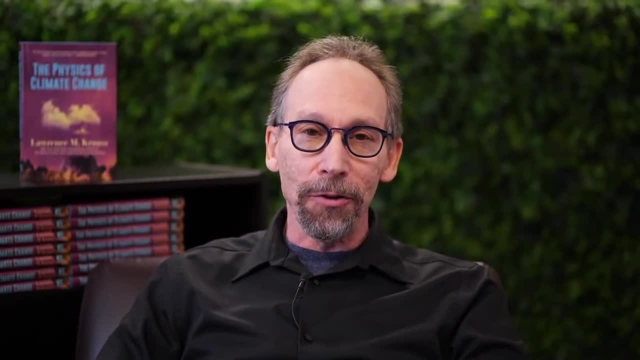 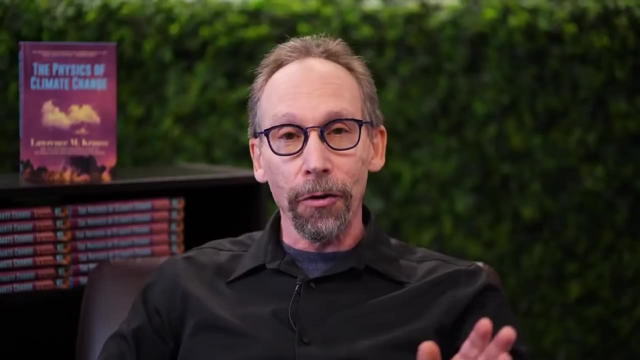 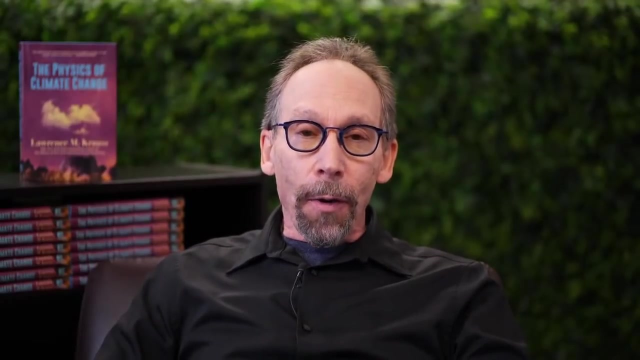 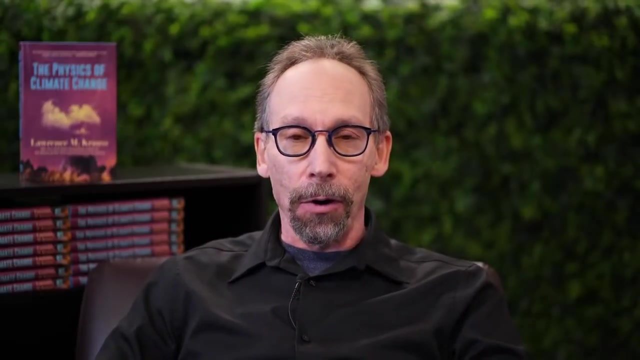 And it's very exciting for us to be able to do this. As you know, this lecture is being provided free online for all those who registered or anyone who happens to show up at the YouTube page or our web page right now. Also, after the lecture, for those who bought premium tickets, we're going to have a question and answer period, which will be an hour or so. 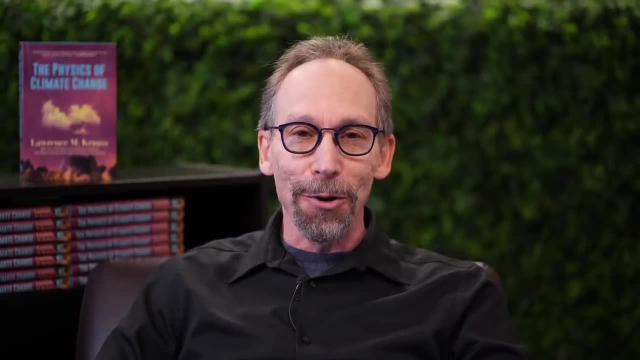 And it'll begin about 10 minutes after the lecture ends, giving you time to go to the bathroom or whatever, And all of those who signed up with premium tickets should have gotten an email by now with the Zoom link And if you're so compelled that you want to purchase a premium ticket while I'm talking now, there are still some available. 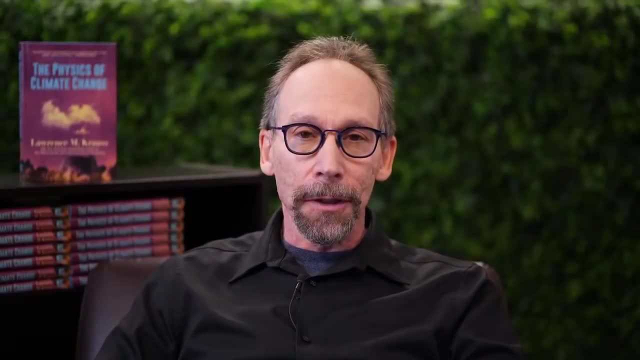 And you can do that, And if you do that during the lecture, you'll get, before the event begins, a Zoom link So you can hook up and I'll be able to see you and you'll be able to see me and we'll be able to chat and I'll answer questions about the lecture. 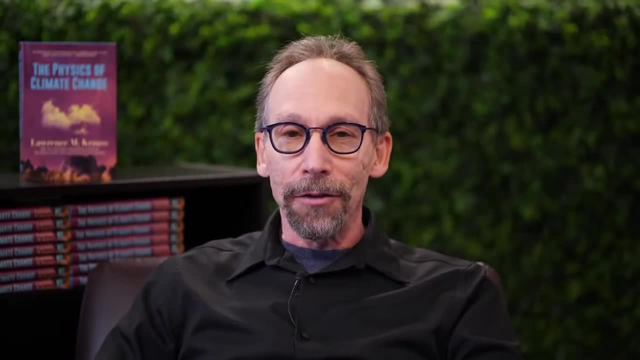 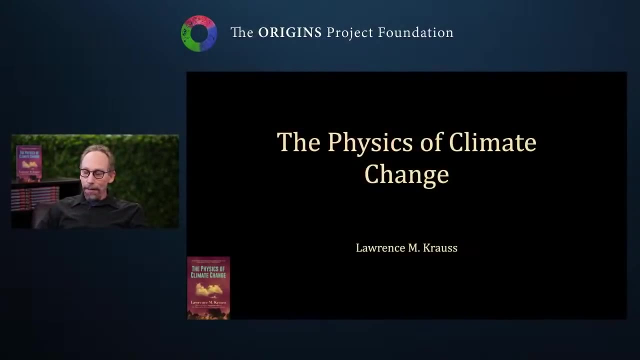 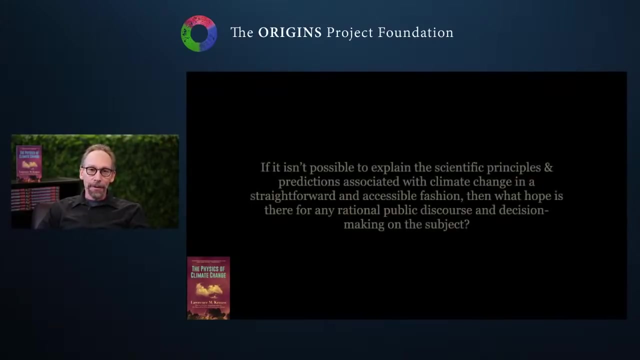 Okay, so now I guess I just want to go right away To my slides and we'll begin the lecture now. So there we go. Okay. One of the reasons I wrote the book, that I did, and one of the reasons we're having this lecture, is this fact: 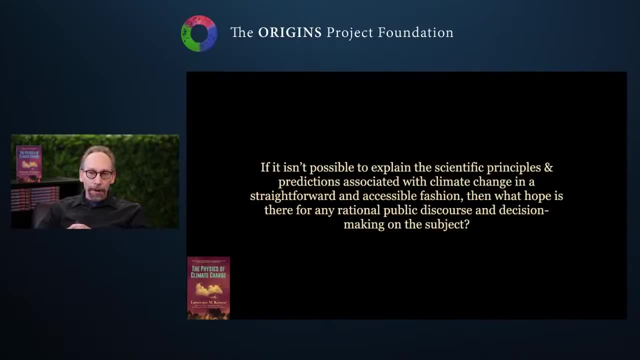 That if it isn't possible to explain the scientific principles and predictions associated with climate change in a straightforward and accessible fashion, then what hope is there for a rational public discourse and decision making on the subject? The Origins Project Foundation was created for many reasons. 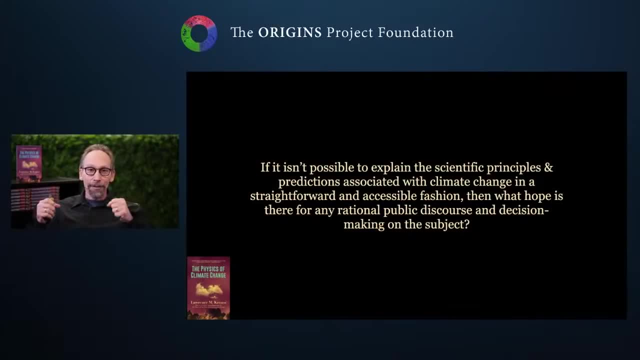 To get people excited about the universe and about the real universe and not nonsense, But also to energize them to help address the challenges we face in the 21st century, And certainly climate change is one of those, And the idea is to provide people a basis for rational discourse. 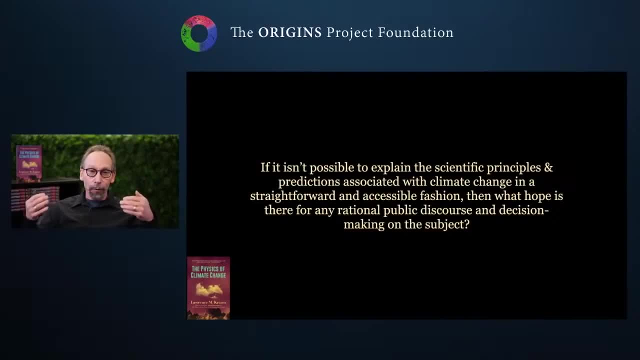 And really healthy democracy depends on the fact of having an informed electorate. So one of the reasons, as I say, I wrote the book and one of the reasons we're doing this is to give people information That will help you talk to your friends and decide how to act. 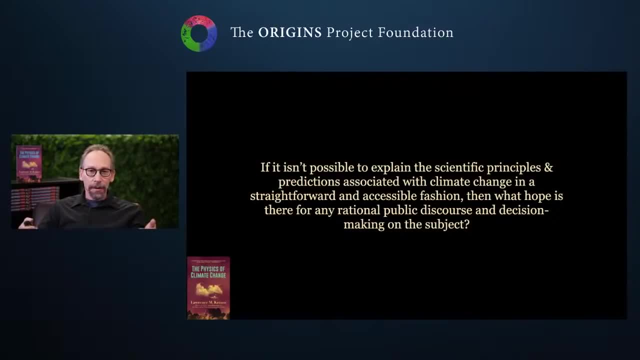 The scientific information. I'm not going to discuss policy At the end I'll talk about possible policy issues, But really the idea is to provide you with the information you need to make your own decisions about how important this issue is for you, your family and your community. 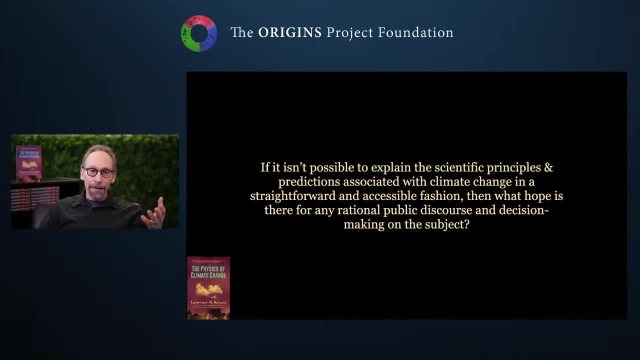 I'm not a climate scientist. I'm a particle physicist and cosmologist by training, But my feeling was that if I couldn't be able to translate it into a language that was understandable by everyone- having a lot of experience doing that with a number of books- then what hope was there? 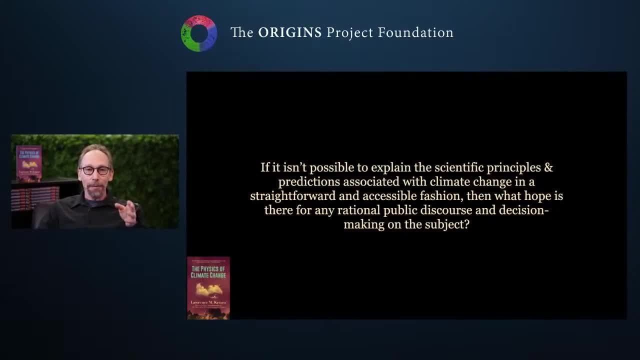 And, of course, I've had a lot of experience over the years. I've been tutored by many, many colleagues who are in climate science. I was chairman of the board of sponsors for many years of the Bolton, the Atomic Scientists that ran the Doomsday Clock. 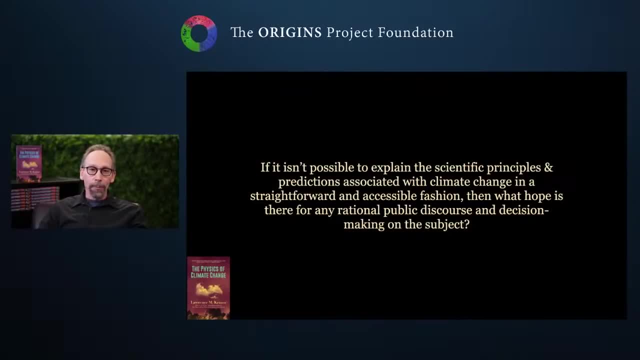 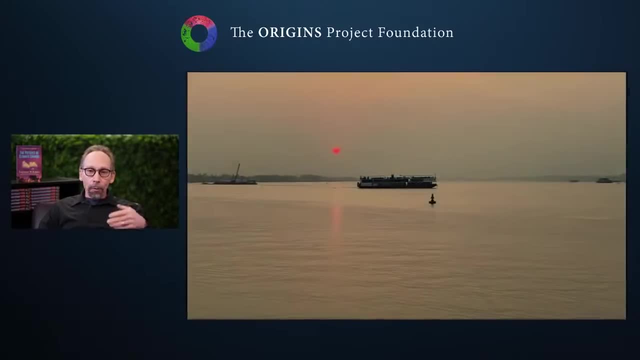 And we used to have a Doomsday Symposium every year where we talk about these issues And I'd hear about them. So this has been bubbling up in my own mind for quite a while, But where it really began for me is recently, about a year ago. 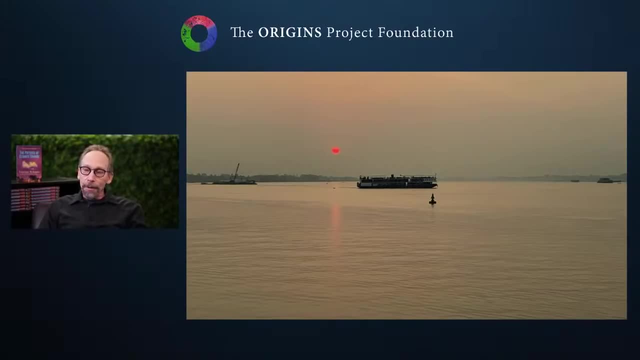 A little over a year ago I took a group through the Origins Project Foundation to the Mekong Delta in Cambodia and South Vietnam- And this is a picture I took from our riverboat- And it was a remarkable experience And they're beautiful countries. 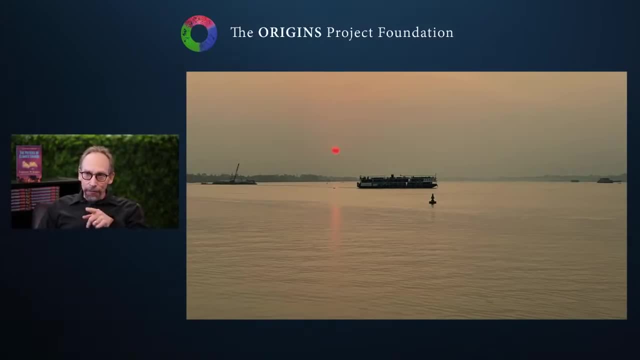 And the cultures are just amazing. And if you look at that picture, you can see on the left side a sand barge digging up sand from the river bottom And they're everywhere on the delta And we'll talk about later the impact that those are having on the river and exacerbating the effects of climate change. 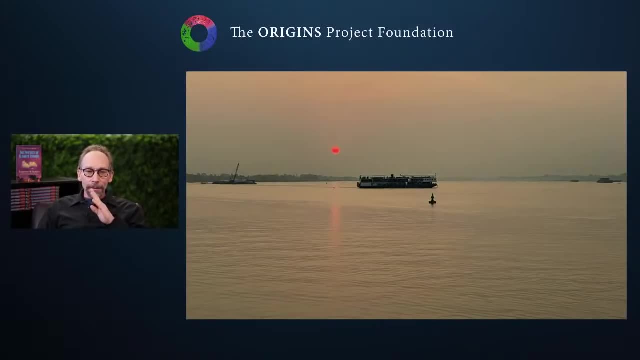 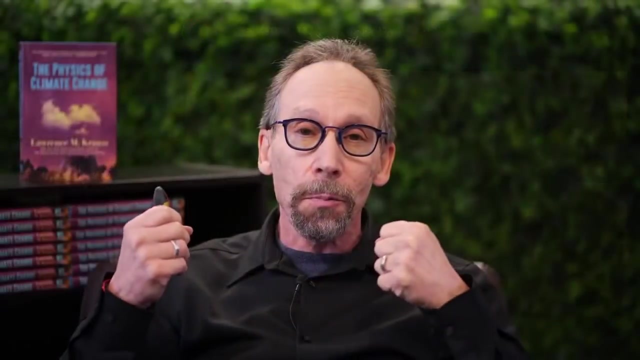 And really what hit home for me was that South Vietnam in particular is kind of a perfect storm for climate change, And when we think about climate change it often seems like it's out there And not where we are. But having visited that region and met the people and seen the wonderful cultures and how they've survived so beautifully after many, many problems in the 20th century, wars and genocides- 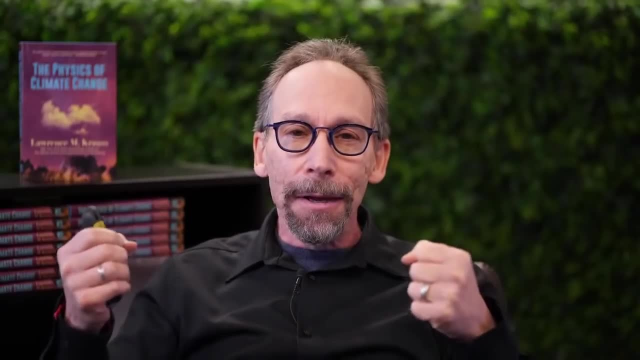 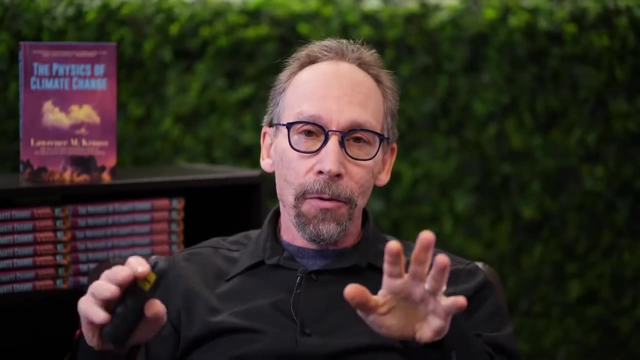 and come out of it hopeful and happy. the thought that they will be exposed to potentially a more severe challenge, not of their own making, really hit home for me, And I'll return at the end of this lecture back to the Mekong to talk about that. 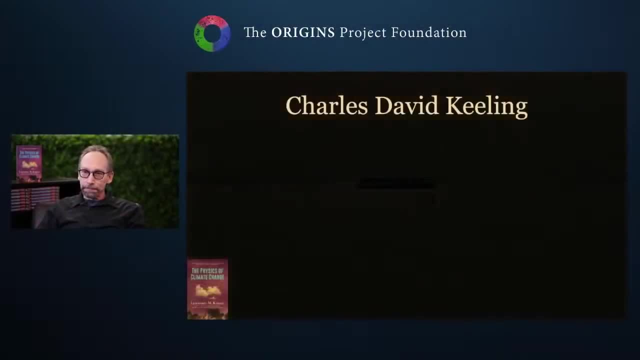 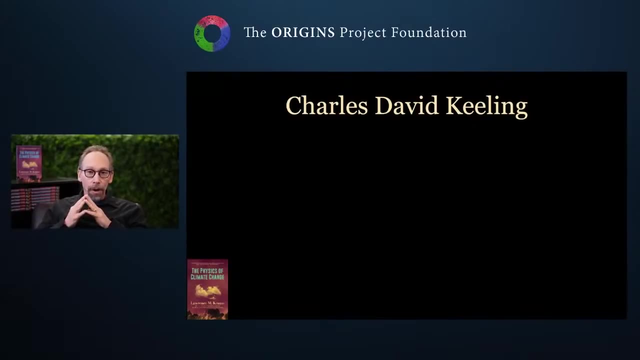 Thank you. Thank you, Let's go to the next slide. In the modern era, the recognition that greenhouse gases could affect climate really began with Charles David Keeling, who was at the time a postdoc at Caltech. He was a geochemistry postdoc. 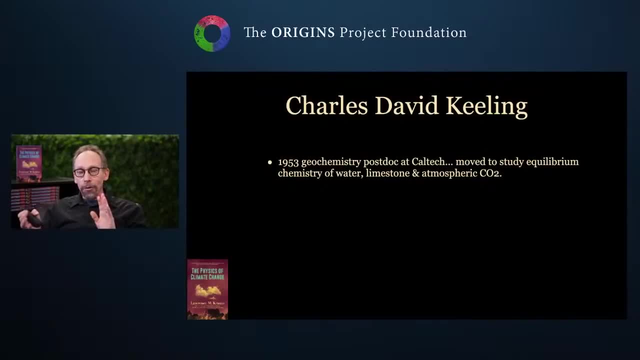 And he was working on actually issues having to do with uranium. But he moved his work to study the equilibrium chemistry of water, limestone and atmospheric CO2. And to do that he had to build a detector. He had to build a detector of atmospheric CO2.. 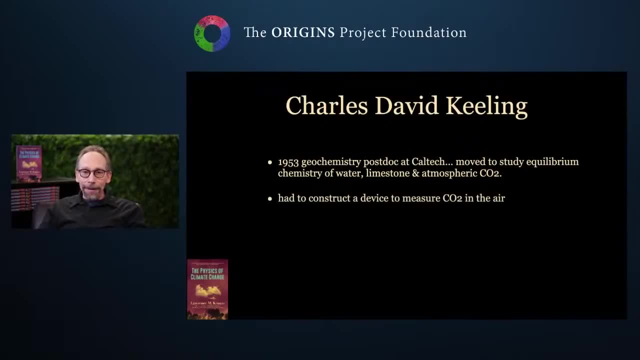 So he did that, He constructed that And he decided to test it out in Pasadena. But everywhere he went in Pasadena he kept getting different readings, depending upon whether he was near an industrial site or far away from an industrial site. So he decided to take the detector farther away. 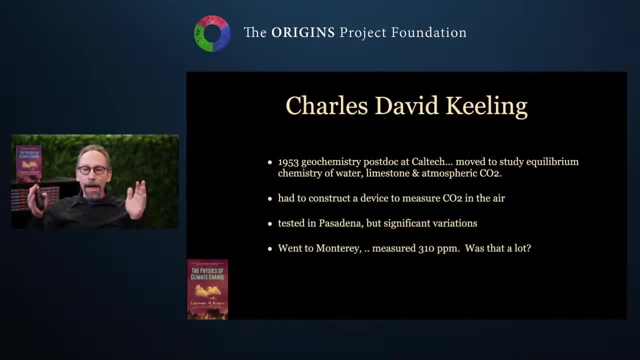 He went to Monterey And he measured a value of 310 parts per million for carbon dioxide in the atmosphere. Now the question is: is that a big number or a small number? And with a single number it's hard to know. 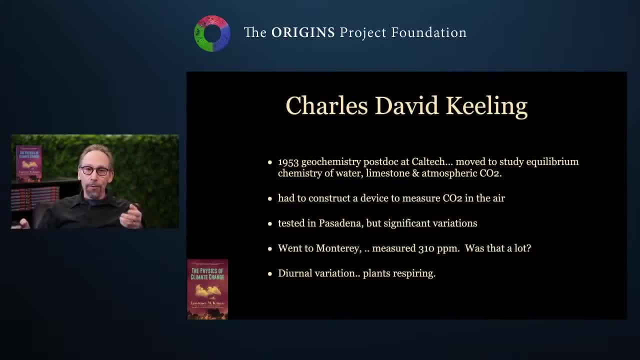 And what he did do right away that surprised him was he measured a different value during the day compared to during the evening And, of course, later on he realized after reading a meteorology textbook that he was getting the local region. he was getting the air from plants around him respiring, taking up carbon dioxide during the day and, in some sense, releasing it at night. 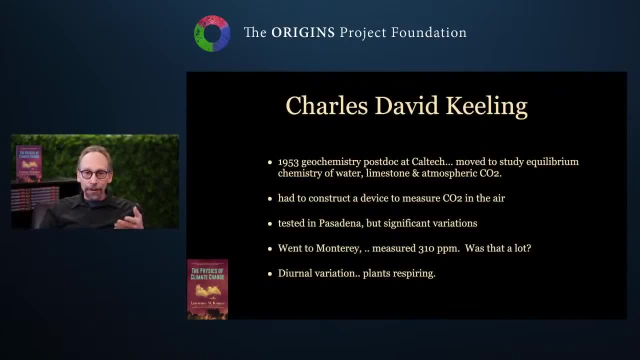 And so he saw that, And so he saw that diurnal variation which in some sense was convincing him that at least he was measuring things, but also convinced him that you really have to get away from that local pocket where he was in a valley to measure a global number. 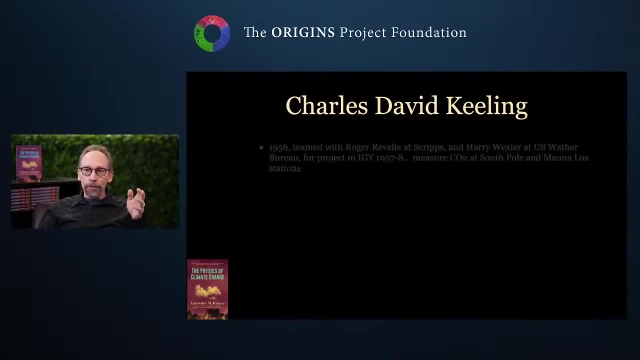 And around that time, a little bit afterwards, two oceanographers and meteorologists, Roger Revell at Scripps and Harry Wexler at the US Weather Bureau, approached him for the question. And Roger Revell approached him to do a project for the International Geophysical Year in 1957-58 to measure CO2 at the South Pole and at the Mauna Loa Station in Hawaii. 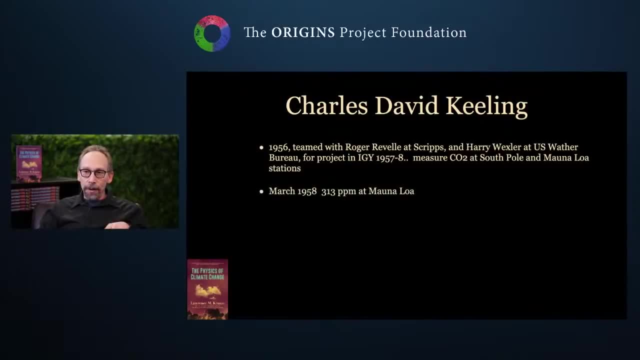 And they collaborated to do that, built detectors there and in March 1958 made the first measurement at Mauna Loa of 313 parts per million. That established what has become what is really an important day in human history For society, because it's probably the most significant continuous terrestrial science project ever done. 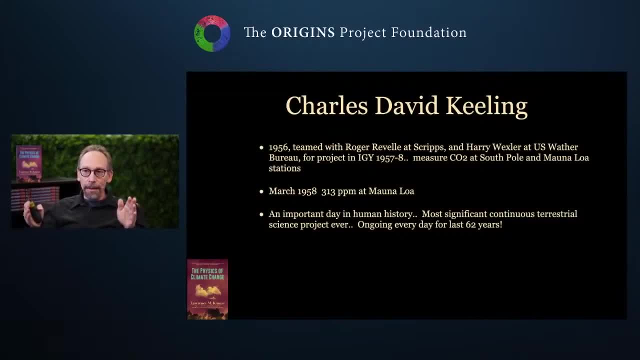 Every day since that day in March 1958, that observatory has measured carbon dioxide in the atmosphere for the last now 62 years, almost 63 years now, In fact, this month 63 years. And one of the things they discovered, which, again, was a surprise, 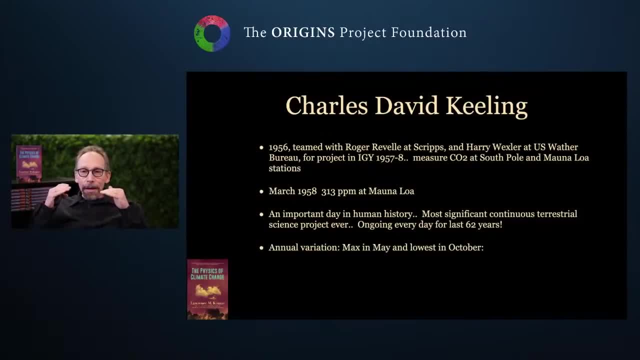 To Keeling. It's kind of fascinating. They measured that the carbon dioxide had a maximum in May and a minimum in October each year as they began to measure it And tried to understand that. And let's go back to the slides again. 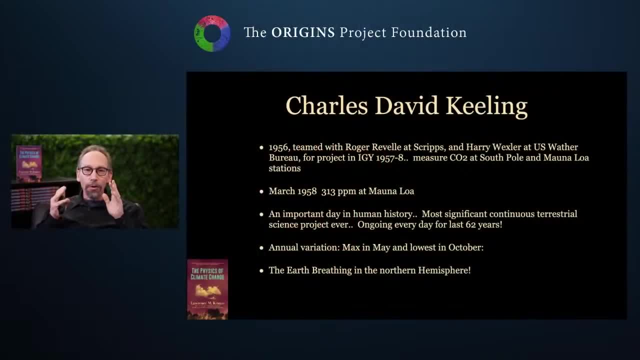 What he discovered, as he described it, was the Earth was breathing in the Northern Hemisphere, in Mauna Loa. Because what happens during the summertime? plants are taking. as plants are growing, Plants are taking up carbon dioxide And then, starting in October, they begin to release it as they release their leaves and die down. 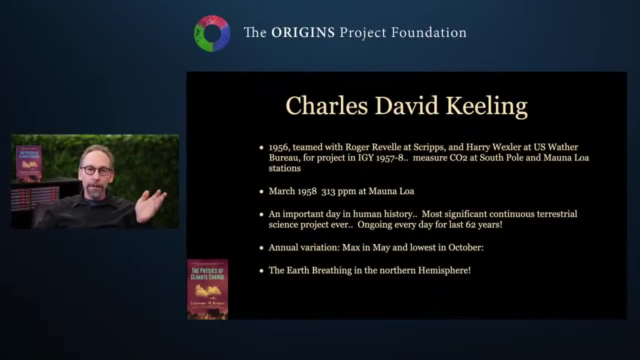 And so really, he saw, as he described it, the Earth breathing. And since that time- well, that's been observed a number of times since then, But in that period- from 1958 to 1960, it was observed in the South Pole that the number went up from 311 to 314 parts per million. 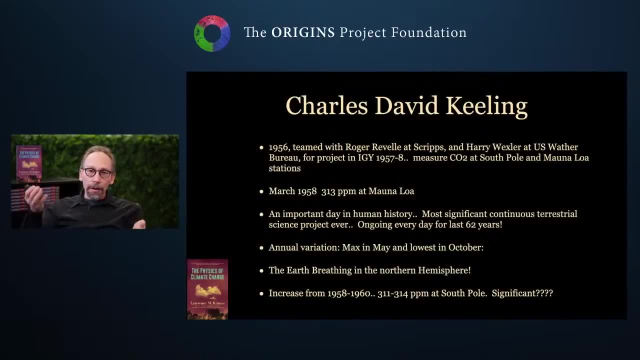 Now, that's not a lot, And given the uncertainties in various things, the question was: is that a significant reading of increase? Well, it wasn't clear at the time, But since then it's clear, And here is what has now become called the Keeling curve. 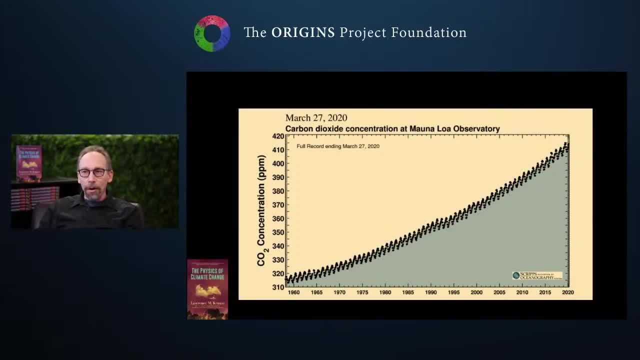 Which is the daily record of carbon dioxide concentration in the atmosphere at Mauna Loa every day between that period in 1958 and today. Well, that was taken March 27, 2020.. And the reason that number is there? That number is there. 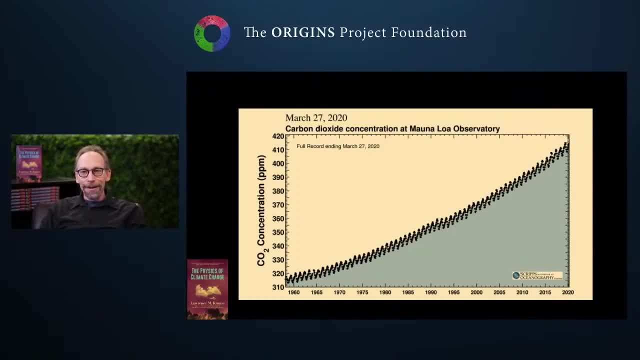 That's the day last year that I finished writing the chapter on this particular subject, And so March 27 was the snapshot. You can go to the Scripps Institution of Oceanography website and see every single day what the carbon dioxide concentration is. It's now, as you can see. it's increased from about 315, 314 parts per million, all the way up to in excess of 410 parts per million. 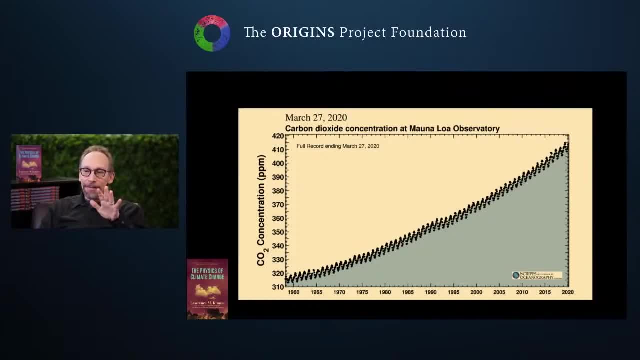 At a peak of around 417 parts per million In the last 60 years. it's increased by 30% alone In 60 years. Now again, is that significant? Well, fortunately, it turns out, while there wasn't a direct measurement of carbon dioxide in the atmosphere before that, we can get an indirect measurement. 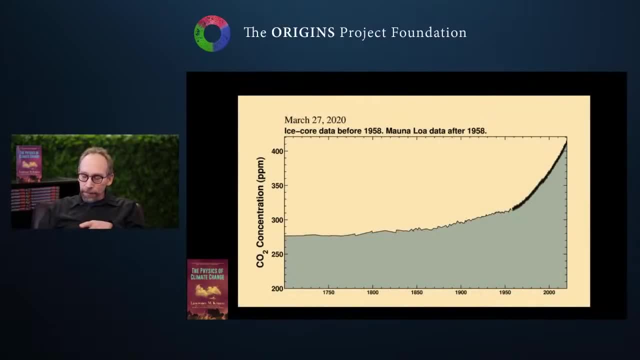 And that comes from looking at ice cores. In Antarctica in particular, Ice cores are kind of like tree rings, Because every year snow falls, gets compacted And you can see the seasonal variations And you can literally count years, And for deep cores we now can go almost a million years back. 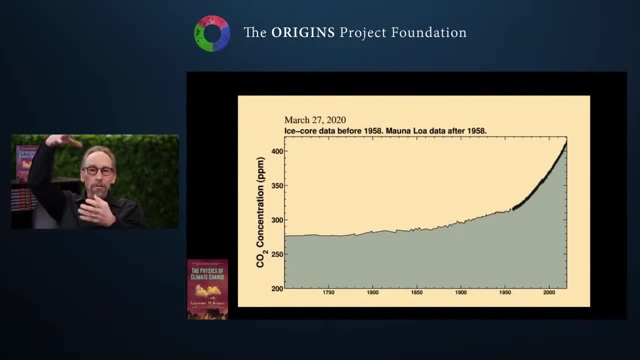 And when snow falls and eventually becomes ice, it captures little bubbles of air in the ice And those little bubbles of course contain carbon dioxide. So in those ice cores at each level you can measure the carbon dioxide and get a record of carbon dioxide over geological times. 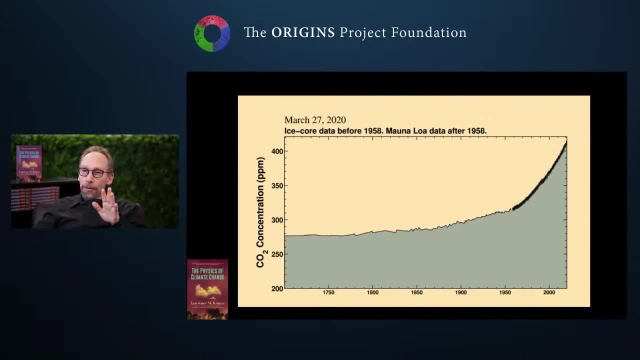 Not just over the last 60 years, And you can see this incorporates a combination of the ice core data before 1958 and the monolodic data after 1958. They match, which is a good sign. It means that things are in agreement. 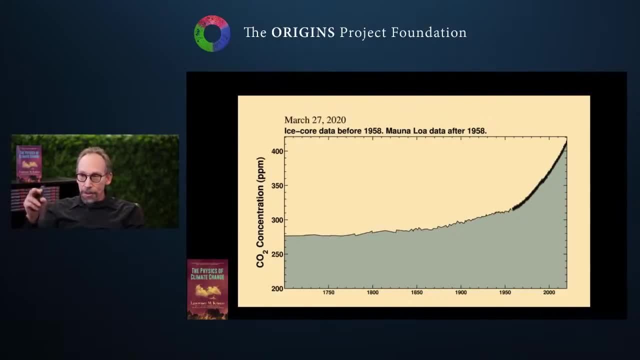 And you can see that at no period, certainly in the industrial age since 1750, has the carbon dioxide concentration approached anything near what it was already by 1960. And clearly not at the current time. Let's go further back, Because the ice core data allows us to do that. 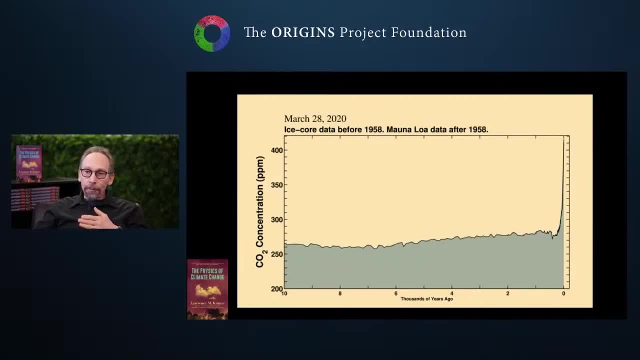 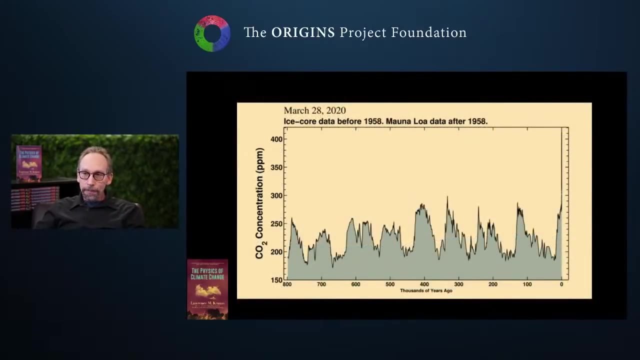 We can go back not just a few hundred years but in this case, 10,000 years. You can see local variations But once again, the current time is unique in that 10,000 year history. And finally, if we go back, in this case with these ice cores, down about 800,000 years back, you can see that there are variations. 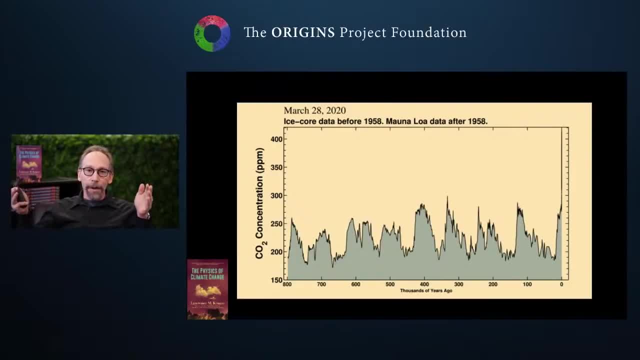 These variations are geological variations corresponding to the years where there was glaciation And when the glaciers went back, And so you can see the Earth went through periodic changes, And that's due to variations in the Earth's orbit around the sun. in fact, 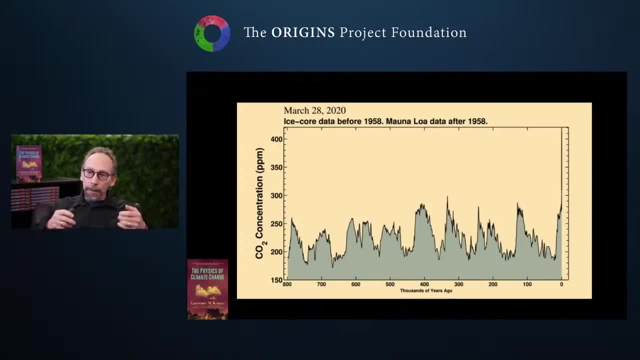 They took place not on century time frames but in fact on tens or 20,000 year time frames, as you can see. But again, during this entire period, during which there was glaciation and no glaciation, the carbon dioxide in the concentration of the atmosphere never really went above close to 300 parts per million. 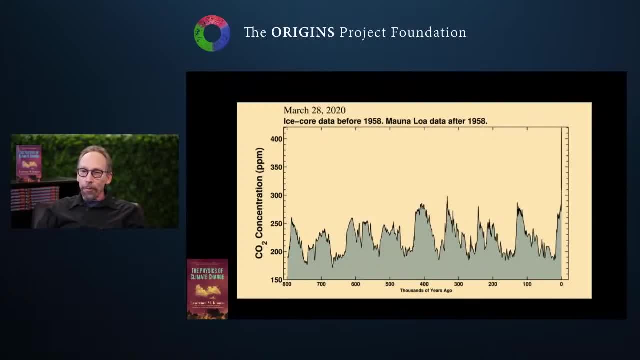 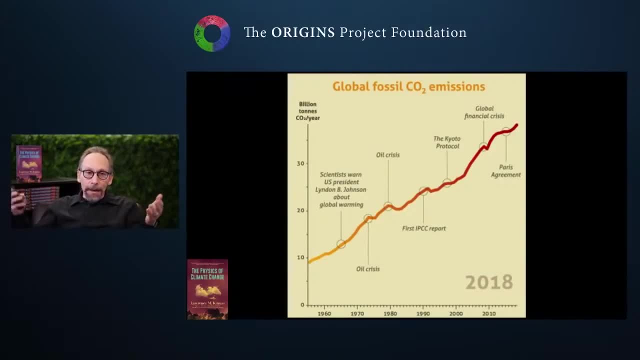 Whereas in the last 60 years it's gone up from 310 parts per million up to 417.. Now some people say, well, maybe that increases, It doesn't have anything to do with humans. And the point is there's a lot of evidence. 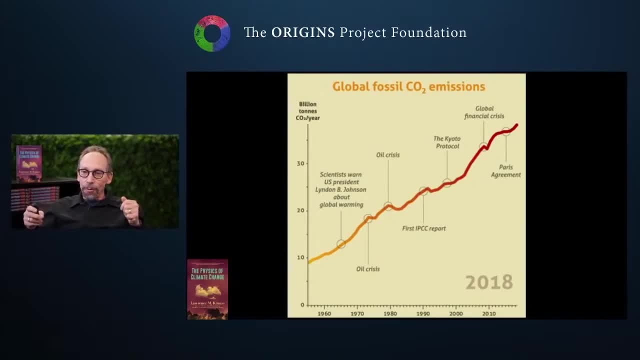 And I'll show you. And we understand that it has to do with humans. But this looks at the healing process. This looks at the healing curve And overlaid on it are certain periods in human history. You can see that the carbon dioxide growth in the atmosphere right in the oil crisis in the early 1970s, it leveled off. 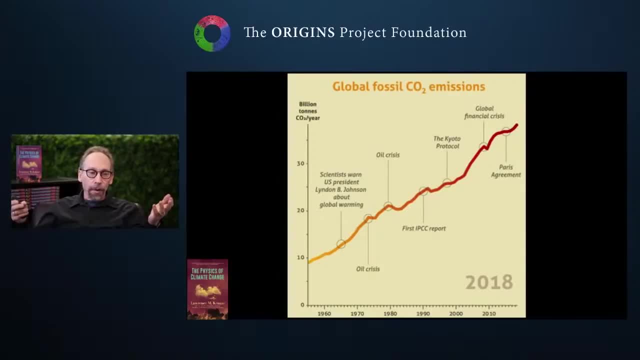 And again in 1980, decreased because of less fossil fuel usage by humans. Again, the global financial crisis in 2009, when there was less travel, when there was less transportation, caused a little dip At the time of the Paris Agreement. maybe psychologically people started to use it a little bit less. 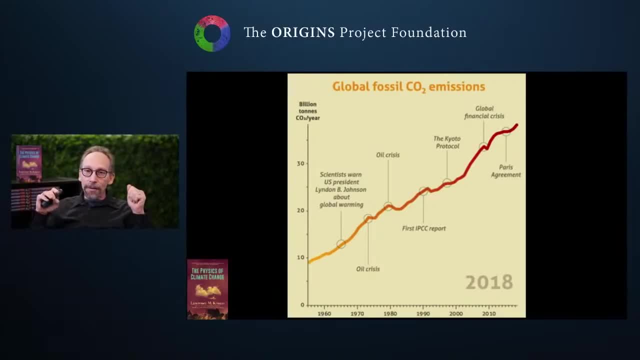 And there was a leveling off And this ended in 2018.. But you can actually see, after the pandemic there's again another little dip, but just a little dip. So human activity is clearly affecting the monotonic rise of carbon dioxide in the atmosphere. 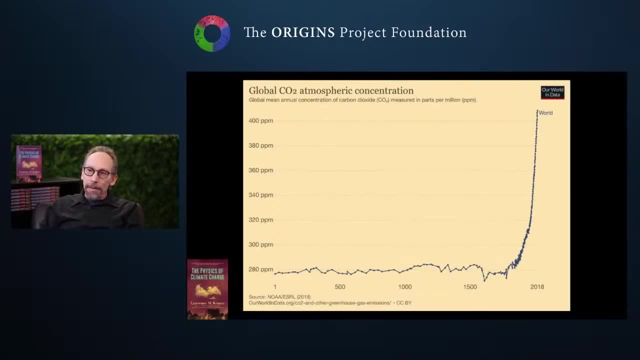 For me, this is one of the. this is the time period that I find most fascinating, From the year 1 AD to the current time, And you can see there were periods there was a little mini ice age in around 1600 or so. 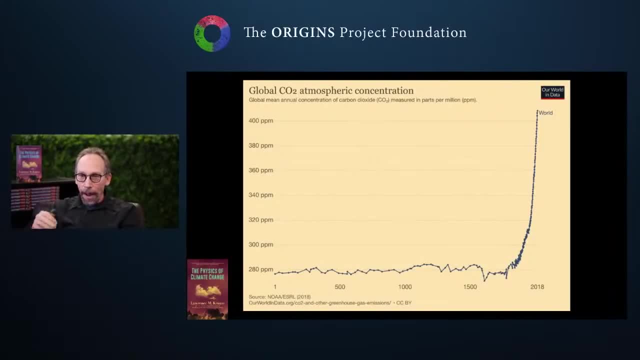 So you can see that there were variations, And those variations were natural and geological and due to various things, In some cases explosions of volcanoes, by the way- But what's happened since 1960 is unprecedented in modern human history, From, basically, 1 AD. 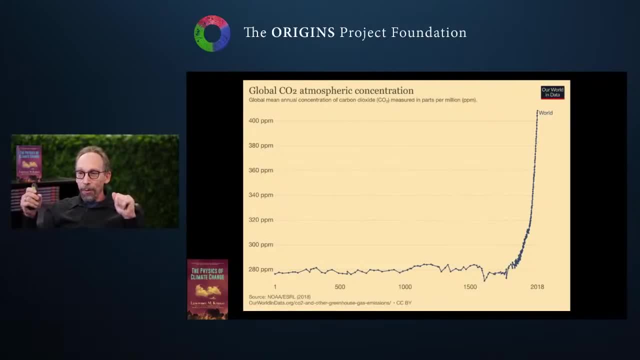 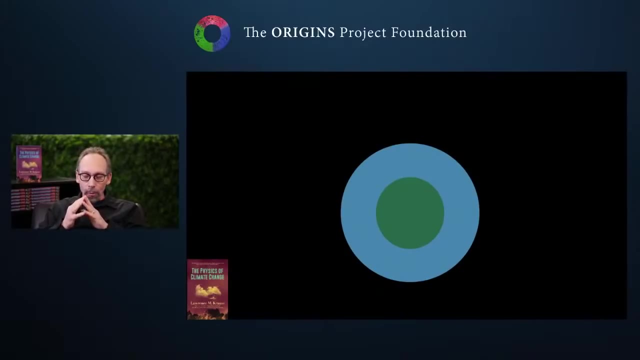 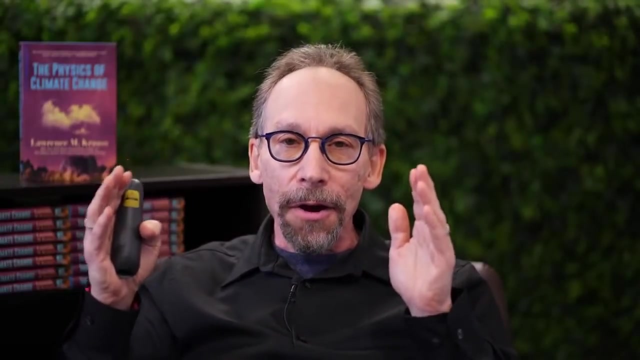 in the last 20 centuries, 21 centuries. you can see that now the world is in a place it's never been before, At least in modern human history. Okay, Now people often wonder. especially deniers ask the question: can humans really have produced enough carbon dioxide to affect the entire global feature of the earth? 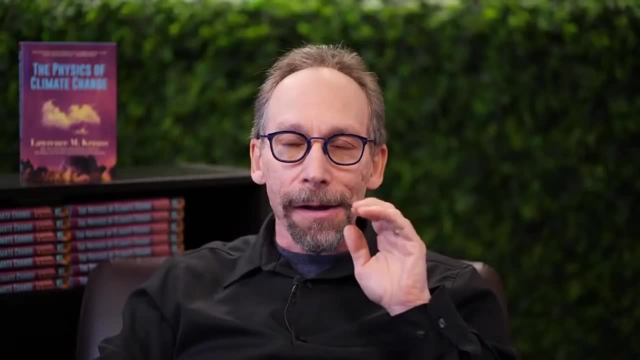 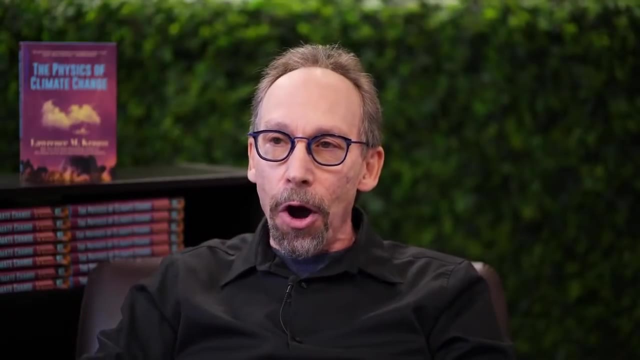 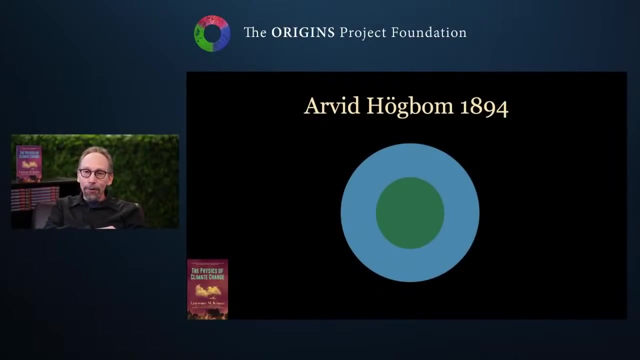 And I think the first person to make a convincing argument about that as I was researching for the book, was a Swedish geoscientist named Arvid Hagbom Who in 1894 did a kind of wonderful calculation. It's kind of back of the envelope calculation. 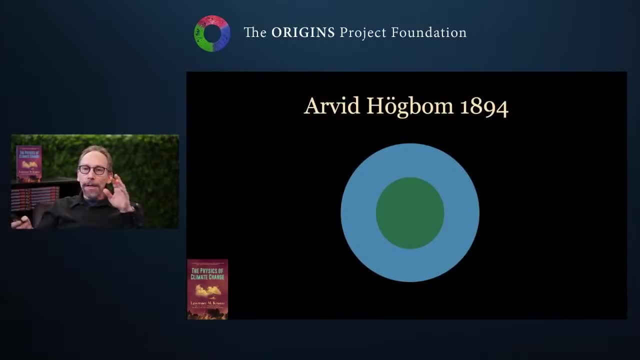 It's the kind I like as a physicist. He said: well, look, he knew roughly how much carbon dioxide was in the atmosphere. They wouldn't have made a specific measurement, But they knew it was around 300 parts per million, As I'll talk about. 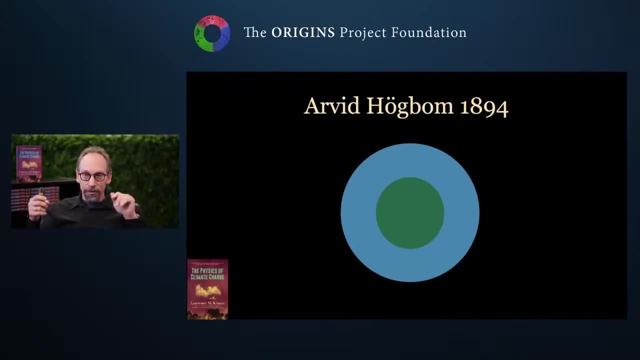 By measurements made earlier By other scientists. And Hagbom said: well, take all of that carbon dioxide in the atmosphere. What would happen if you liquefied it all? Or solidified it all? How thick a layer would it cause on the surface of the earth? 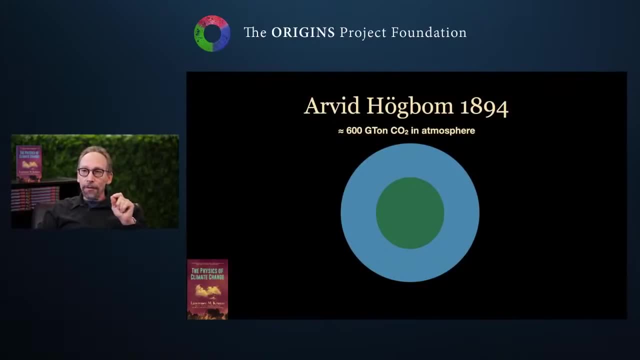 So if you, there was about 600 gigatons of carbon dioxide in the atmosphere in 1894.. 600 billion tons of carbon dioxide in the atmosphere- Actually, that's 600 billion tons of carbon in the atmosphere. Actually, that's 600 billion tons of carbon in the atmosphere. 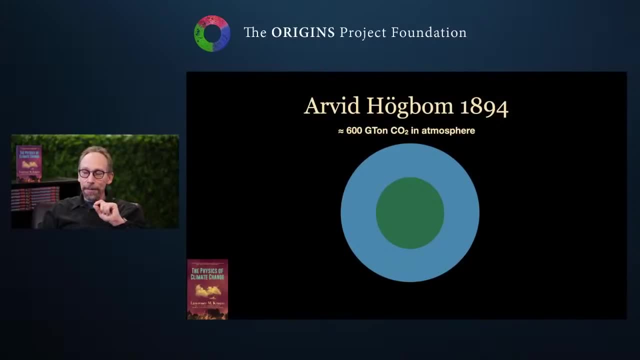 I should have pointed the other way. Not carbon dioxide, but just carbon. And if you liquefied it, he showed that in fact it would produce a layer about one millimeter thick on the earth's surface. At which point he said: clearly, life can affect the carbon abundance in the atmosphere. 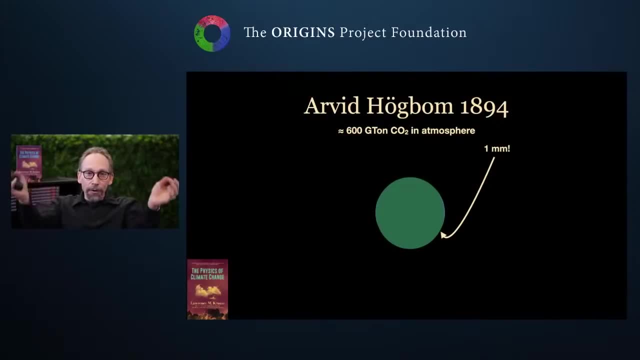 Because, if you look at the earth's surface, life is everywhere, even in the oceans, a layer thicker than one millimeter, And began to speculate, in fact, that maybe human industrial activity, after all, which is beginning to probe not just life in a millimeter. 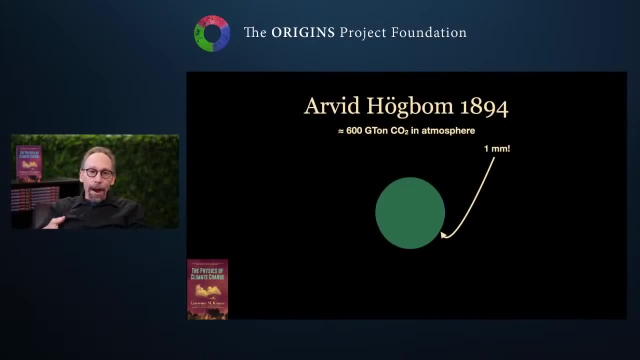 but by digging down for fossil fuels is actually extracting carbon from millions of years of living beings, can clearly affect the carbon in the atmosphere. And of course we have, as you'll see, and as you've seen already with the Keeling curve, 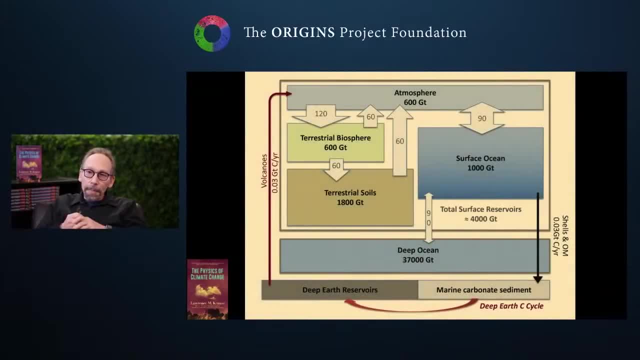 Now here is a block plot that I obtained. Here is a block plot that I obtained From a colleague at Lawrence Berkeley Lab That shows roughly the carbon exchange in the atmosphere in various reservoirs on earth. So, as I said before, by about, you know, somewhere between 1900 and 1960, there was about, let's say, 1900,. 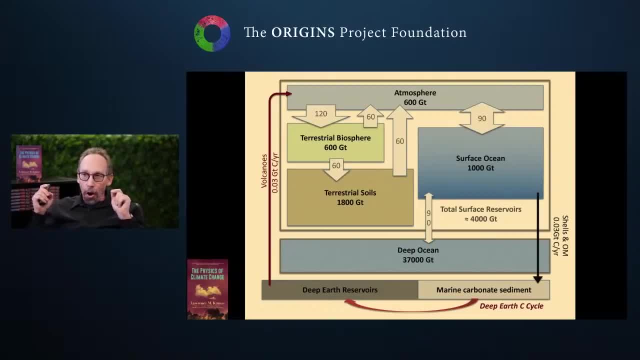 there was about 600 gigatons of carbon in the atmosphere And regularly there's an exchange with the biosphere, with plants and terrestrial soils. You can see it's about 120 gigatons Go back and forth: 60 into the biosphere and 60 into the soils. 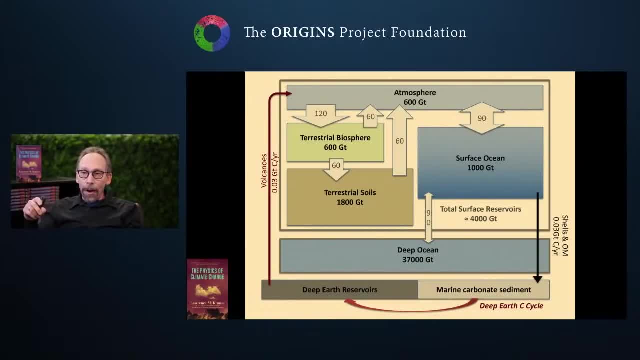 There's exchange with the surface ocean about 90 gigatons, And again the surface ocean exchanges with the deep ocean, which is a huge reservoir of carbon of 37,000 gigatons, And that happens on a regular basis. 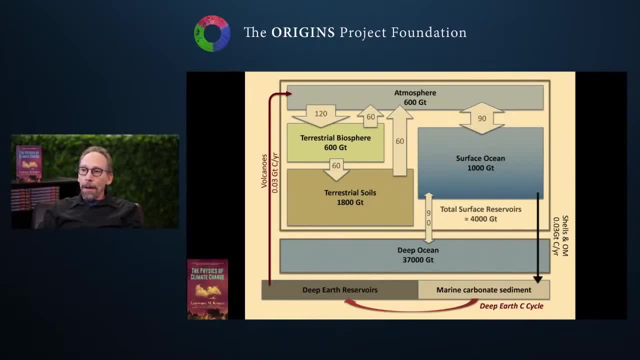 Those are exchanged yearly. On top of that, there's a geological cycle which has been around even before the existence of life, in fact, And that's Carbon in the atmosphere is dissolved in the water, It produces carbonic acid, which basically dissolves and produces calcium carbonate. 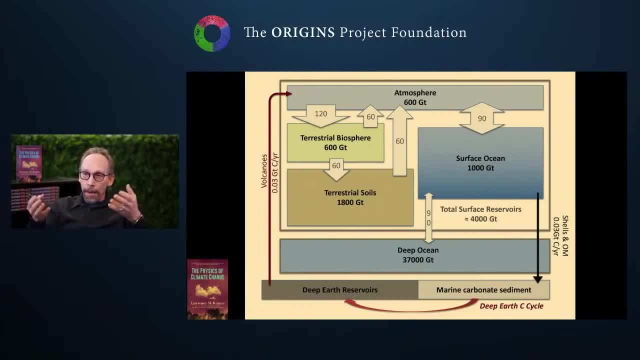 which goes down to the ocean floor, And it also produces shells and living things. That gets down in the carbonate sediment into the ocean floor. But as the global plates move and regions are subducted under the surface, that carbon gets taken into the mantle and into deep earth reservoirs. 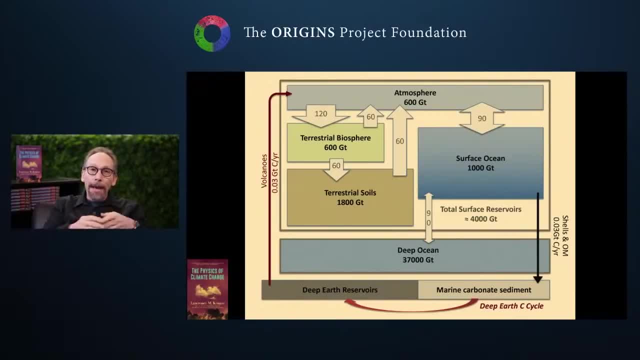 And eventually builds up and is released by volcanoes And over about a 100 million year period that cycle equilibrizes And you'll see, compared to the carbon exchange due to life, it's very small. It's .03 gigatons of carbon per year is cycled through the earth by volcanoes and sediment. 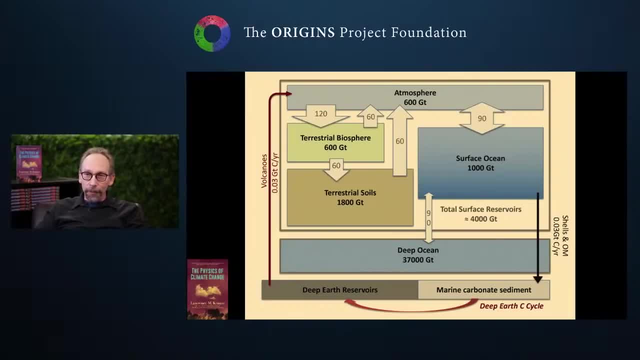 So it's really the rest of life that's producing a significant amount more. That was before Human industrial activity, But how have things changed since that time? Well, here's what we're doing On an annual basis. we And this was in 2018, but the number's basically the same now in 2021.. 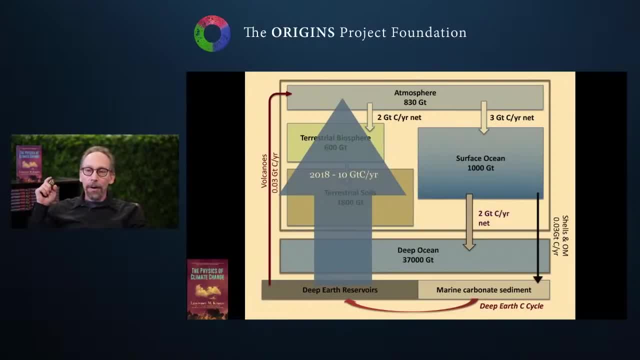 We are producing and putting into the atmosphere roughly 10 gigatons of carbon per year due to human industrial activity. Now that means that in the atmosphere now there's not 600 gigatons of carbon, but there's 830 gigatons. 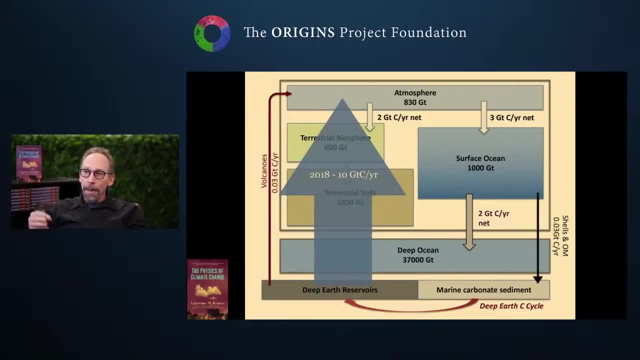 due to the increase, as you saw from that Keeling Curb. What happens to that carbon, that 10 gigatons of carbon per year we put into the atmosphere? About half of it goes back into terrestrial biosphere and to the surface ocean and eventually into the deep oceans. 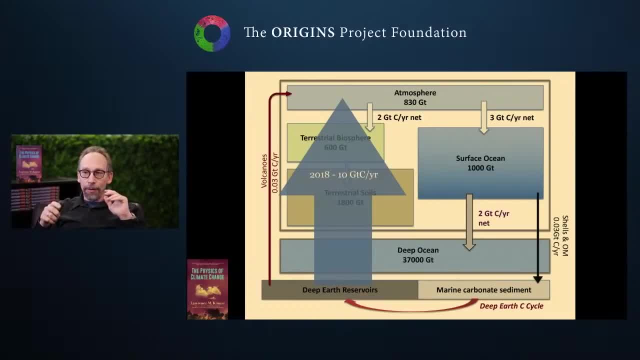 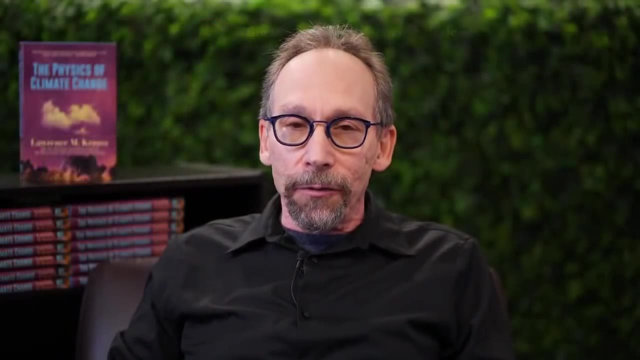 Half of it remains in the atmosphere. So about 5 gigatons per year remaining in the atmosphere, every year increasing the carbon into the atmosphere. Now let's talk about the effect of carbon emissions. Now, this is the famous greenhouse effect. 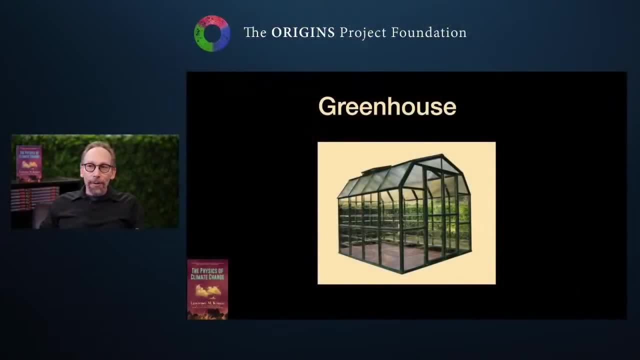 which is poorly named, because the Earth is not like a greenhouse. It's a poor usage of the word when it was first done, Because a greenhouse, of course, and a car. if you're in a greenhouse, you can be much warmer. 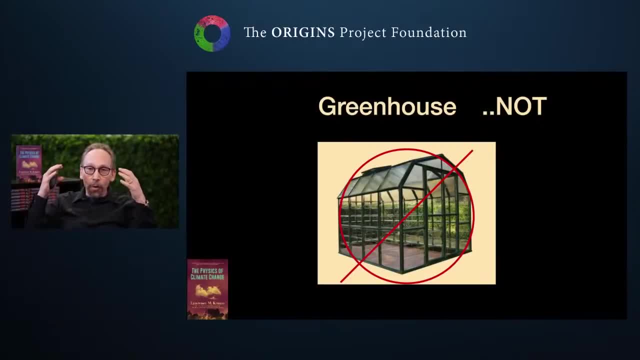 because of course the sunlight comes in and the greenhouse holds in that heat. There's a few reasons the greenhouse holds in that heat. Part of the radiation, the heat radiation that's in the greenhouse, can't escape through the glass. 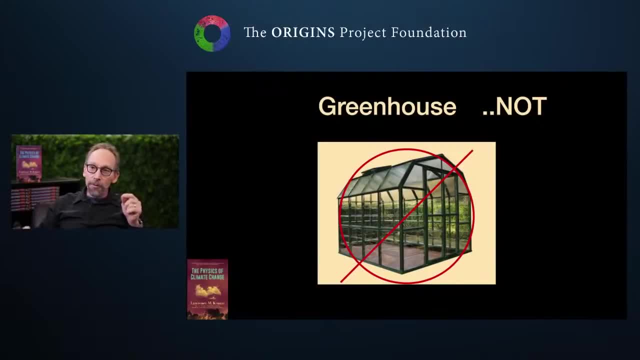 but equally important or perhaps more important. in a greenhouse there's a barrier, there's glass that stops heat from escaping. The Earth doesn't have such a barrier And people often, when they try to be skeptical of the greenhouse effect, recognize that difference. 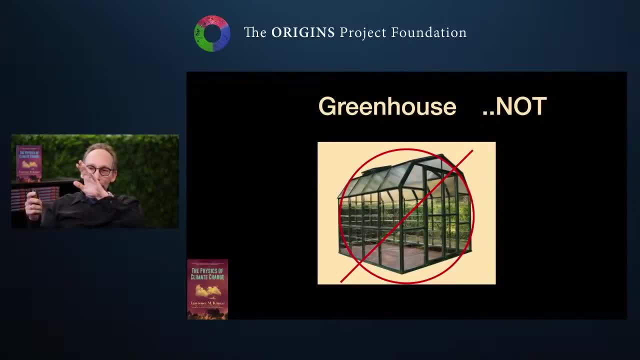 But the real greenhouse effect in the Earth has nothing to do with that glass barrier but rather to the other effect, the fact that sunlight coming in is not as easily radiated going out. And I want to go through those numbers Right now for you. 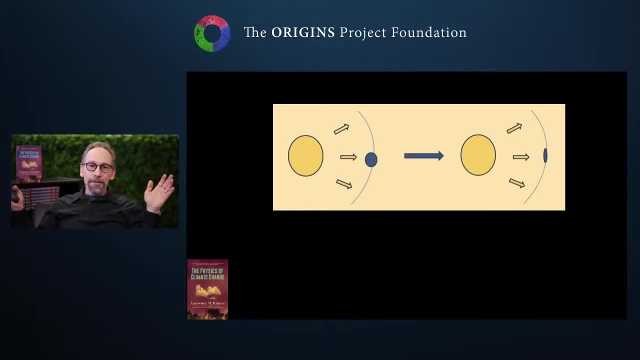 So the sun provides the heat that keeps the Earth going, And for some people it may be a surprise to learn that the Earth is a sphere, If it were a disk directly parallel to or perpendicular to the sun's rays. the sun is depositing about 1,314 watts. 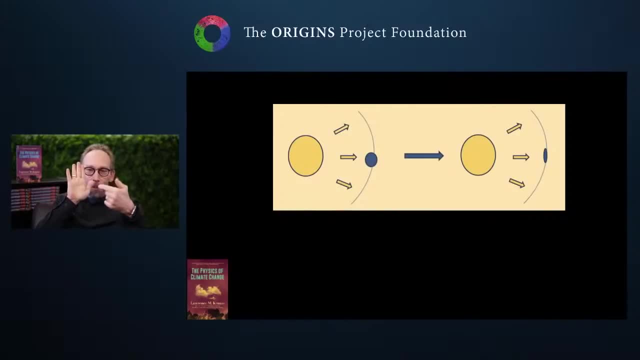 per every meter squared of surface directly perpendicular to the sun's rays. But the Earth is a sphere, And a sphere has four times the area of a disk, So the average radiation impacting on the Earth from the sun is one quarter times, not 1,314, 1,361.. 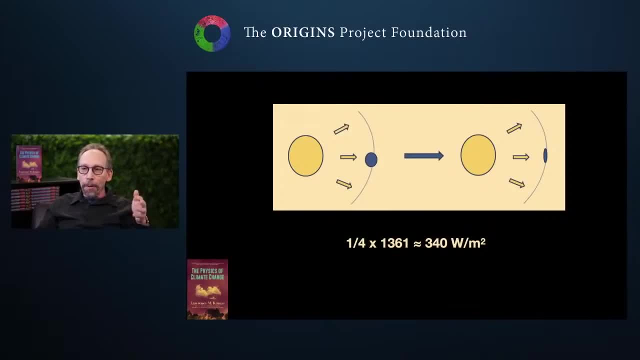 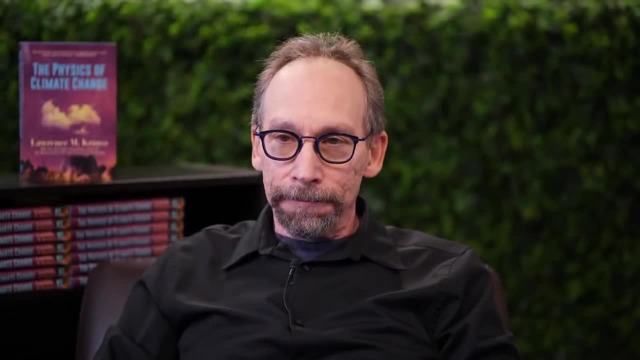 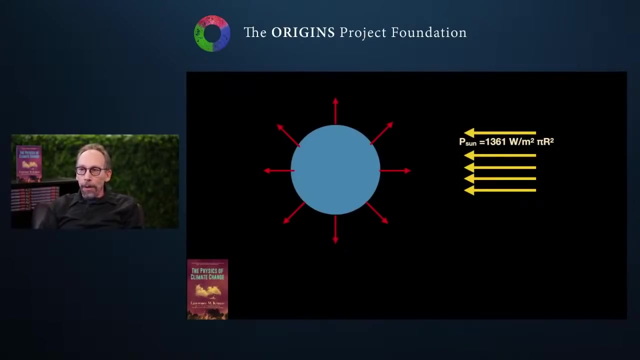 So one quarter times 1,361 is about 340 watts per meter squared is the average energy of the sun hitting the Earth each day. Now what happens? Well, we've got 1,361 watts per meter squared hitting each meter squared of the Earth. 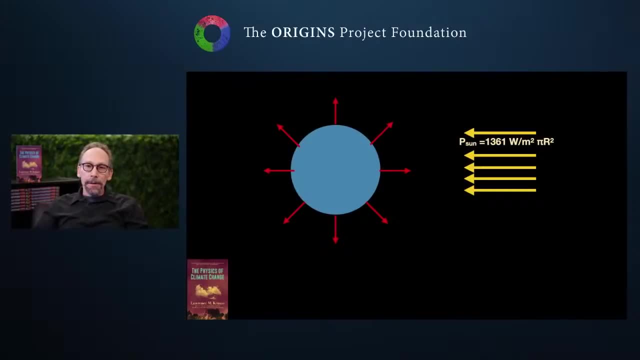 And then, of course, to understand the total heat absorbed by the Earth from the sun, or at least impinging upon the Earth from the sun, you multiply it by the surface area of the Earth, In this case, sorry, the surface area of an effective disk. 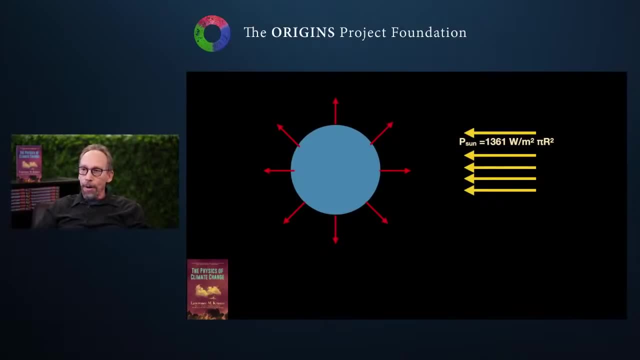 facing the sun. That surface area is pi r squared And you get the total energy impinging on the Earth. Now some of it is reflected right away. Some fraction A is reflected right away, So the amount of energy power. 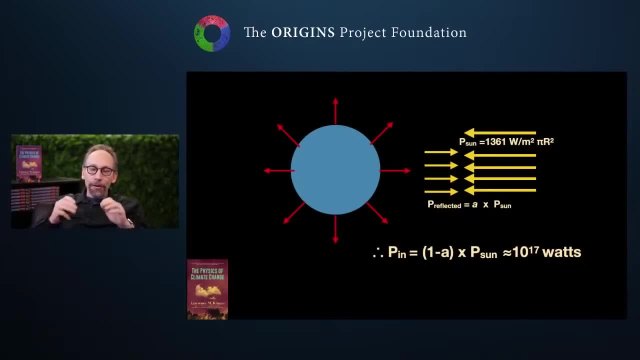 coming into the Earth is 1 minus A. the fraction that isn't reflected, times the total power coming from the sun And when you work it out over the Earth you get about 10 to the 17 watts, Or about about 100,000. 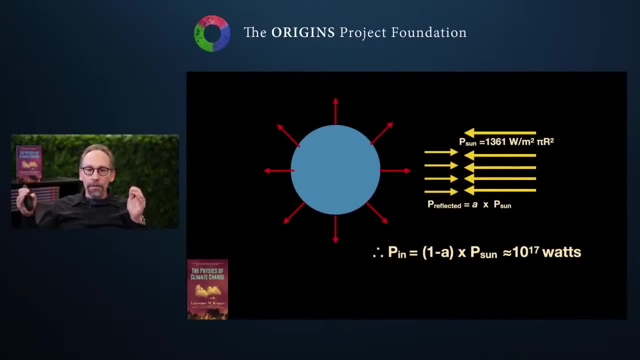 gig terawatts, About 100,000 terawatts of power. Now the reason I talk about terawatts is rather interesting to me. Humanity, all of humanity, uses about 20 terawatts of power, And that means that the sun each day 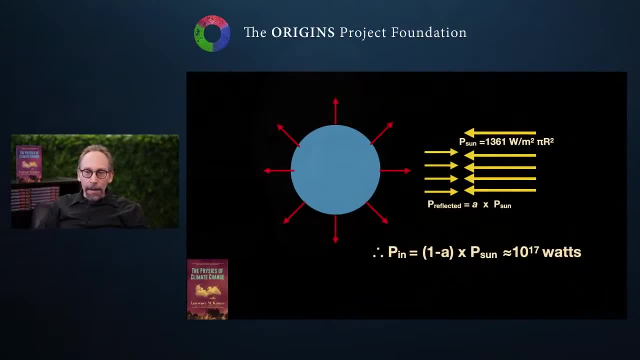 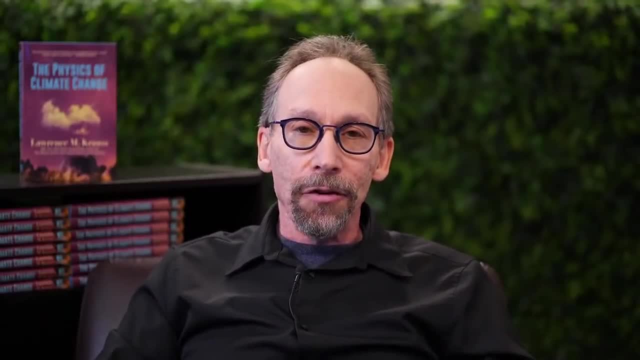 is is sending roughly 10,000 times as much energy as all of humanity uses in solar radiation, One of the reasons that many of us think the sun is a good place to look for energy: 10,000 times as much energy is impinging on the Earth's surface. 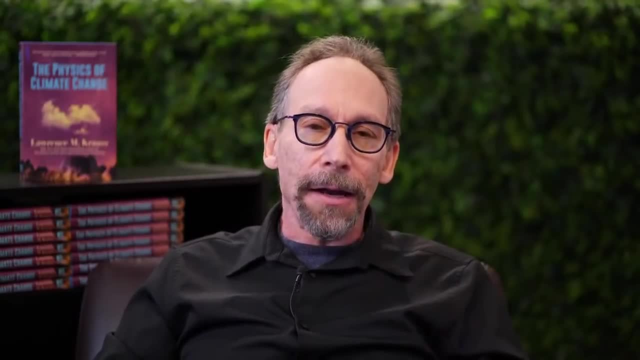 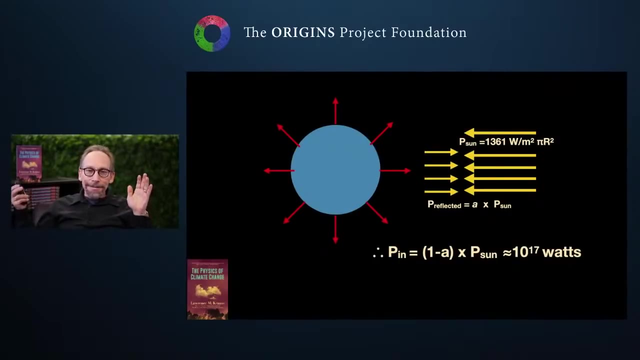 each day as compared to that total usage by human industrial activity. In any case, that's the power in. Now, the central premise of climate and physics is not very difficult. It is that power in equals power out if nothing's going to change. 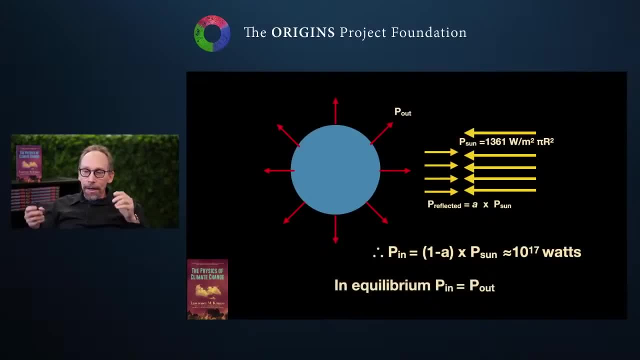 So how much power is going out of the Earth In equilibrium? if the temperature's not going to change, P in has to equal P out. So if the Earth is radiating as much out as is coming in, the temperature will remain the same. 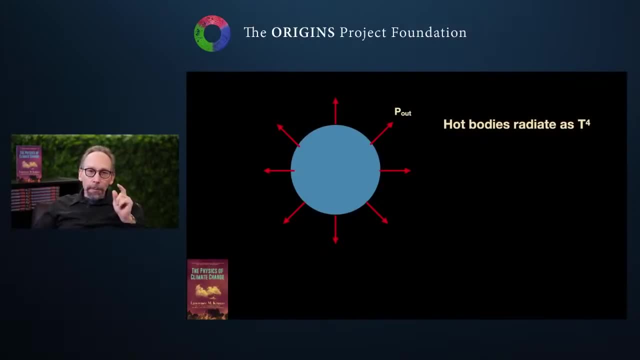 Okay, Now the other piece of physics that you need to know is that a hot body radiates as the fourth power of the temperature. So we can just say: okay, the Earth is radiating with a surface area of 4 pi r squared. 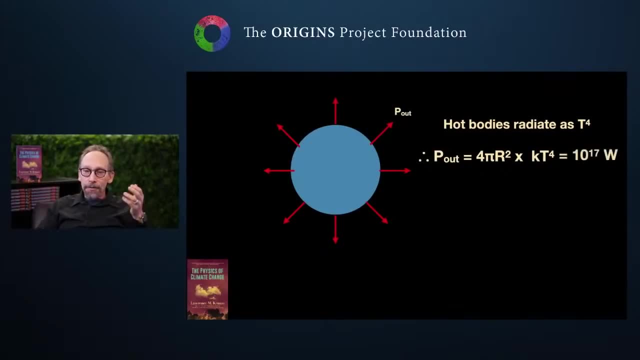 times, some constant times, T to the fourth, and that, if the temperature isn't going to change, has to equal 10 to the 17th watts. This calculation was first done by Joseph Fourier, a very famous mathematician and physicist, I think in 1824.. 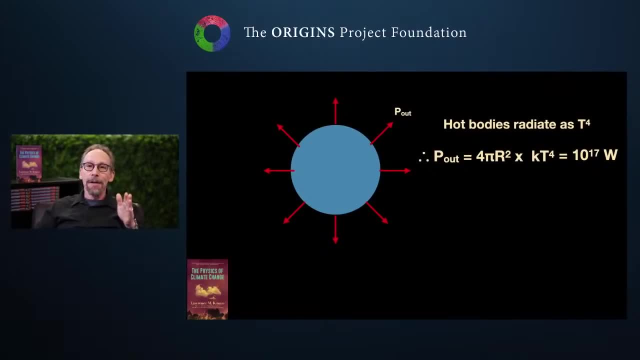 And he did that calculation and said and solved for T. He said what should be the temperature of the Earth? And when he did he found out the temperature of the Earth should be 18 degrees below zero Celsius. Frigid Much colder than the polar vortex was. 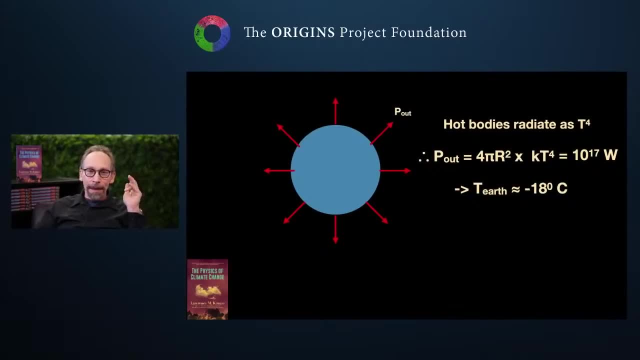 for most of the United States and some of Canada, And it was 1824.. He said: if this is true, the Earth should be frozen solid. The temperature of the Earth should be much lower than it actually is The actual temperature of the Earth. 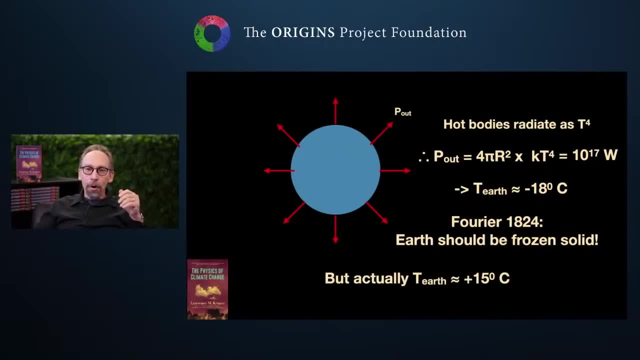 is 15 degrees Celsius, Okay, 33 degrees warmer Celsius than this simple calculation would predict. And so the answer is: there had to be something else keeping the Earth warm. And he began to recognize, and in fact he was the first one to suggest. 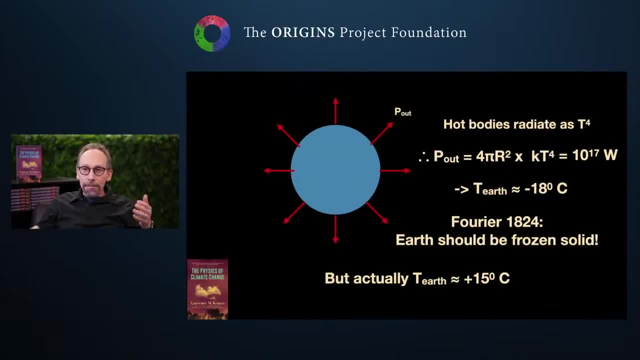 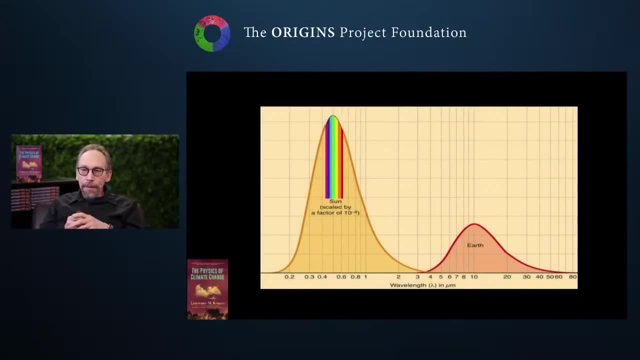 what might now be called the greenhouse effect, and did some experiments saying maybe there's an insulating layer that's holding the heat in. And we can understand this by looking at radiation coming in. The sun's radiation comes at a given set of frequencies. 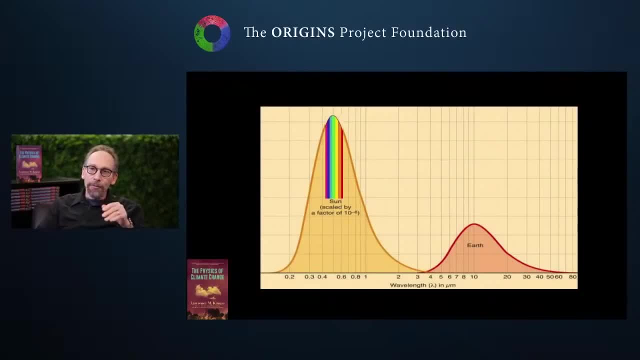 in micrometers, less than one micrometer. If you look at the visible light from the sun, it's, in the range shown there, much less than a micrometer, And in that wavelength band the atmosphere is transparent. But if you look at what would be, 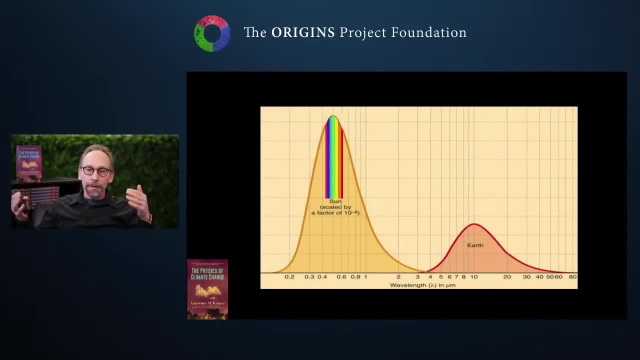 the radiation emitted by a surface body at 15 degrees Celsius. you see the curve that I show you. for the Earth Generally, it'll be emitting in the band that peaks around 10 micrometers, or microns as we call it. A very different radiation band And the atmosphere is transparent in the smaller radiation band but isn't transparent in the larger wavelength band, That's in the infrared. The smaller band is visible light, The larger wavelength band is the infrared And the atmosphere is not transparent there. 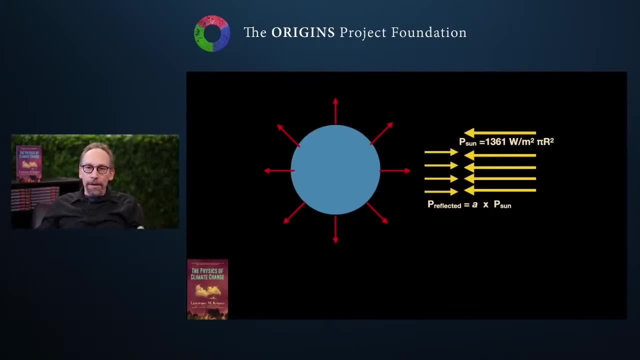 So let's go through and do a simple calculation, a very simple model. This is what I showed you before. Some fraction of the sunlight is reflected in the surface of the Earth, But now we have this layer of atmosphere that's doing some absorbing. 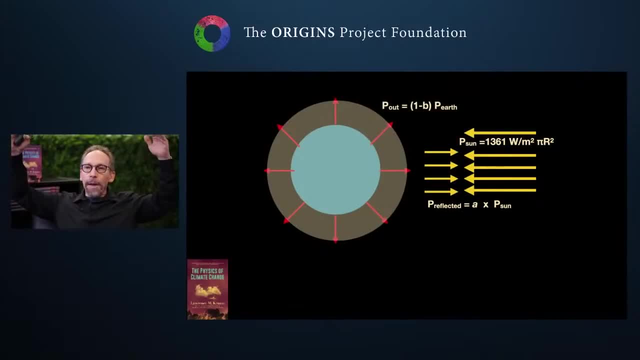 And so say that now the radiation that gets out into space is not the radiation emitted from the surface of the Earth, but rather some smaller fraction, because some fraction of it is absorbed. So the power going out is 1 minus b times the radiation emitted from the surface of the Earth. 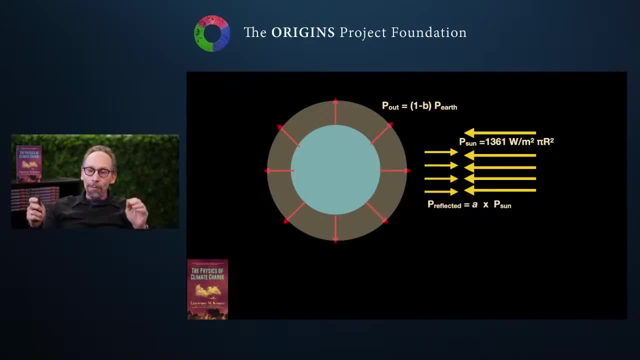 where 1 minus b is now a number less than 1.. And that means that the power radiated by the Earth is the power that gets into space divided by 1 minus b. But since 1 minus b is a number less than 1,, 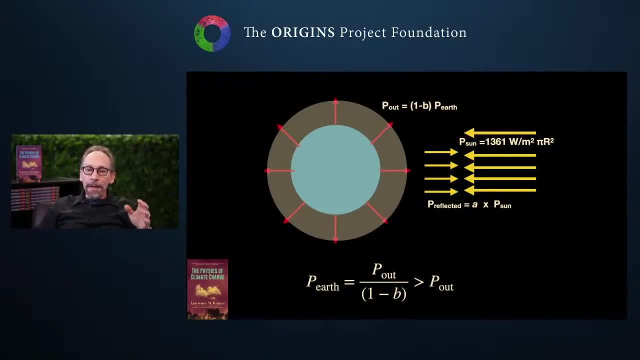 that's much bigger than the power out, So it means the Earth can radiate much more than you in order to get a power out. that's equal to 10 to the 17th watts. the Earth is actually radiating at its surface. 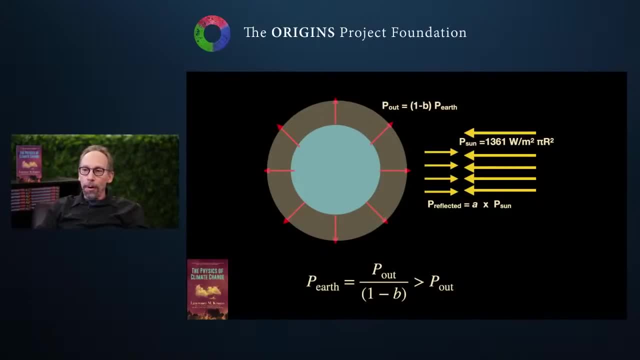 much more energy, but a lot of it's being absorbed and therefore you get a temperature much, much greater than minus 18 degrees Celsius. And this is a very simplified model Because in fact it treats the atmosphere as one bulk medium. 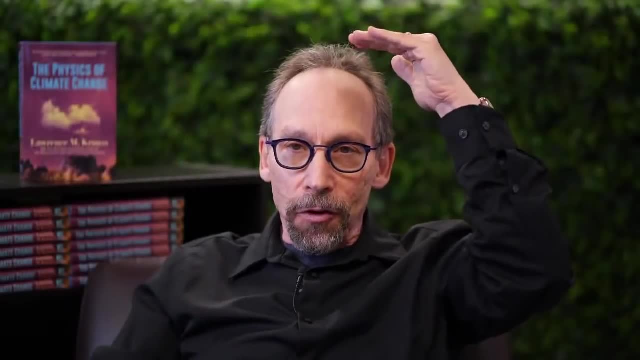 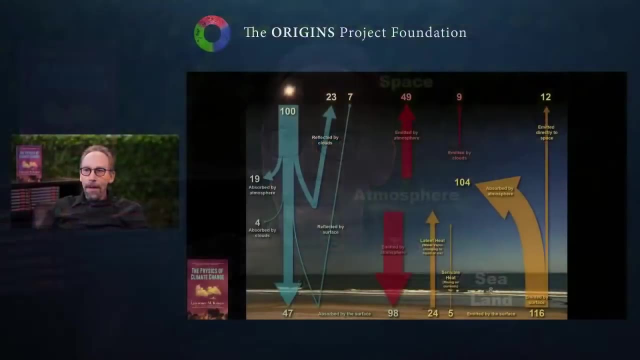 but, as I'll talk to you about, it's vitally important that the atmosphere is colder at the top and warmer at the bottom, as you'll see when we try and actually make some more realistic predictions. Here is a picture actually provided by the US government. 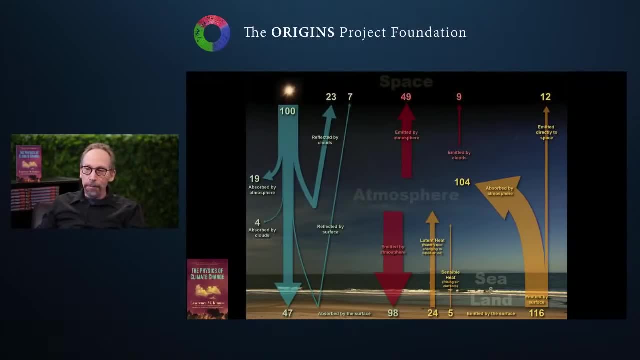 NOAA, the National Geographic and Atmospheric Administration, that actually shows the radiation coming in and what's happening. So 100,, if you wish, is the number coming in, normalized to be 100, from the Sun. Some of it's absorbed by the atmosphere right off. 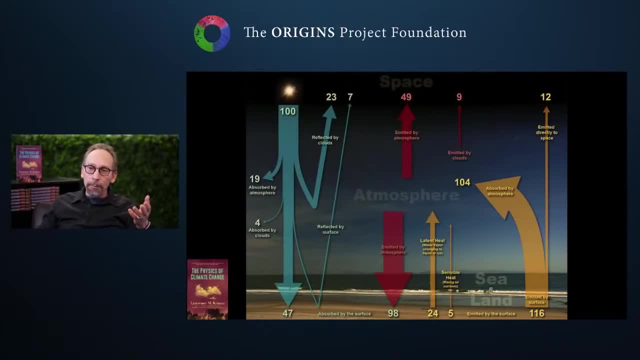 some of it's reflected. 23% of it is reflected, 19% absorbed by the atmosphere, some more absorbed by clouds. about 47% of that radiation makes it down to the Earth. Now the atmosphere ends up emitting energy into space. 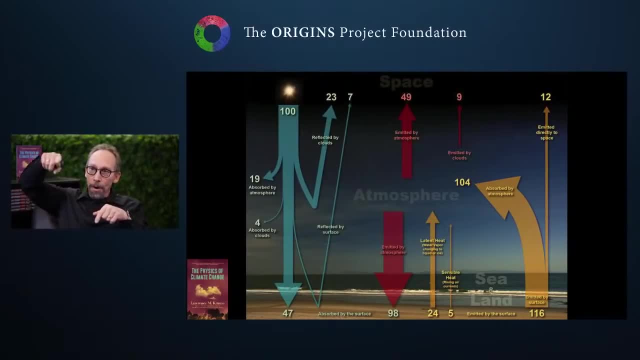 but if the atmosphere is emitting a certain temperature, it's emitting in all directions. so 49% of what was originally incumbent is emitted into space directly, but then another 49% must be sent down to Earth, But in fact the Earth. 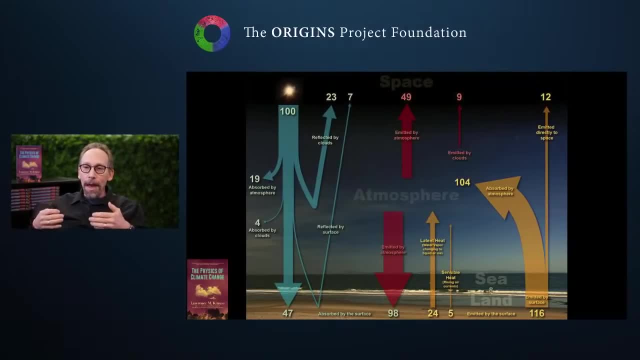 isn't just radiating. it's exchanging heat with the atmosphere by other means, by convection and by water vapor, and so the Earth is actually dumping a lot more radiation in the atmosphere. In fact, the Earth is actually dumping about 104% of what the 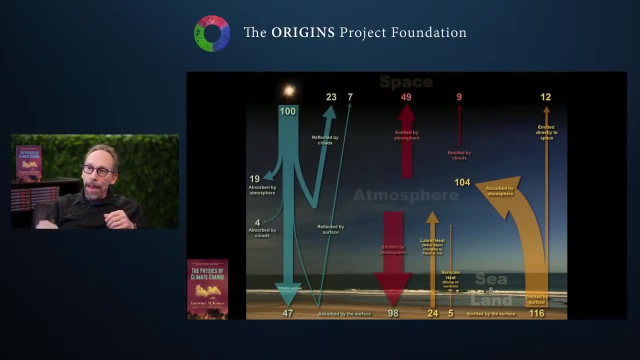 original solar radiation coming in into the atmosphere and only 12% of that is getting directly into space, coming from the surface of the Earth. Most of the radiation being emitted into space- and this is the key point- most of the radiation being emitted. 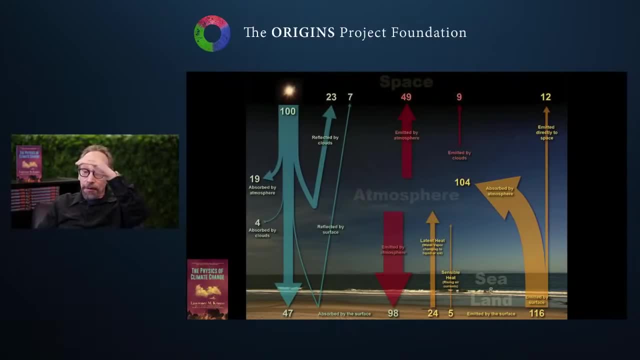 into space is coming from the top of the atmosphere, But the atmosphere is actually due to that heat exchange from the Earth to keep things in equilibrium, is actually radiating down to the Earth an amount equal to almost the entire incident solar radiation- about 98% of 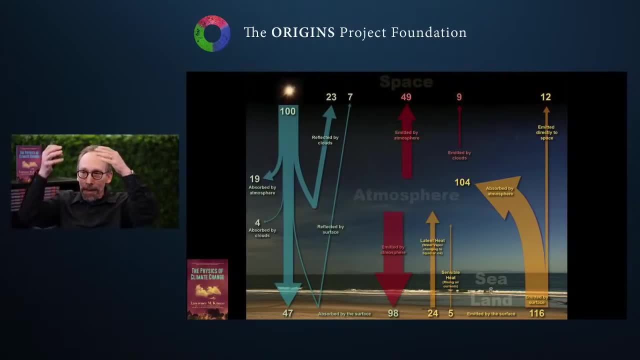 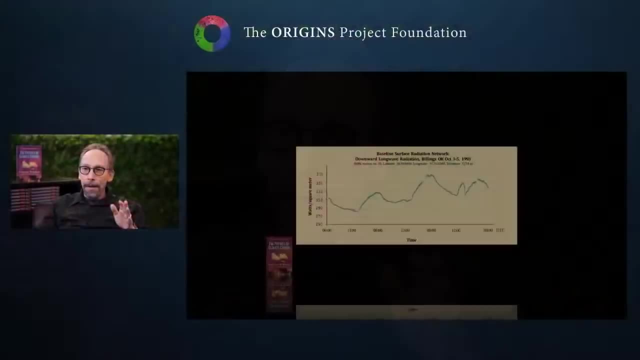 what was the value of the initial? solar radiation is coming and being emitted by the atmosphere down to the Earth And we can make these predictions. but these are not just predictions. we can make measurements. Here is some data that I got from a network. 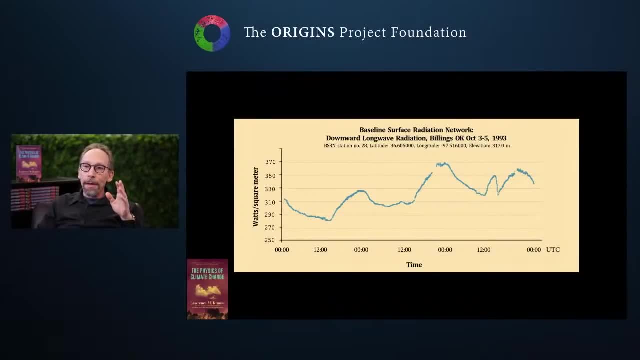 in Billings, Oklahoma, that looked on a given day, October 3rd to 5th 1993, it looked at the long wavelength, the infrared radiation coming down from the atmosphere. There was a detector, so it's looking at infrared radiation, not the radiation. 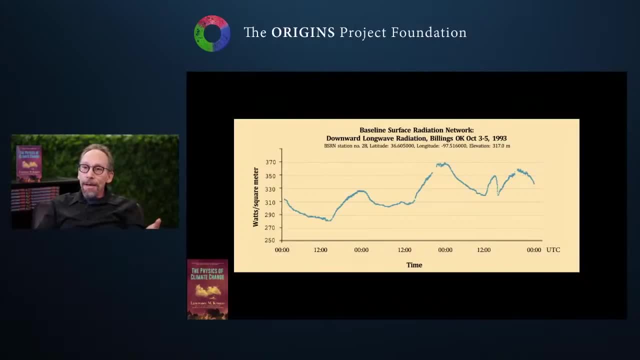 emitted by the sun, but the radiation emitted by the atmosphere and you can see this is a mid-level range, so it's about the remember. the average radiation coming into the Earth, giving the curvature to the Earth, is about 340 watts per square meter and you 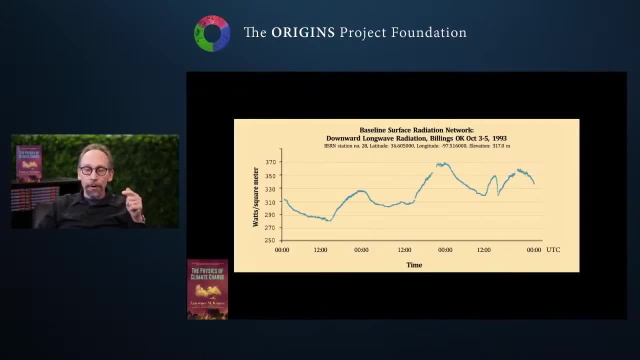 can see that the radiation coming down from the atmosphere, the long wavelength radiation, is precisely almost the same value, about 340 watts per square centimeter. So this picture holds together. But even more than that, it holds together for other reasons, because we 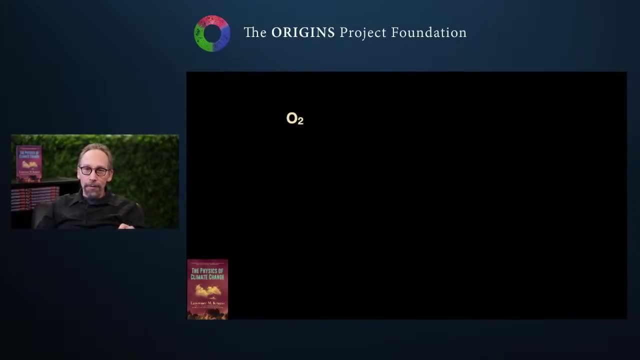 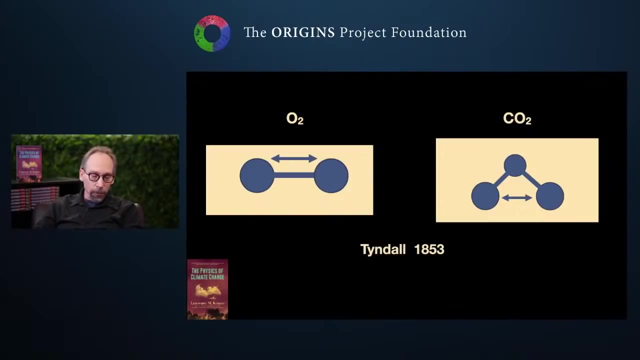 begin to understand the absorption by carbon dioxide in the atmosphere. And the first. the physics of this is actually quite interesting. Now, the first person to really begin, the real father of climate change in some sense is Tyndall, I think, a Scottish, I think he's Scottish. 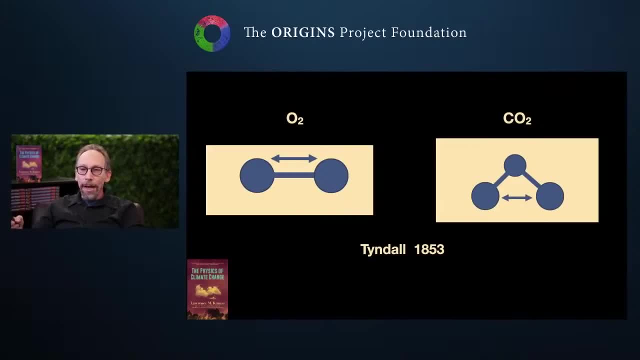 or Irish, I can't remember scientist who in 1853 really began to do the first studies to measure the absorption of infrared radiation, the so-called dark radiation. back then infrared radiation by carbon dioxide, Built detectors to try and measure that absorption. 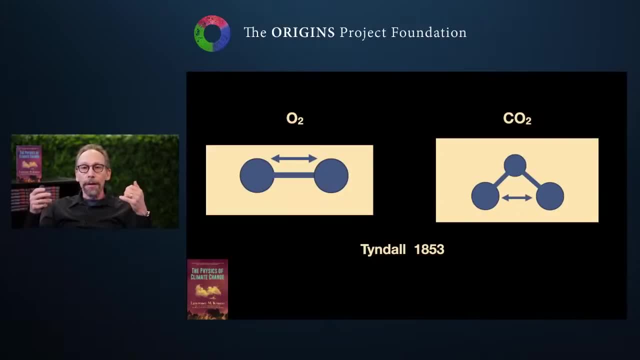 and began to suggest that carbon dioxide was what we would now call a greenhouse gas, which absorbs infrared radiation and helps lead to that effect I talked about earlier. But the real father of the greenhouse effect is a Swedish chemist called Svante Arrhenius. 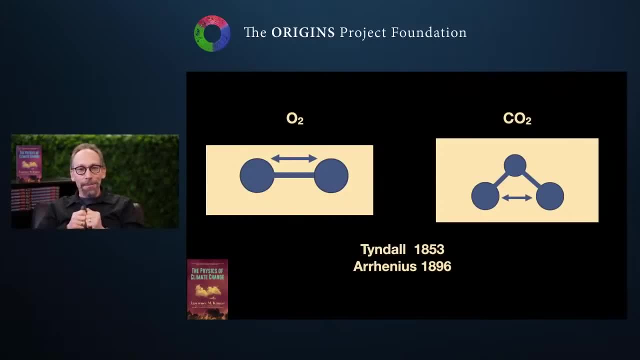 who was an interesting guy actually, and it was fascinating for me to learn about him a little bit more. He was well. he seemed to have trouble with others throughout most of his life. His PhD thesis basically got a D. He barely passed. He then complained. 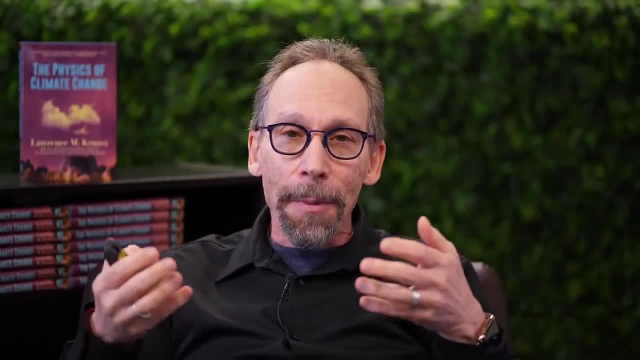 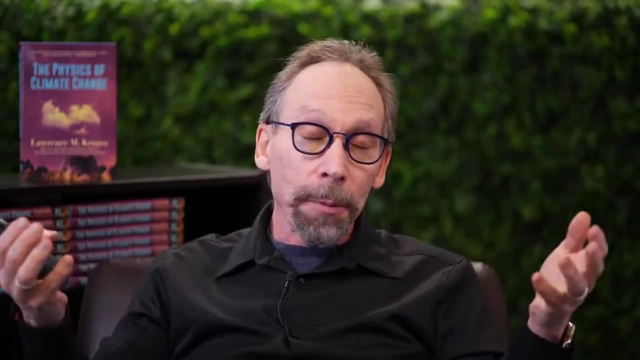 and protested and got raised to a C. Eventually he somehow managed to be able to get on the faculty in chemistry in Uppsala, but was not particularly liked by his colleagues, who barely voted him on Somehow in spite of that. 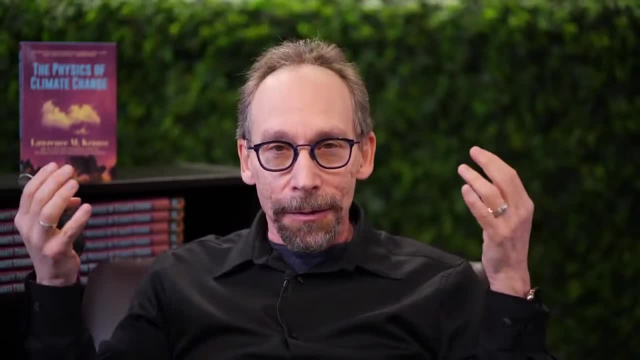 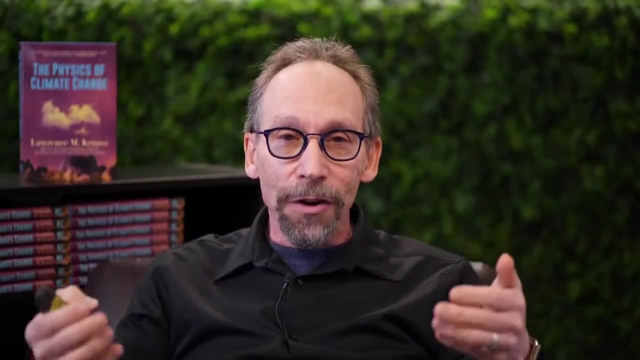 he rose to the level of rector of the university, the head of the university, which again there was complaints when he became head of the university, but he did Eventually getting on to the Royal Swedish Academy of Sciences, squeaking in that election. 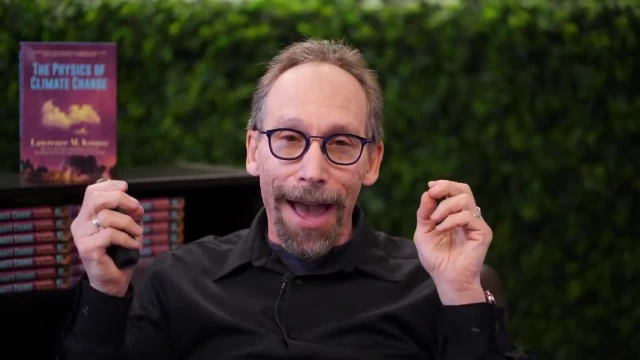 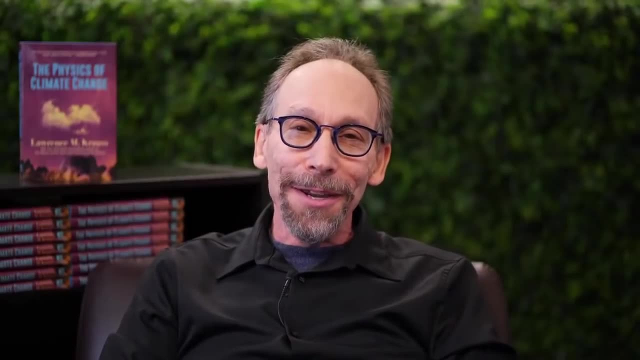 where he was elected to the Royal Swedish Academy of Sciences, which is the academy that gives out the Nobel Prize, and, interestingly, three years later he was the first Swede to win the Nobel Prize In chemistry in that case, and you might think that was a little bit of nepotism. 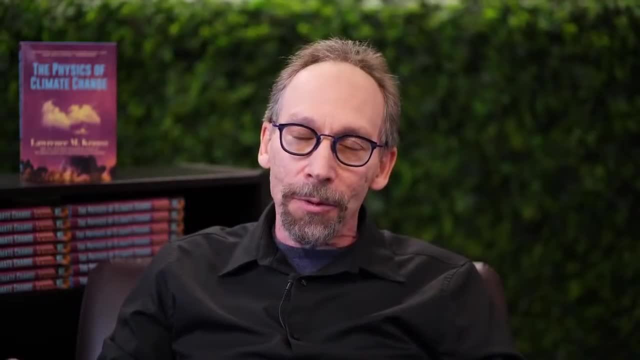 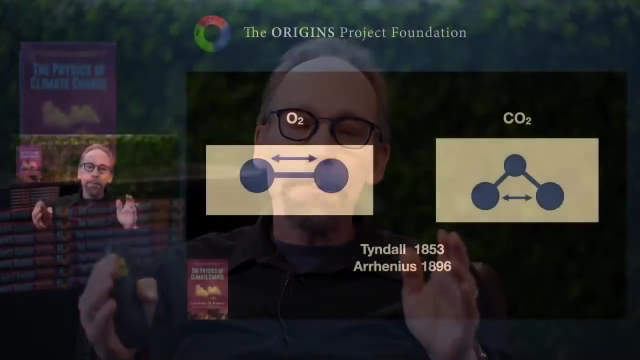 and maybe it was, but happily it turns out. Arrhenius' contribution to chemistry were incredibly important, so he certainly deserved it. But Arrhenius in 1896 released a very important paper where he basically laid the foundation of what we. 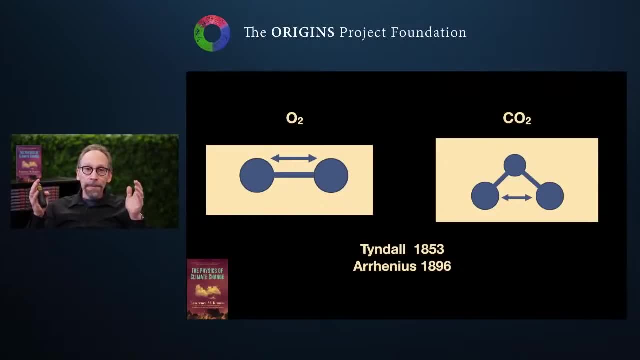 now call the greenhouse effect, argued that a doubling of carbon dioxide in the atmosphere would change temperature of the Earth. He argued at the time, given the data that he had- and I showed the data in the book and talk a little bit about that- would change. 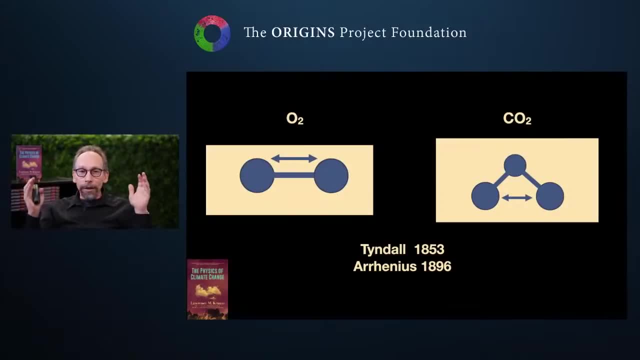 the temperature of the Earth by five or six degrees, which he thought was a wonderful thing. Living in Sweden, he loved the idea of the Earth getting warmer, And so he began to speak publicly about this, and he actually used Arvid Hagbom's 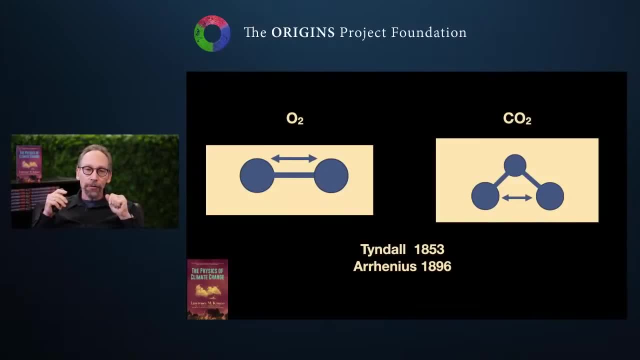 papers and translated them into English for the first time for other people. But Arrhenius' work didn't have the effect it might have because of another Swede, Knud Engström, who I thought he was well one of the. 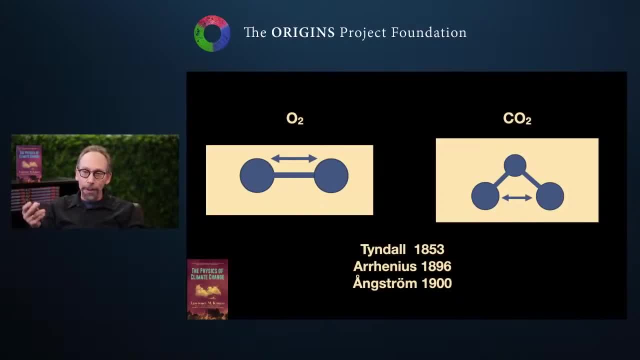 a word for a unit of length in physics is the Engström, and I thought he was the Engström behind that, but that was actually his father. But Knud Engström, for a number of reasons, argued that Arrhenius was completely wrong in his arguments. 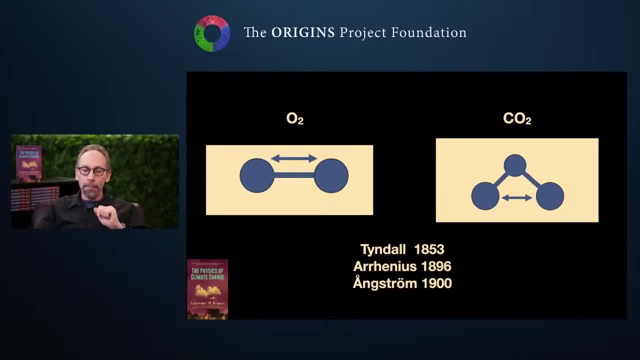 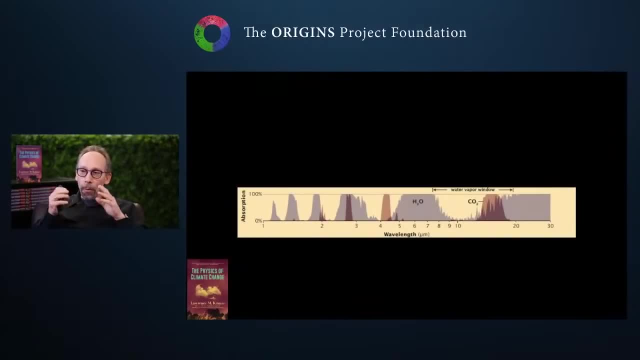 about what carbon dioxide could do, And I talk about some of these things at length in the book One I want to talk about here. This shows absorption by water and carbon dioxide in the atmosphere. Water is a greenhouse gas And Knud Engström argued: look. 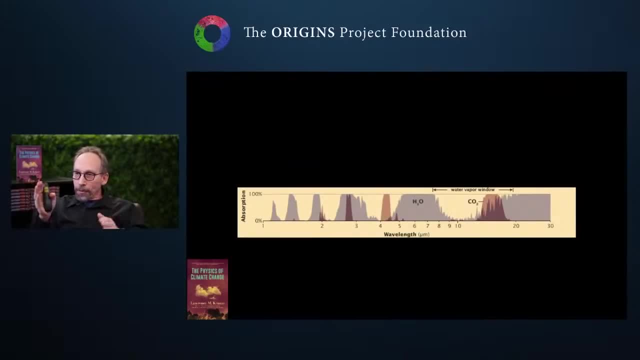 carbon dioxide absorbs. if you look at the range between 10 and 20 microns, there, carbon dioxide absorbs in a range that's similar to water, And therefore adding carbon dioxide in the atmosphere isn't going to do anything, because water is already absorbing. 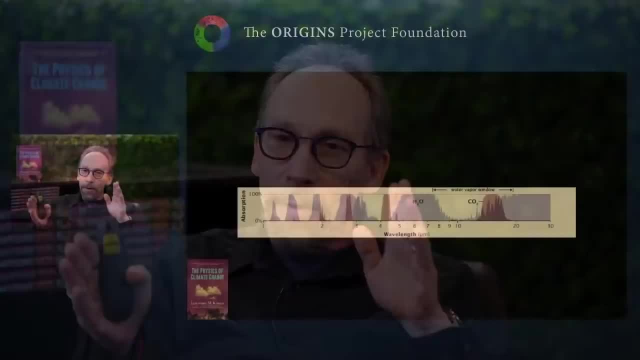 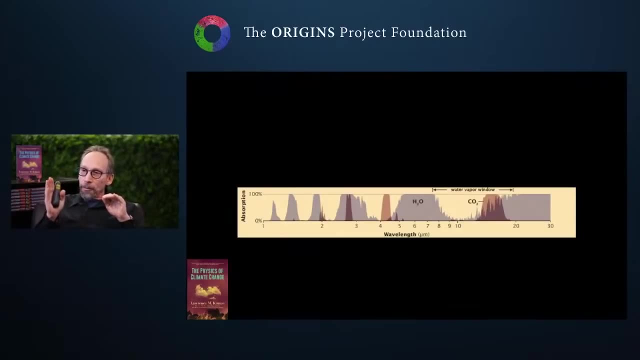 The problem is Knud Engström didn't realize he didn't have the resolution and spectroscopy that we now have to see that the water peaks were. there were many, many peaks in troughs, Whereas the carbon dioxide absorption peak is. 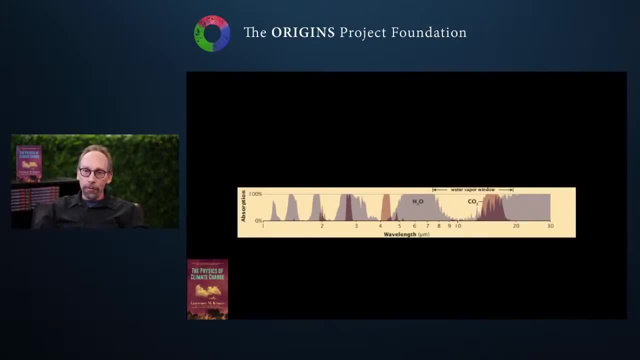 very broad and it can actually absorb between those hydrogen, those water peaks and can have an effect. But then he said it doesn't matter, because if once things are saturated, once you're absorbing 100%, it doesn't matter if you increase the carbon dioxide abundance. 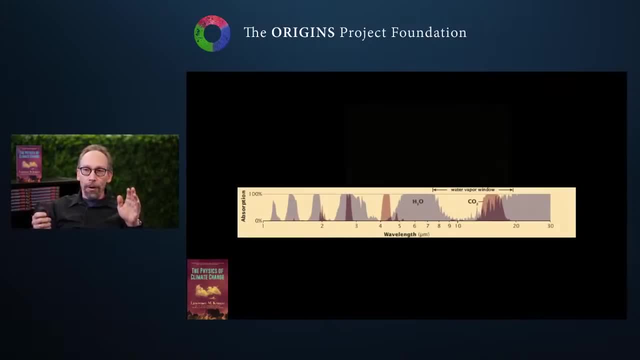 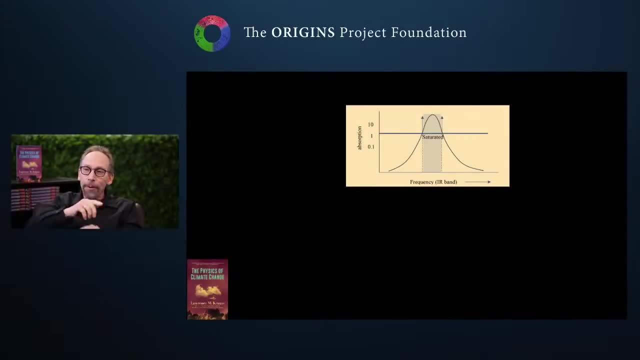 anymore. you can't absorb more than 100%. And he was right and wrong Because he didn't understand the nature of absorption peaks, which are not always at a single frequency but spread out. So here's just a schematic of one peak of absorption. Now, 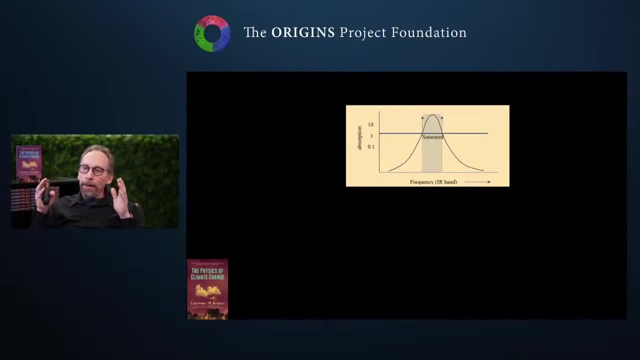 in the IR band. So say, in that peak the abundance of carbon dioxide is sufficient that at an absorption rate of 2, in this normalized value, at an absorption rate of 2, it saturates. Namely all radiation in that frequency band is absorbed by carbon dioxide. 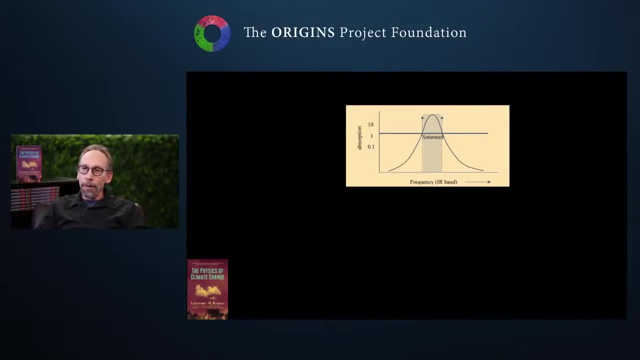 Okay For absorption factor of 2.. But if I increase carbon dioxide in the atmosphere by a factor of 4, then all frequencies where the absorption factor is bigger than 1 half will now be absorbed. But, as you can see, what that does is 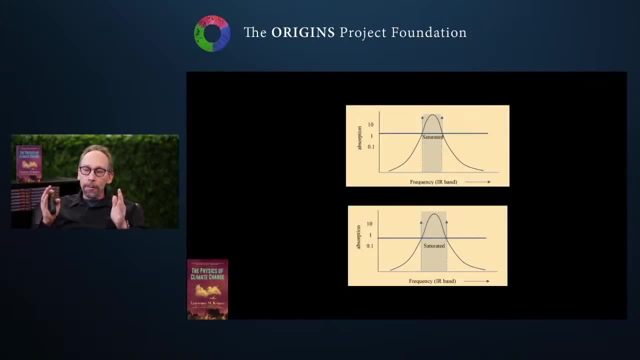 it increases the frequency range over which radiation is absorbed. So of course the region before, where things were saturated, is still saturated. but what Engstrom didn't realize is that you broaden the region and you open up more frequencies that can be saturated. 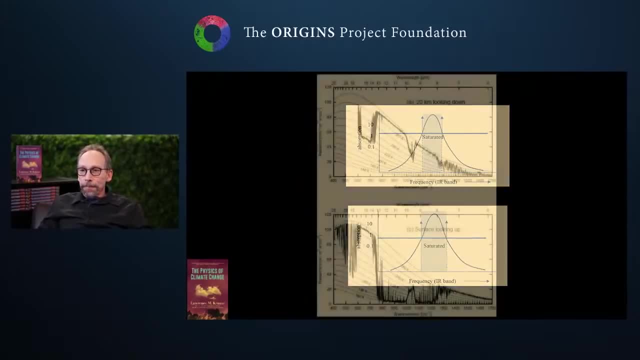 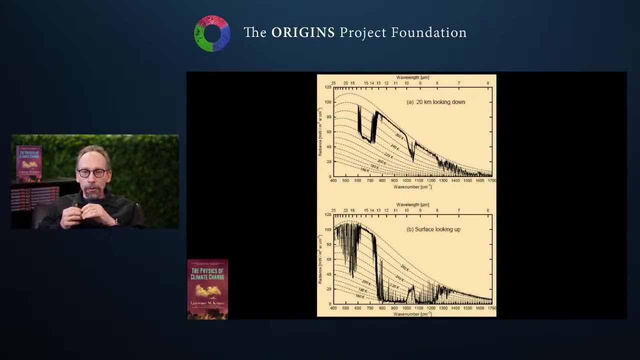 And this is a very important effect, as I'll show you Now. in fact, let's go from theory to data. This is some modern data taken, I believe, by a group in Wisconsin, and it's up in the Arctic Circle. Two different. 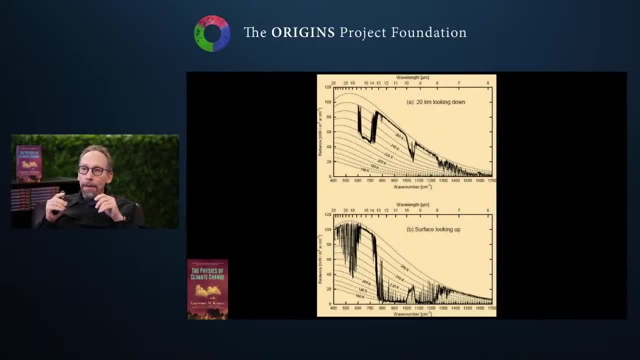 measurements: One from a satellite or a balloon at 20 kilometers looking down to the Earth, looking at the frequencies of radiation that are emitted by the Earth, and another with a detector on the Earth. Now, if you look at those dashed curves, what are they? 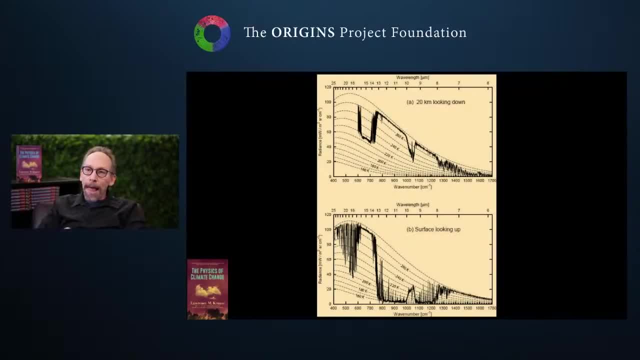 Those are called black body curves, Namely if you had a black body at a certain temperature. you can see one there: 260 degrees Kelvin, which is 0 degrees Celsius, is 273 degrees Kelvin, And so 260 degrees Kelvin. 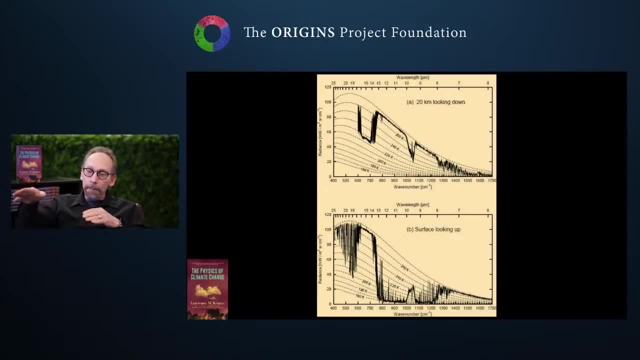 is below 0 Celsius. But if you had a black body, the Earth radiating at that temperature, it would emit radiation with that kind of general curve And what you can see if you're looking down is that in the regions 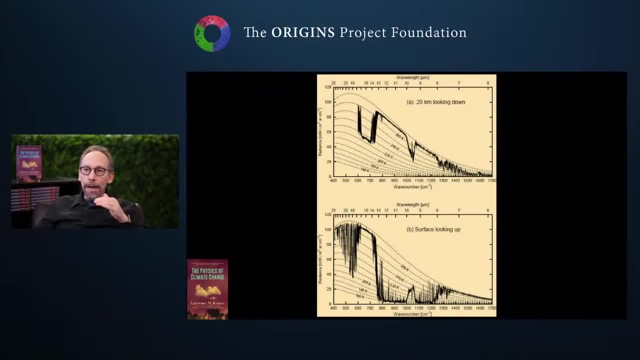 where carbon dioxide isn't absorbing radiation. you'll see radiation from, effectively, the surface of the Earth. This is in the Antarctic, below zero. You can see it's following that curve, But right there around a wavelength, a wave number, in this case, of a little over. 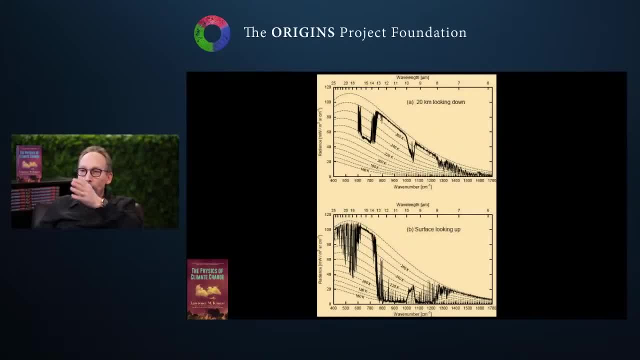 1,000 to 50,. that corresponds to around 10 microns. That's where carbon dioxide is absorbing and there's a lower frequency where it's also absorbing. You see, the characteristic temperature that it's now experiencing is crossing a curve that's much colder. 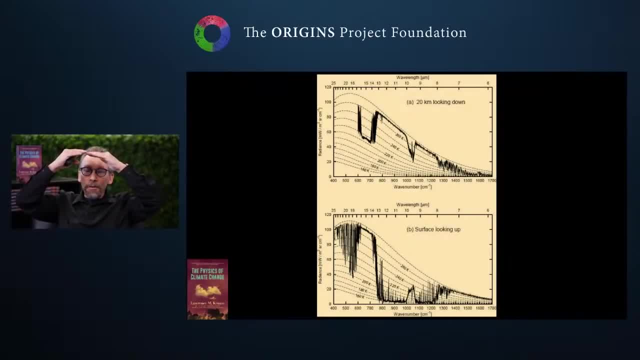 Why is it much colder? Because now, because carbon dioxide is absorbing all that radiation. now the atmosphere is emitting that radiation from much higher than the Earth's surface and it's much colder up there. So you're now seeing radiation being emitted. 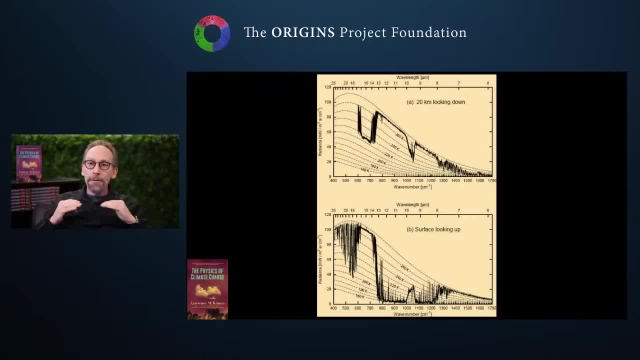 from a surface which is maybe 30 or 40 degrees colder than the surface of the Earth, and that will be an important effect. Also, if you're at the surface of the Earth, if you look at the lower curve again, if you're looking. 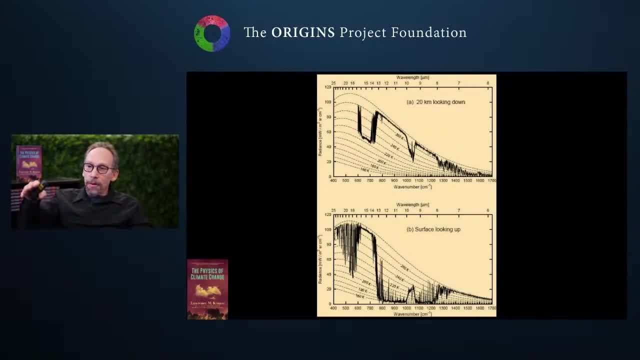 in the regions where carbon dioxide is not absorbing. then you're looking at radiation directly from space and you're seeing how much colder you're seeing- around 800 to 1,000.. It's much, much colder. It's following a curve of 160 degrees Kelvin. 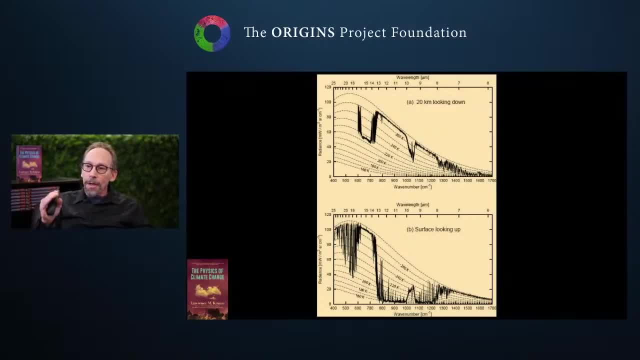 But right there, in that peak where carbon dioxide is absorbing, you're seeing, it's now much warmer but now characteristic around 230 degrees Kelvin and that's because now that region of frequency the atmosphere is absorbing the radiation you're not seeing it from. 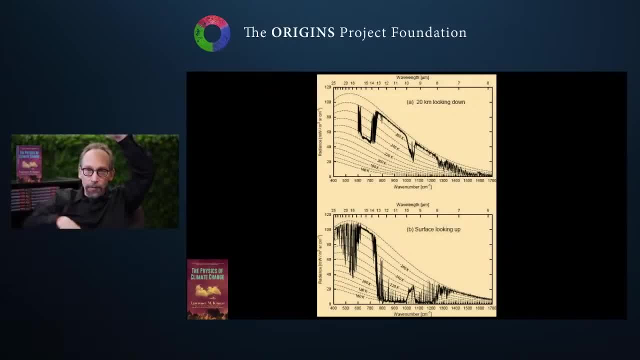 space. you're seeing the radiation being emitted from the surface of the atmosphere down, and that's why it's warmer than space itself. So you're seeing the effect I described, namely the fact that the atmosphere is absorbing in that frequency band, and that's the frequency. 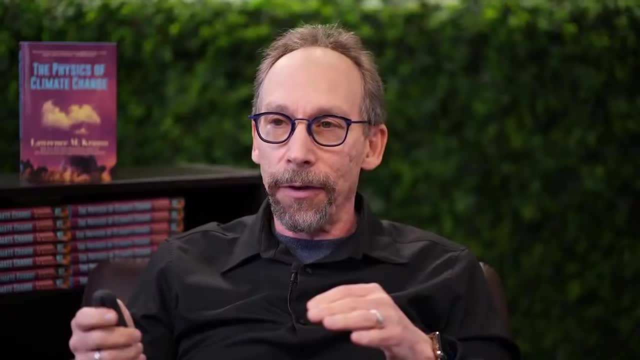 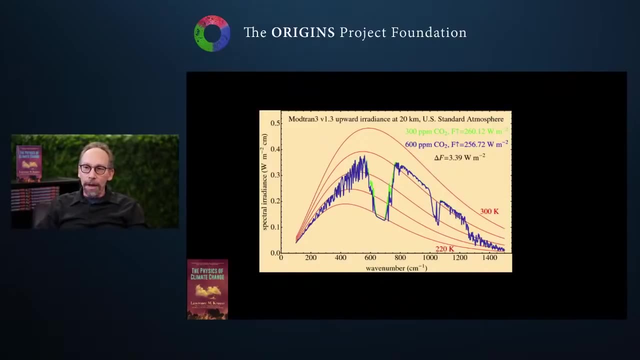 band that's ultimately producing what we now call the greenhouse effect. Now here is. here are theoretical curves based on the best atmospheric models you can have of what happens if you start out with 300 parts per million of carbon dioxide, which is, of course, much less than there was even 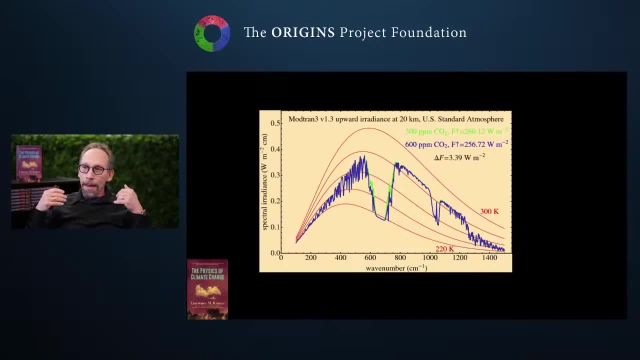 at the turn of the last century and you can calculate and you can see how much. in that orangey-red curve you can see that there's a trough where the carbon dioxide is absorbing some of the radiation that would otherwise go out into space. 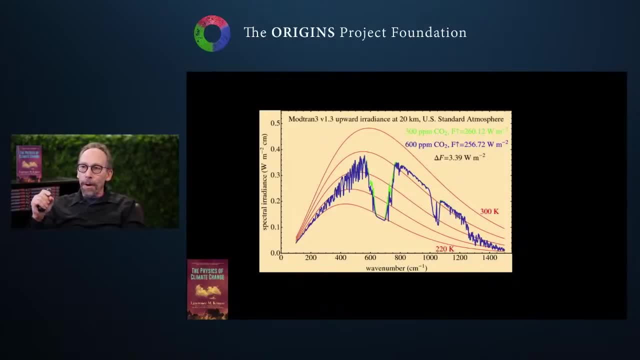 and you're seeing that basically the Earth is emitting around 260 watts per meter squared out into space because of that absorption. But if you double the carbon dioxide what you can see is the wings of that trough are a little bit broader. You know the curve I showed you. 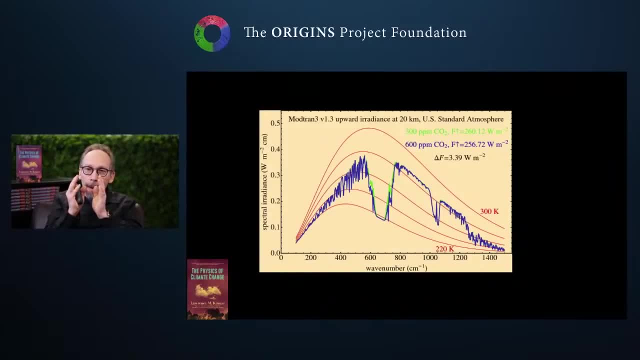 earlier the schematic curve was a much exaggerated version. but by increasing the carbon dioxide you're increasing the frequency range of absorption, In this case just by about one or two percent, but it's enough to lower the radiation emitted into space by 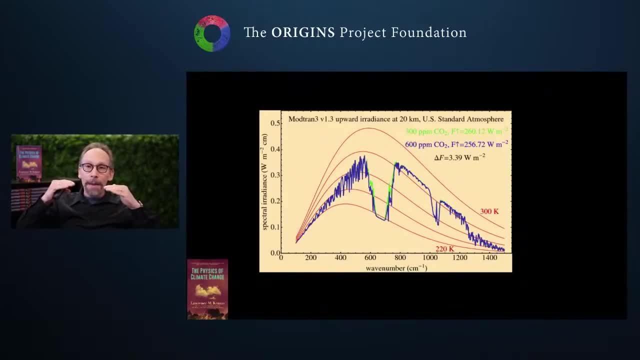 3.39 watts per meter squared And that produces an imbalance Because it says beforehand: when things were equal, when the power in equaled power out, the temperature was remaining constant. but now, when you add carbon dioxide in the atmosphere, 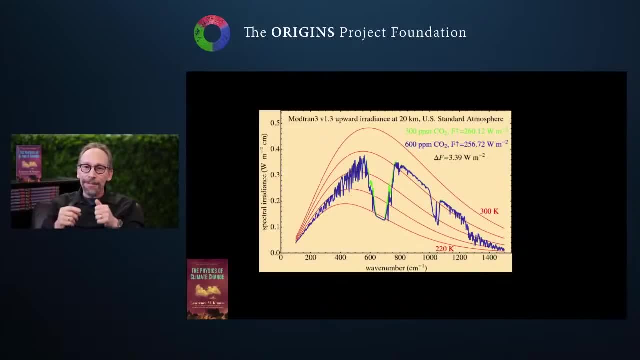 the power you're emitting is 3.3 watts per meter squared, less than it would be otherwise, and that's radiation that heats up the Earth. 3.3 watts per meter squared may not seem like a lot, but when you multiply it, 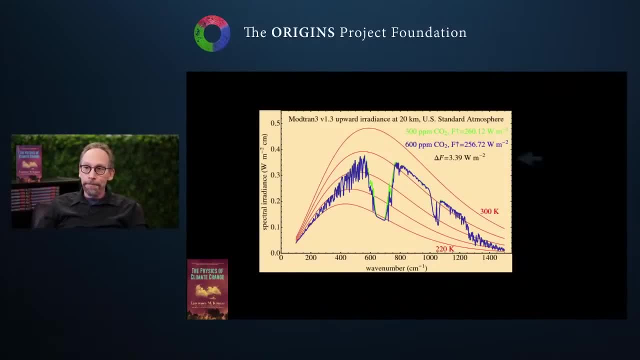 over the entire surface of the Earth. it's a lot of heat, And that is basically the fundamental quantity that is relevant for understanding climate change. It's called radiative forcing. We can measure it and we can predict it, And it's a few watts per meter squared. 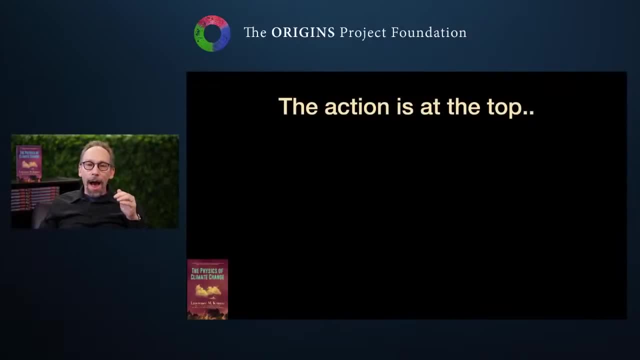 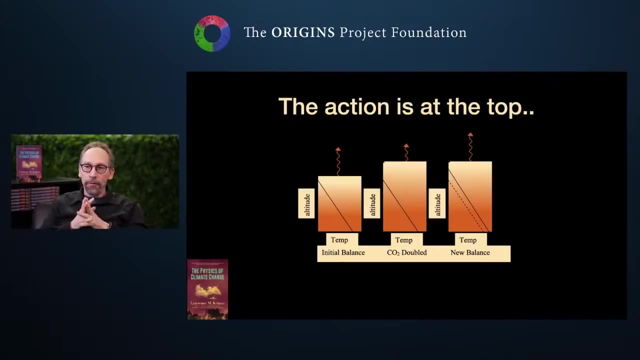 Now this is really how carbon dioxide heats up the surface of the Earth. Really, the action is at the top of the atmosphere. So originally let's say we have 600 gigatons of carbon in the atmosphere in 1900,. 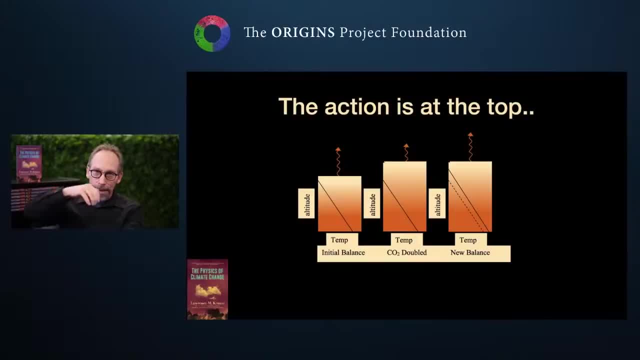 and we have a temperature imbalance and the radiation out is equal to the radiation in, And the length of that little squiggly line is the power that the Earth is emitting into space and in equilibrium that power is equal to the total amount of radiation coming in. 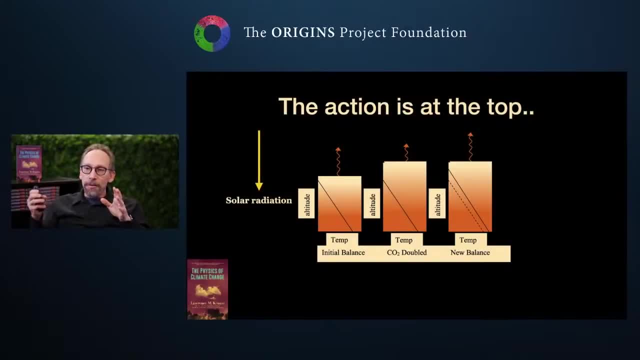 So things are in balance. What happens if you double the CO2?? What happens is because CO2 is absorbing the atmosphere. the point in the atmosphere where radiation is now free to go into space is higher up, because more of the atmosphere is opaque. 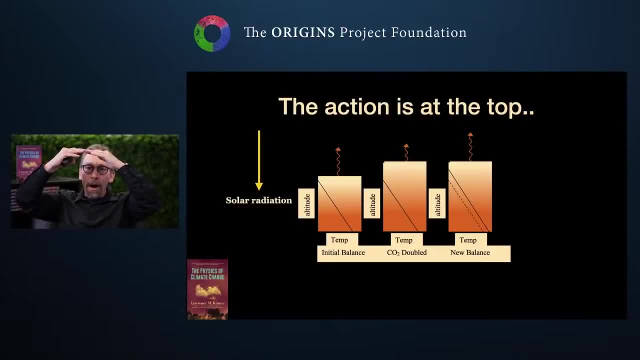 So the atmosphere is emitting radiation from higher up, but at a higher altitude. it's colder, So the atmosphere is emitting at a colder temperature And since the radiative power goes as the fourth power of temperature, that means the atmosphere is emitting into. 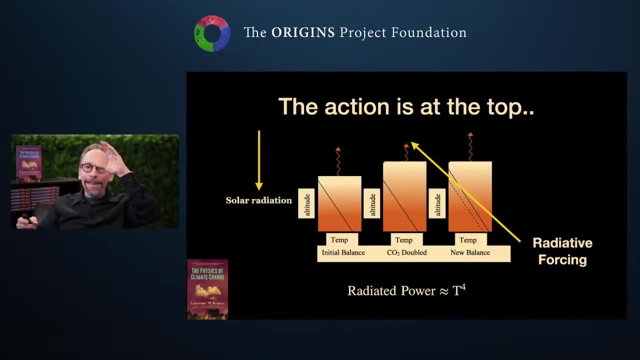 space less radiation than would be otherwise, and the gap is what we call radiative forcing. Now, eventually, if nothing else changes, eventually you'll get to an equilibrium again where, basically, the top of the atmosphere will be hotter than it was before and you'll be emitting. 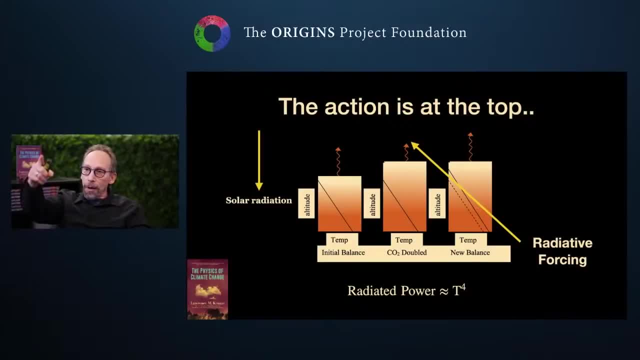 as much radiation as you were before. but if you look at those curves, the lines, if the top of the atmosphere is hotter than it was before, then the surface of the Earth is hotter than it was before And that's the greenhouse effect. 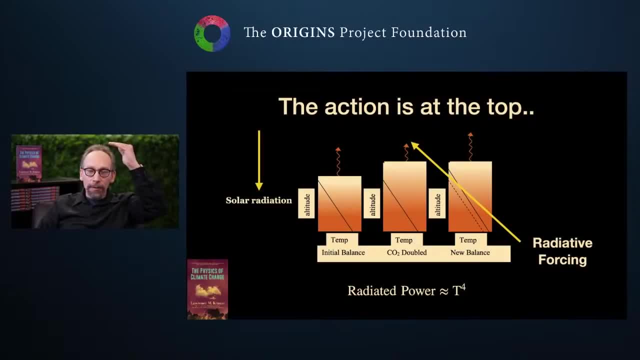 The greenhouse effect is really an effect that's occurring at the top of the atmosphere and first what it does is produce an imbalance where more energy is stored in the Earth than is radiated and the Earth heats up. but eventually the Earth heats up, so the top of the 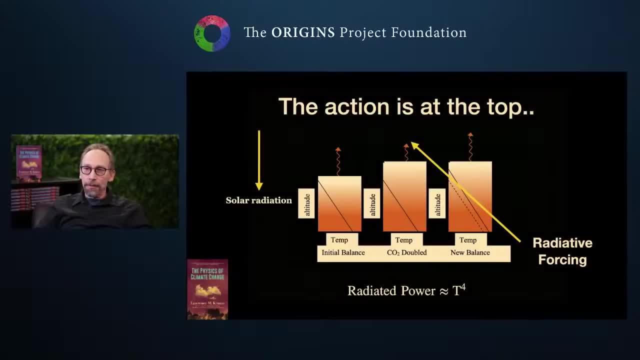 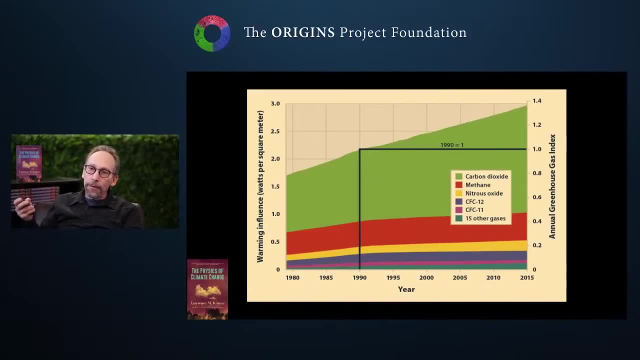 atmosphere heats up, but so does the bottom of the atmosphere where the Earth is, And that's the substance. This is measuring, basically the effect of radiative forcing due to different greenhouse gases. Carbon dioxide is just one of them. There's methane. 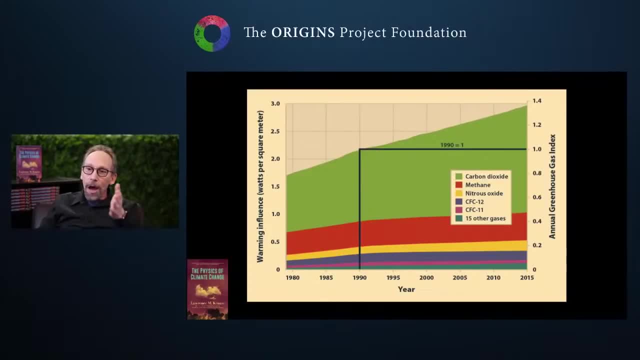 nitrous oxide, other gases, including water, and you can see how, over the period from 1980 to 2015, that radiative forcing effect has gone up from about 2 to almost 3 watts per meter squared due to just those quantities. 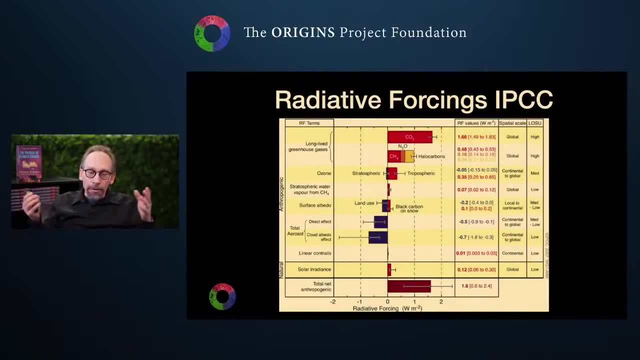 Now the Intergovernmental Panel on Climate Change produces regular reports, and this is one of the more recent reports. I think this one's from 2012,, but it might be from 2018.. I forgot which one I picked for this. 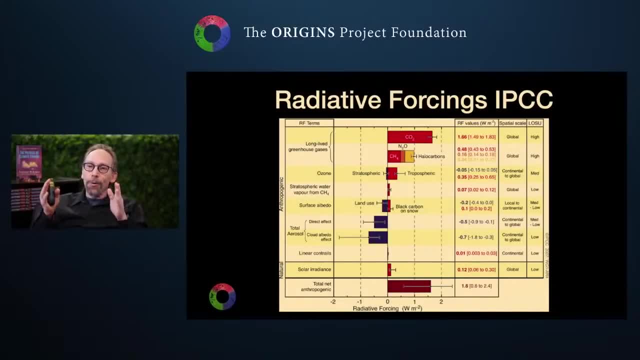 image And it measures the radiative forcing, which is the key effect, And you can see that carbon dioxide is by far the largest impact here in the radiative forcing. This is the relative radiative forcing compared to 1900.. Compared to: 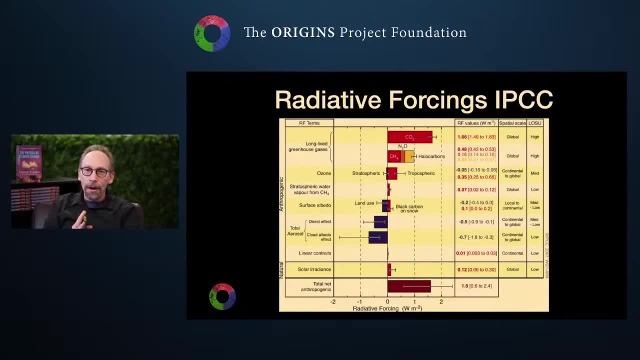 what it was when there was basically 600 gigatons of carbon in the atmosphere And you can see that the increase in carbon dioxide between then and 2012 has produced that radiative forcing. But there's methane, nitrous oxide, various 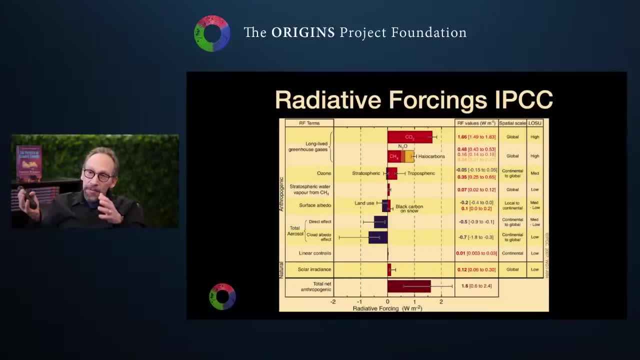 halo carbons. There are other effects. For example, some land use reduces causes- reflection of light, if you wish, and reduces the absorption of radiation in the earth. So do clouds. But when you include all of these effects, the net anthropogenic, the net. 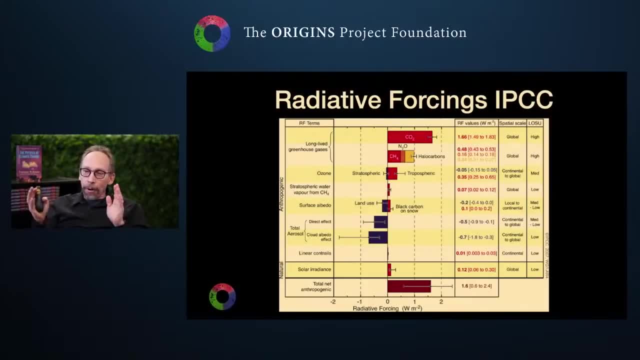 radiative forcing produced by humanity is around averages, around 1.6 watts per meter squared at this time And that has produced a temperature change which, in fact, if you actually I describe in the book how we can kind of calculate this. but ultimately, 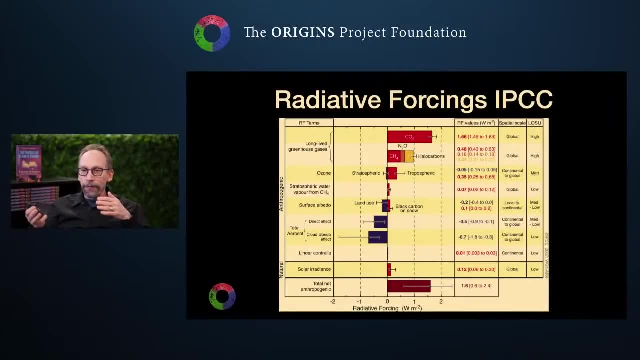 it turns out there's more or less a linear relationship between the radiative forcing and temperature change And the factor is about 0.75.. So if you multiply 1.6 by 0.75, you get you predict about 1.2 or 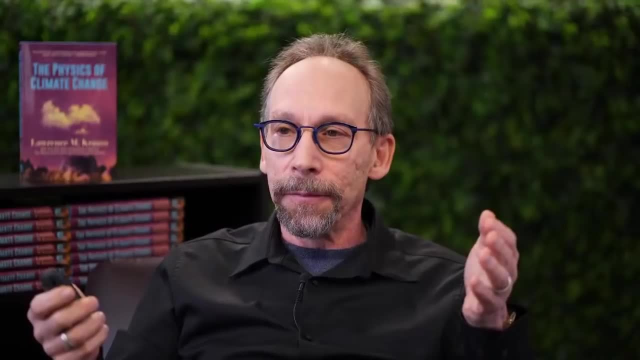 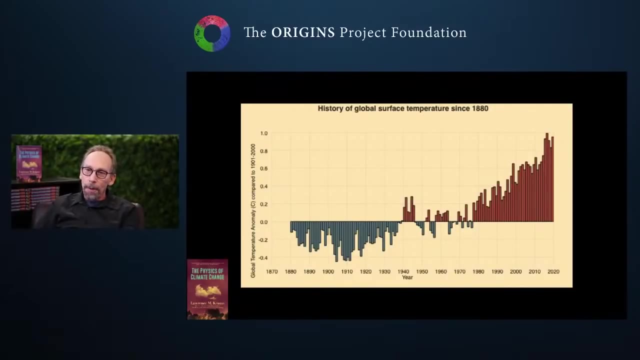 1.3 degrees of warming since 1900.. What have we seen? Well, if you look at it since 1900, where in that curve you see the global temperature was about minus 0.4, it's normalized to be 1960, to be 0.. 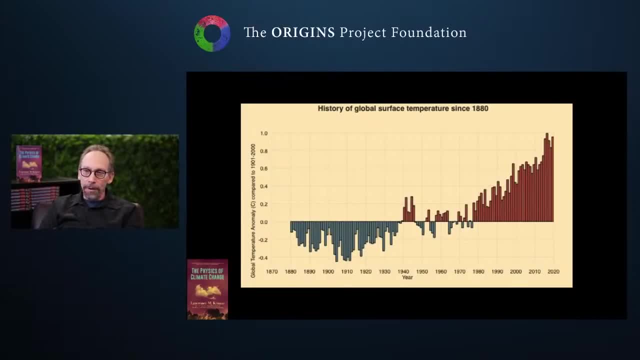 So it's about 0.4 degrees Celsius below that in 1900.. It's 1 degree about 0.9 degrees above it in 2020.. You add the two, you get 1.3 degrees Celsius. You get exactly. 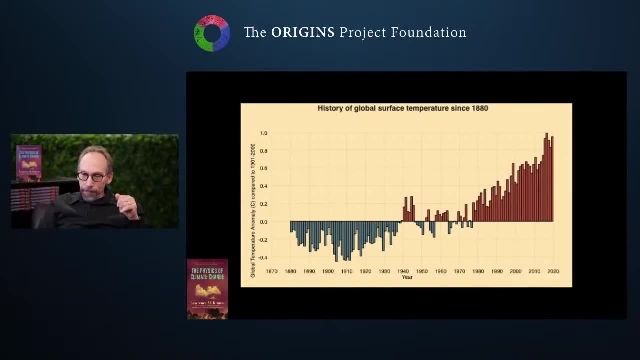 what you'd predict essentially. Now, this is really important because people often point out, and I often point out, that correlation is not causation And therefore correlating temperature to carbon dioxide themselves doesn't show you that carbon dioxide is responsible for heating the atmosphere. 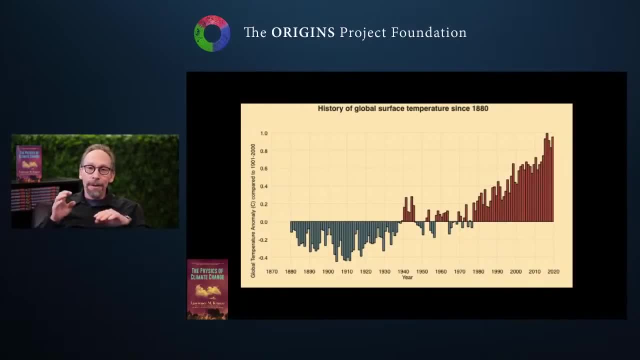 But if you have a theoretical prediction that tells you why you should have that correlation, then correlation may be causation And when you, when this predicts, bang on exactly what you see. and if it walks like a duck and quacks like a duck, it's probably. 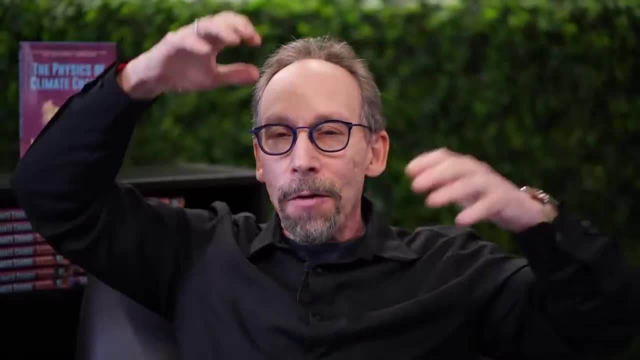 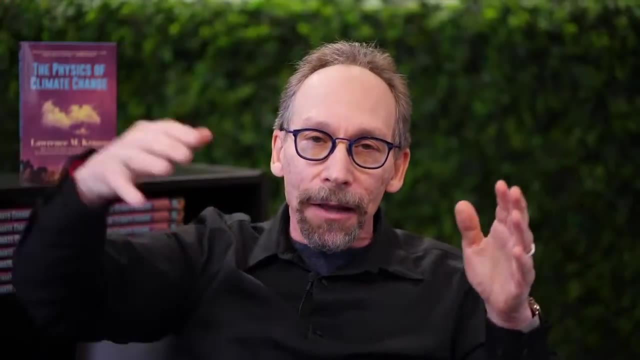 a duck. I mean you could argue that maybe there's some conspiracy, that many other things that cancel out everything completely, can't make our, that cancel out all the predictions that we make and something else is responsible. But here a simple basic. 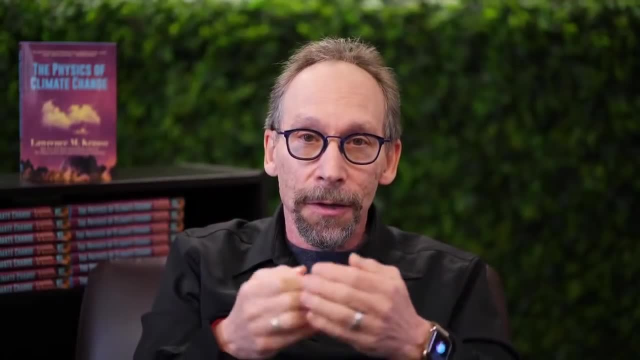 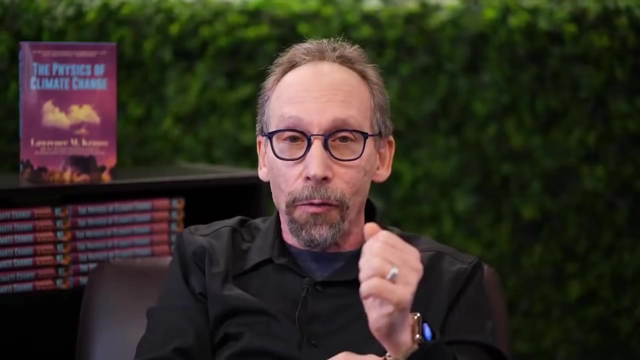 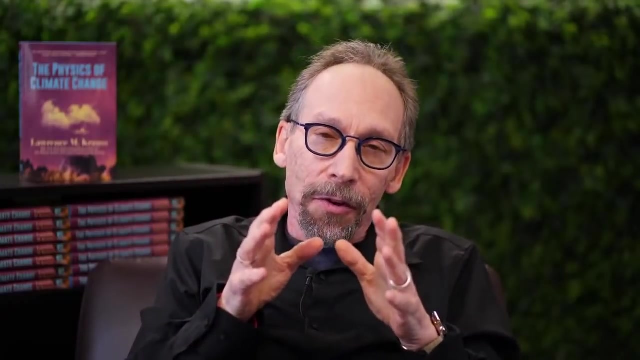 calculation which is really based on 150-year-old physics- Nothing you know. high school level physics, as I discuss in the book, developed sometimes accidentally by scientists over that period, predicts exactly what we're seeing Too often because, of course, the details of climate change. 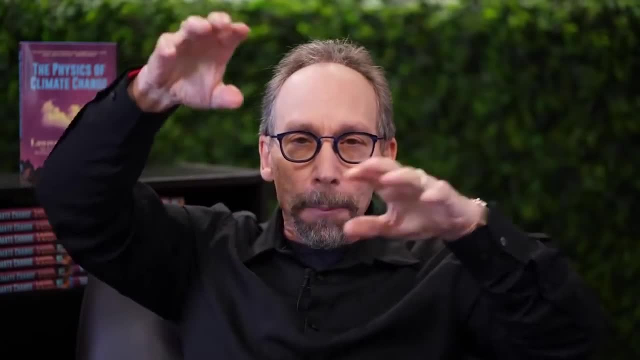 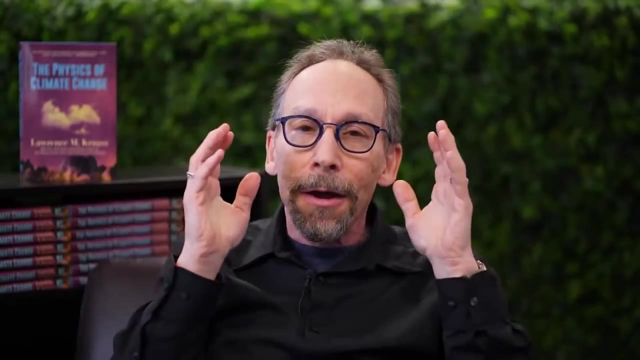 how climate is going to affect currents and temperatures across the globe, which I talk about in the book too. that requires super computer models of the atmosphere and the earth And people think, well, I don't trust those. Those predictions are not believable. 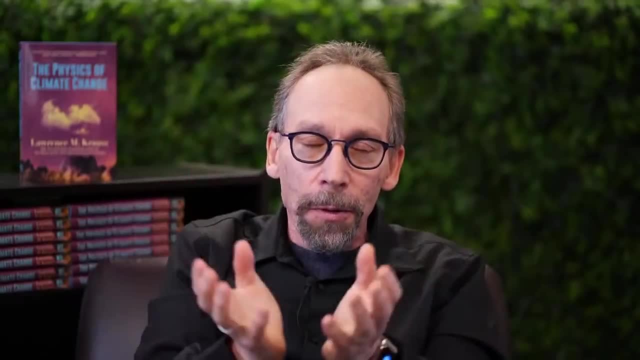 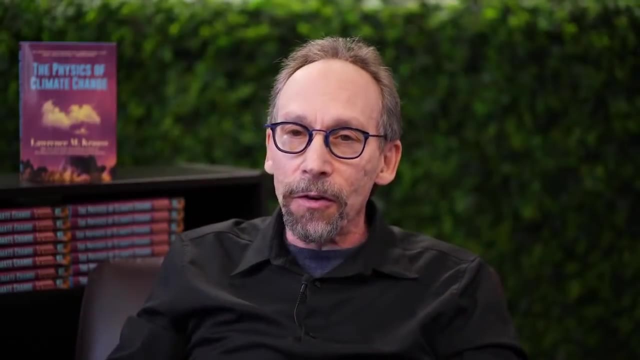 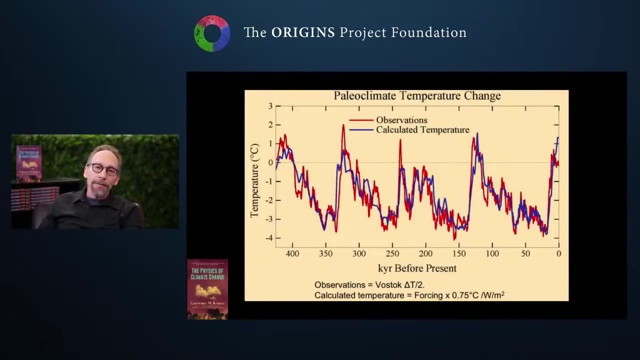 But in fact the fundamental prediction of the global temperature rise is: it doesn't require super computers, it just requires basic physics, And the physics agrees with observations. Okay, If you don't, if you think it's an accident, here's a. 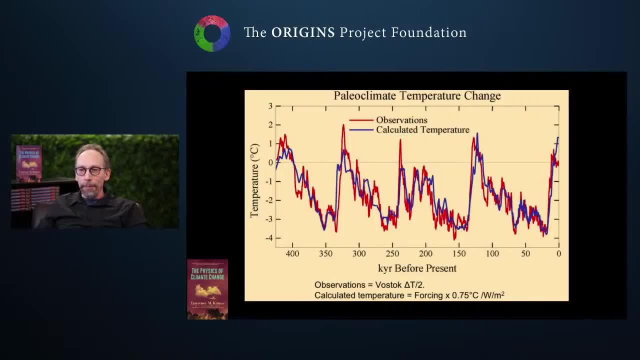 curve. I got from Jim Hansen, a very well-known climate scientist, and this is just looking at the observations of temperature, because you can actually measure by looking at isotope ratios in ice cores. you can also measure the temperature over periods of the earth. 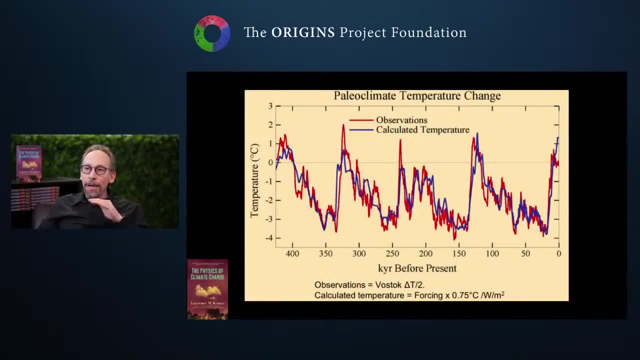 going back 400 or 800 thousand years and just taking the observed carbon dioxide and multiplying by 0.75, a very rough thing- you can see what good agreement you have. So if you don't believe what's happening now, you can see that. 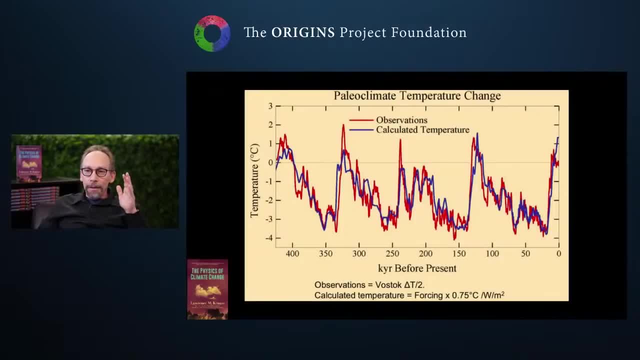 over a 400 thousand year period. understanding the forcing produced by climate, by carbon dioxide in the atmosphere, and comparing it to the observed temperature, gives you a pretty good agreement. And again it tells you the physics is working And it's unlikely that there's some. 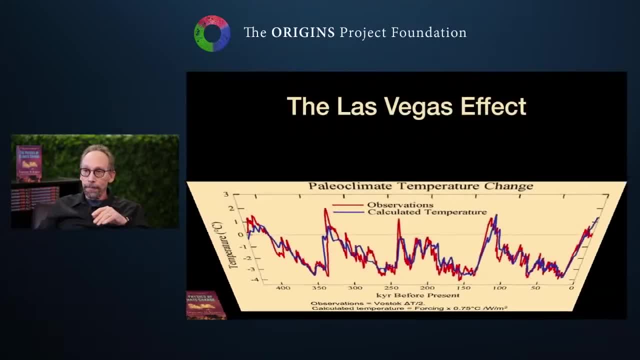 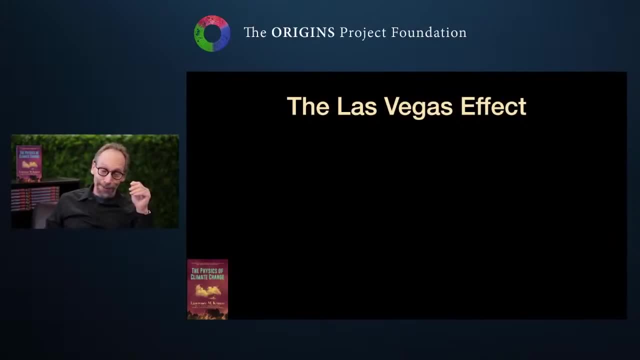 hidden conspiracy going on that's cancelling out the well-known physics. Now the next thing I want to talk about is the Las Vegas effect. What I call the Las Vegas effect, Namely, what happens in the atmosphere stays in the atmosphere. And the really important- 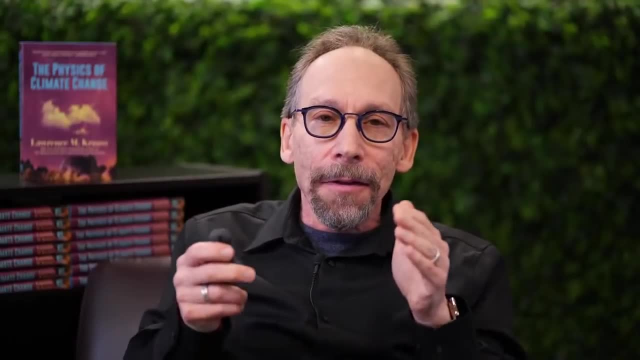 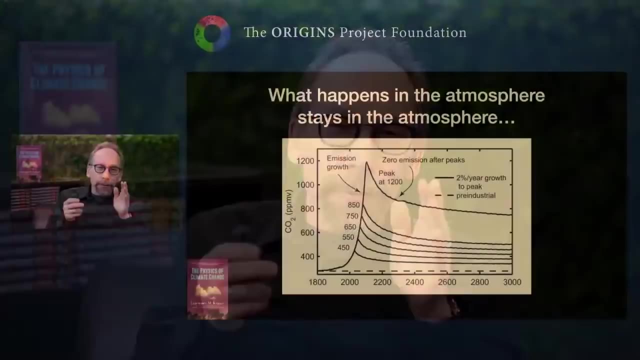 thing that is important for us today is that the carbon we're putting in the atmosphere, the abundance of carbon in the atmosphere we put in there, will remain up there for not decades but centuries. Here's a calculation, and there are many different calculations that have 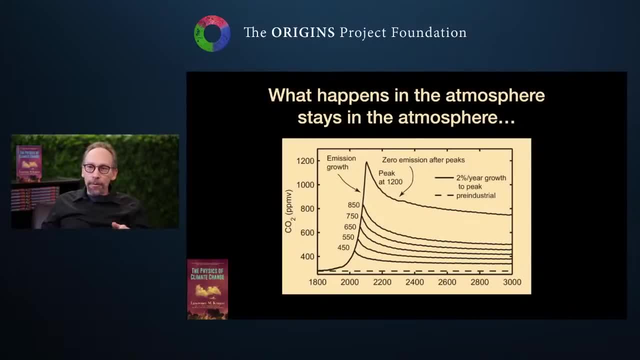 been done. that say: look at carbon in the atmosphere. So let's say we turned off all carbon in the atmosphere right now, around 450 parts per million, 440 parts per million. What would happen? Well, individual carbon dioxide molecules get exchanged with the ocean. 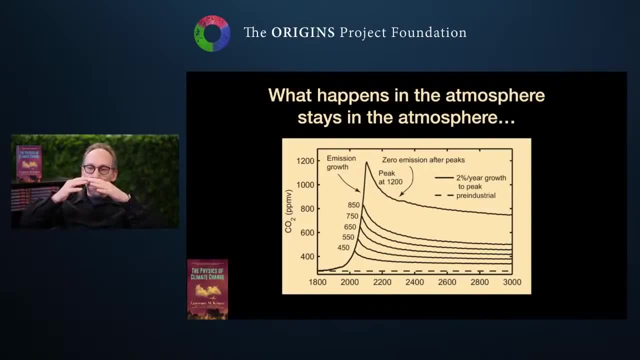 as I told you, and they have a lifetime of just years, But the net abundance doesn't change. The fall off is, if you look at it, about 60%, even a thousand years later, about 60% of the carbon abundance in the atmosphere. 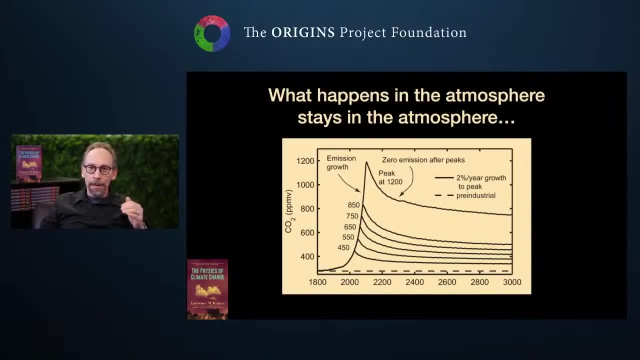 that we've put up there will remain there. So if we're at 470, 417 parts per million and we turn it off in a few years at 430 or 440, about 60% of that, about 3 to 400. 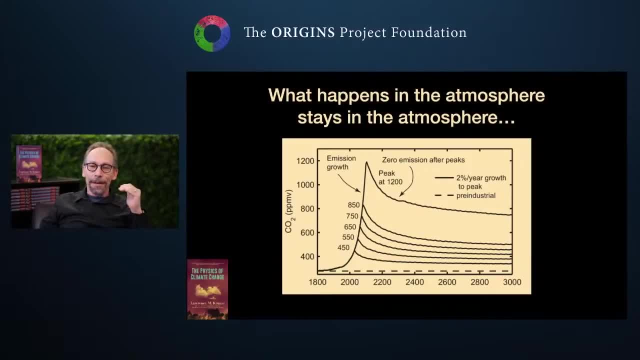 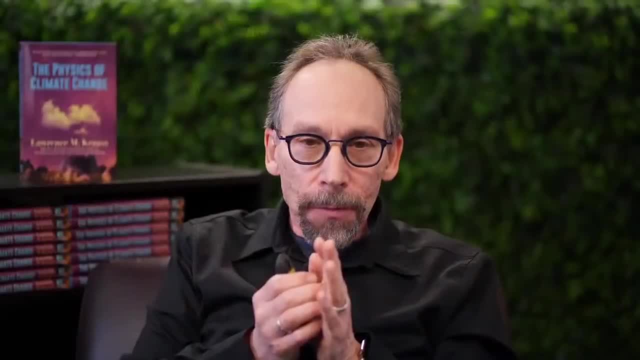 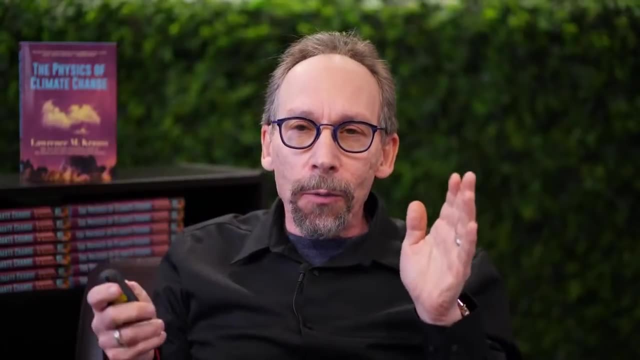 parts per million will be up there still a thousand years from now. And that's the reason there's some urgency to this, Because people often say: well, we can wait, Maybe it's going to produce financial hardships now to do something about it. But every year we wait. 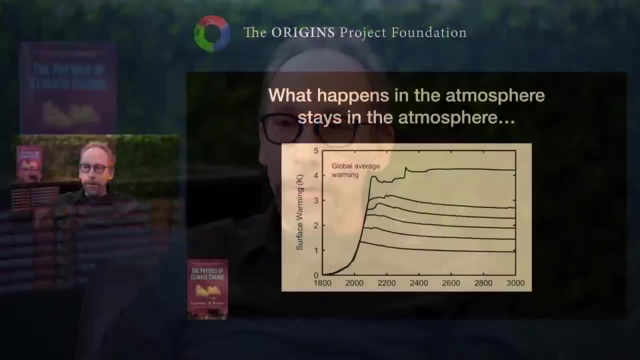 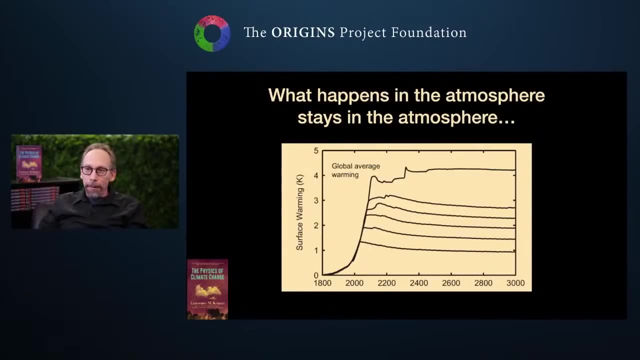 exacerbates the situation. By the way, this is the same computer calculation for what the global temperature warming is. You can see that if we turn it off now, the average warming compared to 1800 or 1900 is about 1.3. 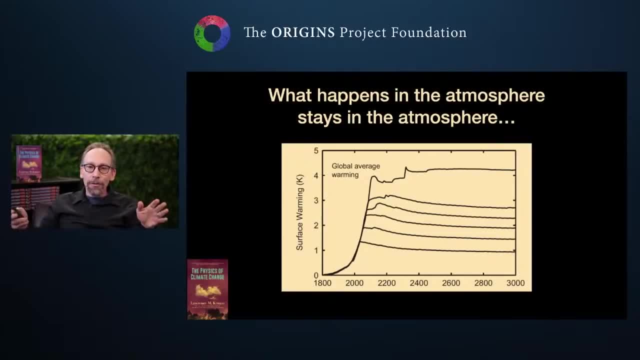 degrees, That warming is going to stay there. There's nothing we can do, even if we stop producing carbon dioxide right now. unless we take carbon dioxide out or do something more dramatic, that's going to change that. That warming is written in stone. 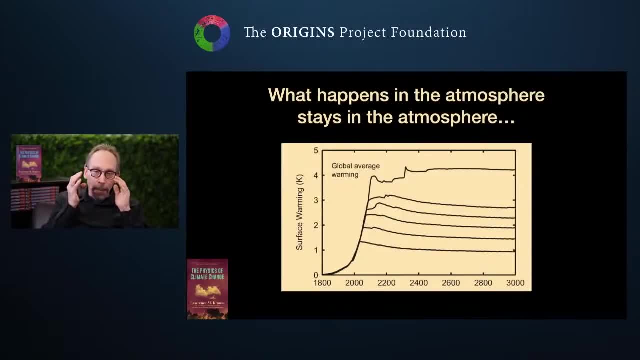 And we'll come back to that, Because I think it's really important, when you talk about the predictions of climate change, to talk about what's written in stone, what's firm and what's more speculative, And you can see if we continue business. 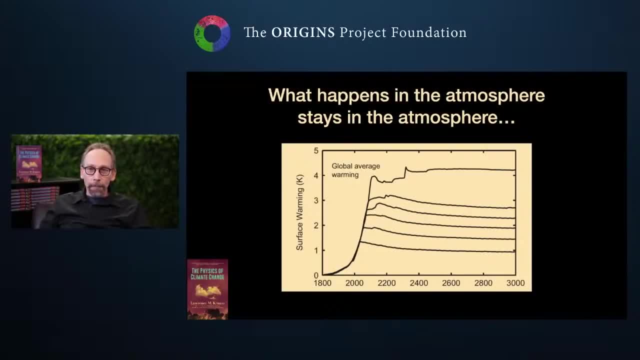 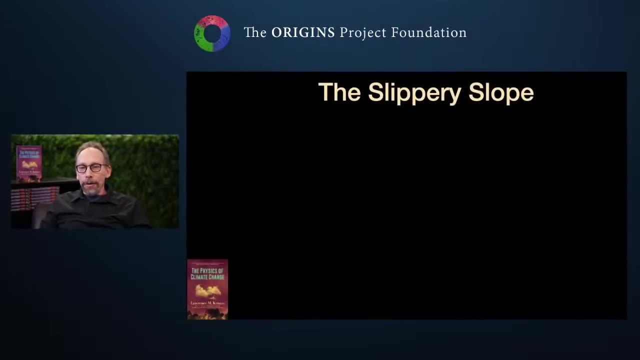 as usual and don't reduce our carbon production in the atmosphere, we're going to have about 4 degrees of warming by 2100.. And that's going to remain that way for a thousand years Now. the Copenhagen Dialogue about 30 years ago. 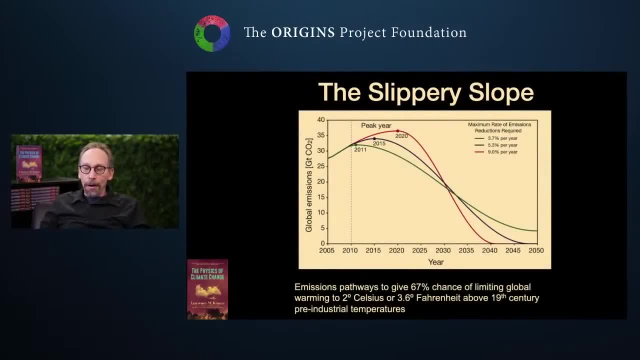 produced what was called the ski slope curve. I call it the slippery slope. Basically it says: let's say we have a target. We want to limit global warming to 2 degrees Celsius. It's an arbitrary number. It's not as if the world is going to end if it's 2.1.. 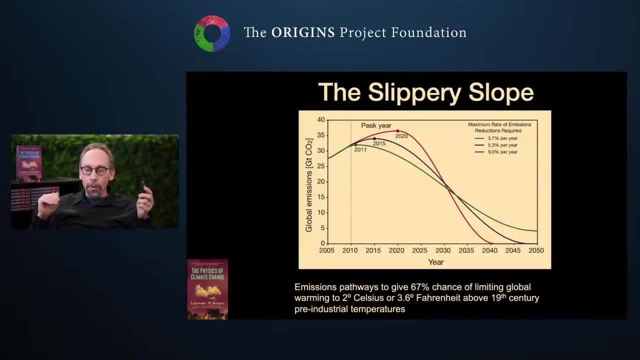 But it's a target You can say: we don't want things to increase more than 2 degrees Celsius above the 19th century value. What are the emission pathways? given 67% chance of limiting global warming to that? Well, if we. 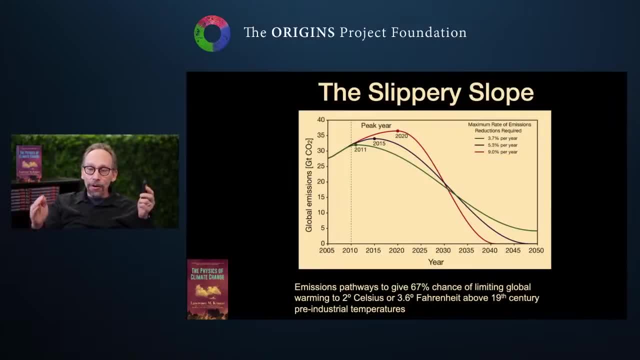 basically started turning the curve. over 10 years ago, we would have had to reduce our emissions by 3.7% per year, But now, because we haven't turned the curve and we've been producing more and more each year in order to reach that goal, 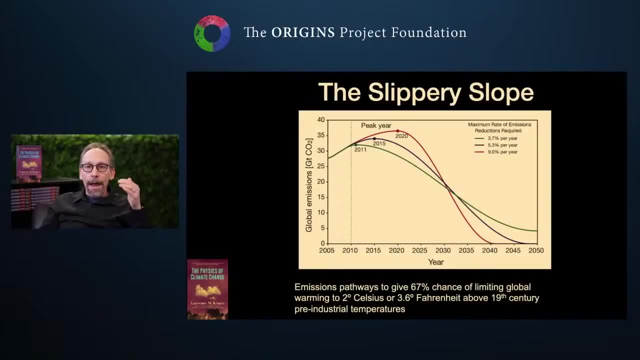 we have to reduce it by 9% per year And therefore the requirements on us to do the same thing are more dramatic. every year we wait. Every year we wait, we're adding 10 gigatons of carbon in the atmosphere, 5 gigatons of which just stays there. 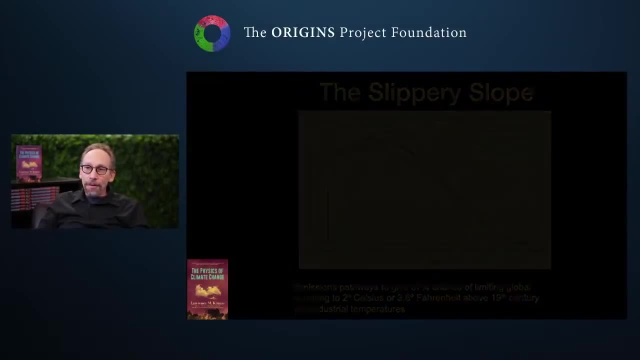 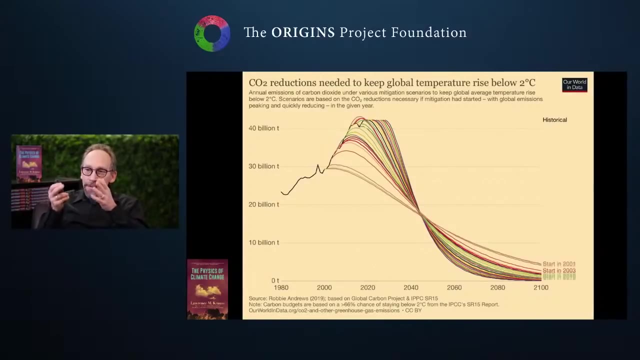 and that's 5 gigatons. that's not going to go away And you can see it's gotten even worse. That was a plot done in 2010, but here's a plot today. You can see that today, basically by- if we don't turn things around, by- 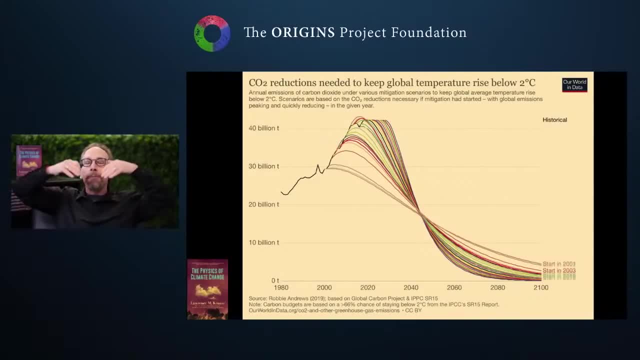 2025 or 2030, there's nothing we can do. We'll have already dumped enough carbon in the atmosphere that we're going to have a 2 degree temperature change. But if we want to try and limit things as the Paris 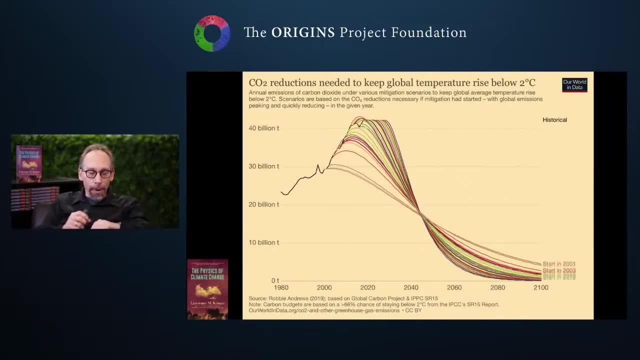 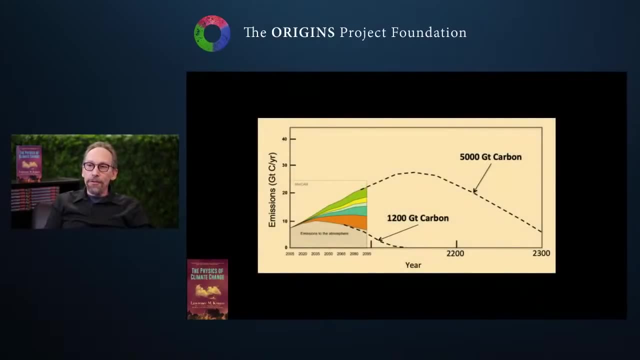 Accords wants to do. every year we wait. what we have to do is more dramatic Here. by the way, just to give you a sense, remember there was 600 gigatons of carbon in the atmosphere before the industrial times, If we turn. 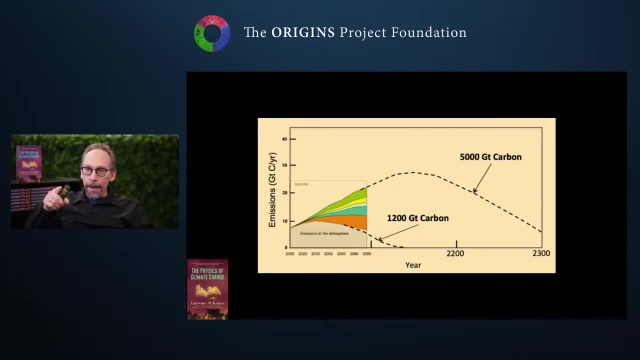 things around around 2030 and follow that lower curve, the net abundance of carbon in the atmosphere by the time we basically produce zero carbon emissions will be about 1200 gigatons of carbon. We'll have doubled the amount of carbon in the atmosphere. 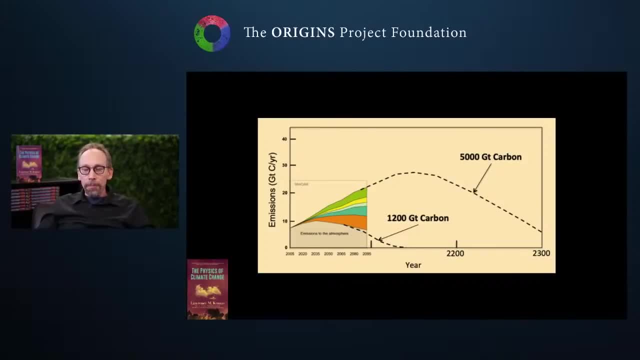 since before humans started spewing carbon into the atmosphere beyond their breathing. If we don't, if we consider business as usual to 2100, if we don't lower things by then the total amount of total amount of carbon we'll have added in the atmosphere. 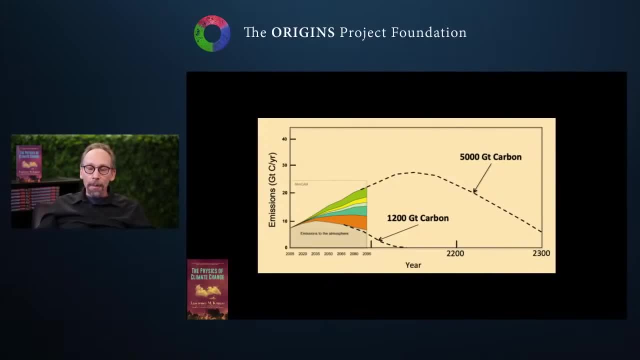 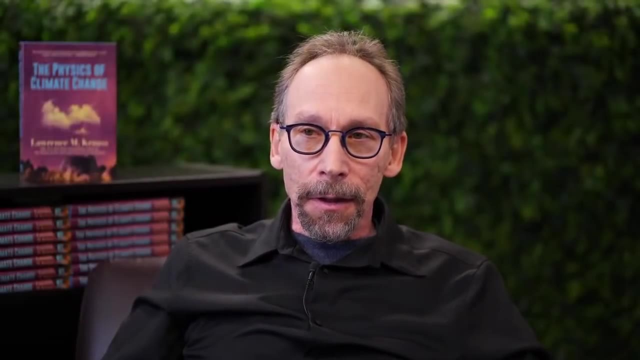 is 5000 gigatons- Almost 10 times more carbon. that was in the atmosphere in the turn of the industrial era and for recorded Earth's history back for at least a million years. We're dramatically changing the climate that way Now. 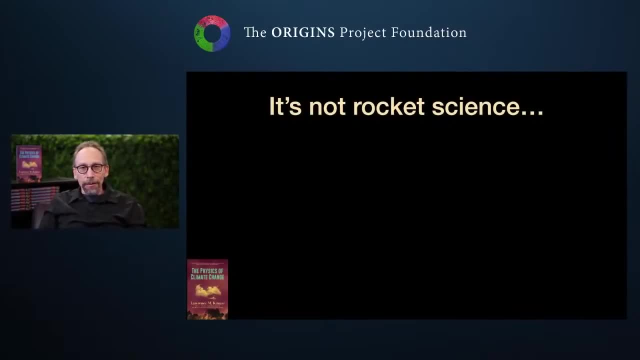 the last thing I really want to talk about before I go back to the Mekong, I think is- is this fact that it's not rocket science, And I wrote a book about rocket science. well, imaginary rocket science, the physics of Star Trek. 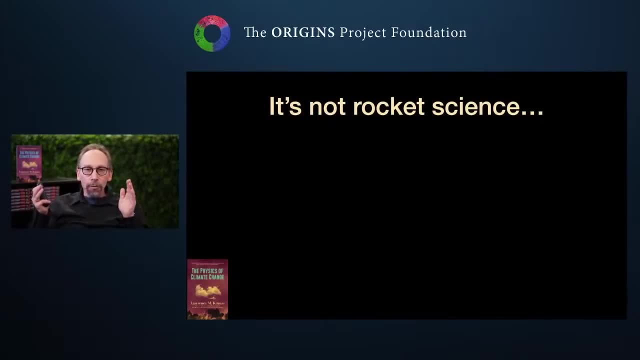 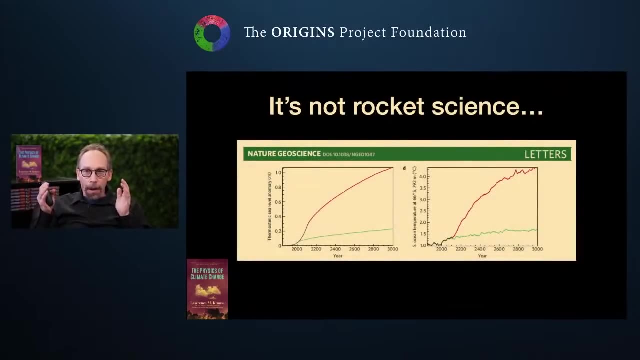 But people often think that a lot of these predictions require serious, detailed models and they're not believable. Well, here's a prediction that doesn't require anything but high school or middle school science. Namely, we have dumped heat into the ocean in the last 25. 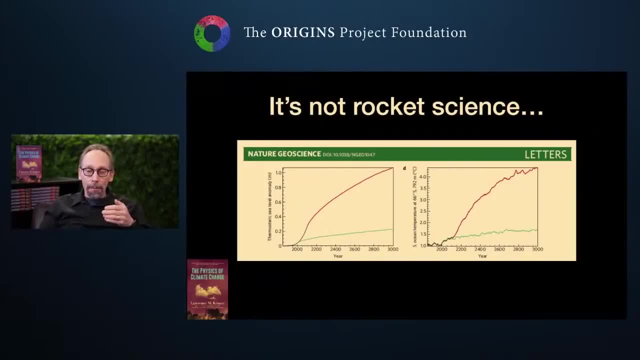 years, due to radiative forcing, We've dumped heat and I'll tell you how much That heat gets equilibrated in the ocean. It takes a little while to do it And you can see two curves here from predictions. One, assuming we turn off. 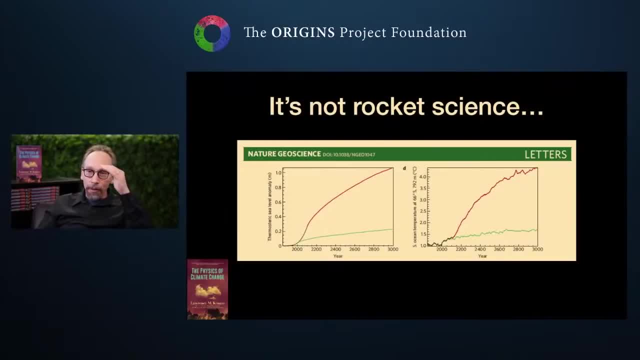 carbon production around 2010 or 2020.. The other saying we turn it off around 2100.. That heat heats up the oceans and when water is heated up it expands And we can see that roughly 20 centimeters, two tenths of a meter of sea level. 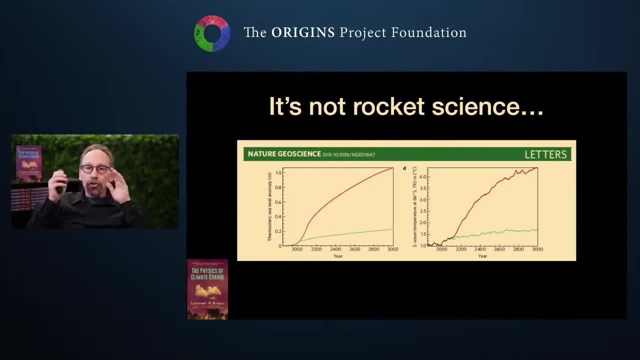 rise will happen by 2100 or so close to that, just independent of glaciers melting or what happens in the Arctic or ocean currents or anything else. just because the sea level is going to heat up and rise, It's not due to anything. 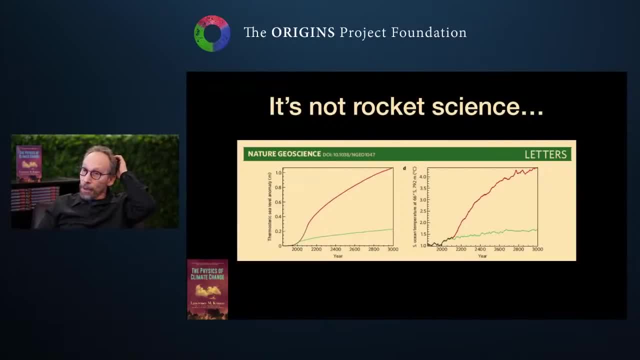 similar, more serious, If we continue business as usual until 2100, you can see that we're going to ultimately produce one meter of sea level rise over the long run as that heat gets equilibrated in the ocean just due to the expansion of water. 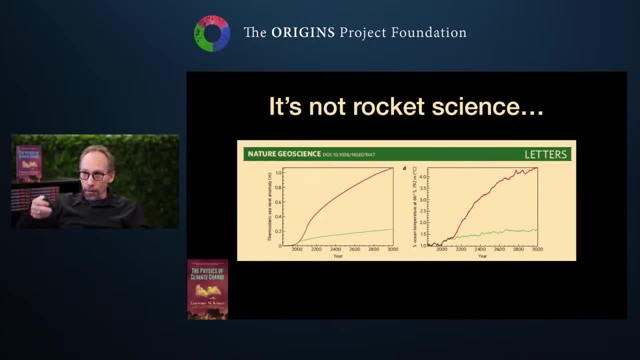 And you can see that the heat the sea level rise corresponds to the temperature increase in water as measured there. Now, if you want to get a sense of what's happened, in the last 25 years the average temperature of the oceans has increased by 0.75 degrees. 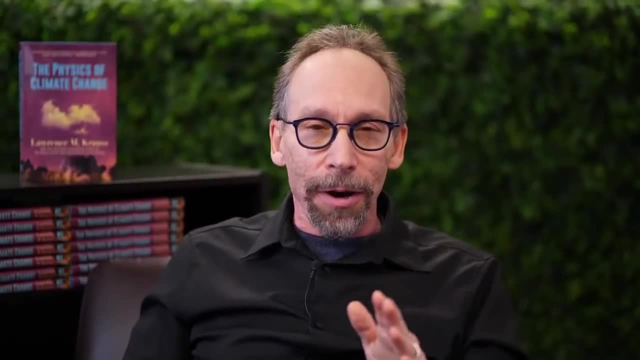 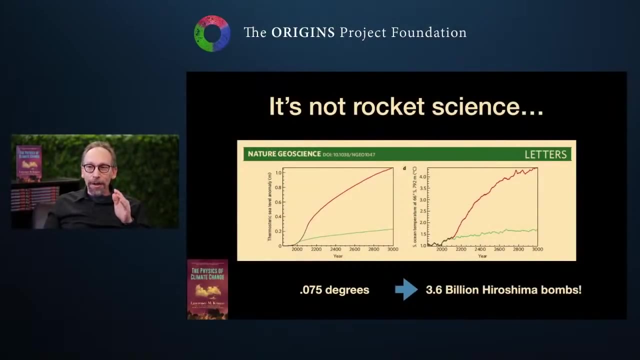 That may not seem like a lot, but a Japanese collaboration turned that into another number said it's the equivalent of having exploded 3.6 billion Hiroshima level bombs into the ocean over the last 25 years. Four atomic bombs worth of heat. 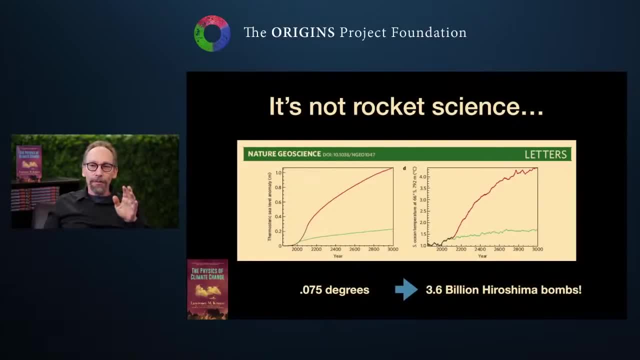 every second, 24 hours a day, for the last 25 years And that, as I say, is written in stone. No matter what we do now that's the kind of sea level rise we're going to get Some fraction of a meter, a fair fraction. 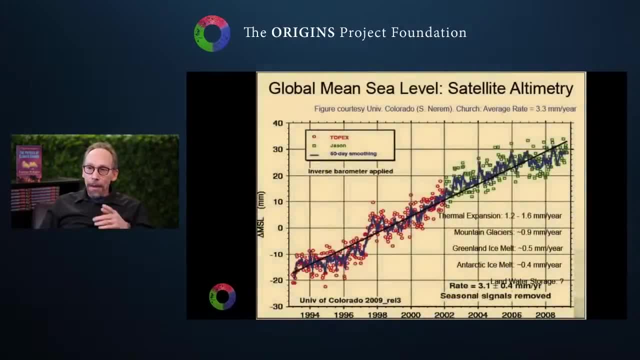 of a meter, And that can be significant. By the way, just to show you, this is measurements that were done up to 2008.. This is the sea level rise. measured sea level rise and thermal expansion corresponded to about half of that. Half of that came. 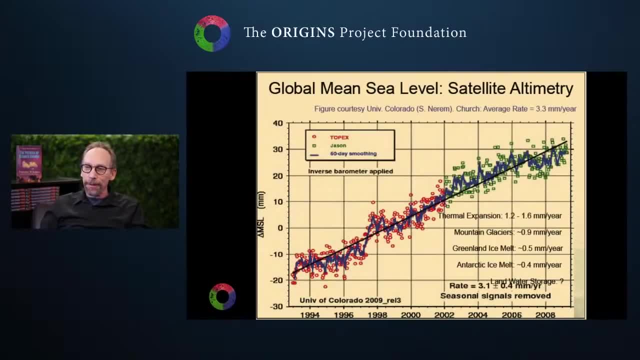 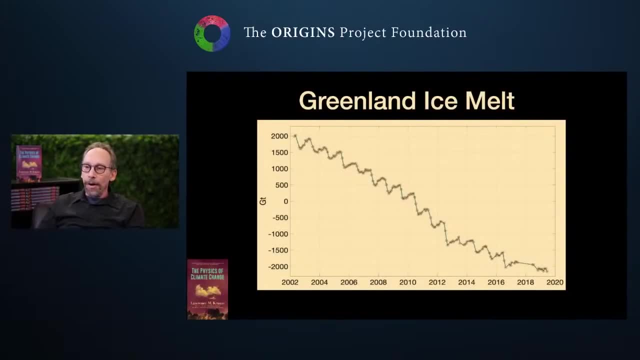 from mountain glaciers and Greenland and ice and the Arctic ice melting. Now Greenland and Antarctica are melting faster. Here's the amount of the gigatons of that are of ice in Greenland And you can see that the Greenland ice sheet is melting. 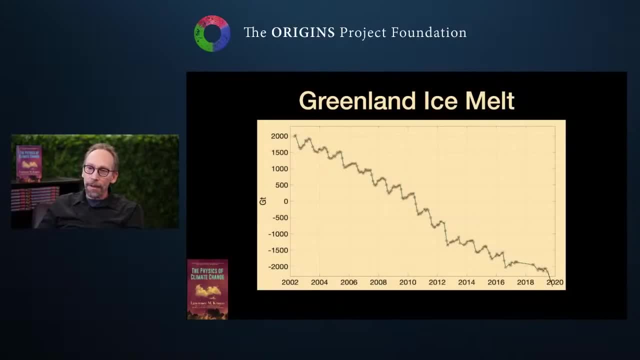 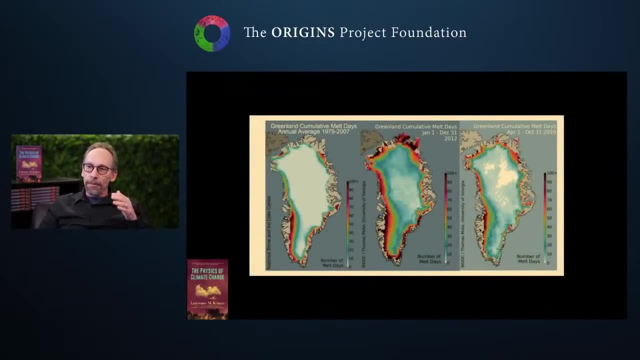 and in fact, if I put one more curve on here in 2019, and it's melting, it turns out that melting is accelerating And if we can see that, here's the average cumulative number of melt days And you can see in the 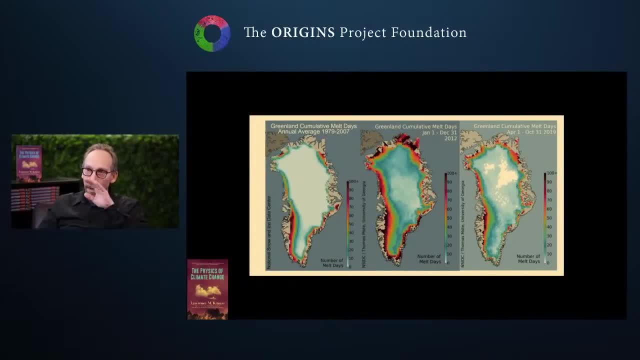 white and blue is a low number And as you get to green- I think I'm color blind- you can see the number gets higher. And if you take the average between 1979 and 2007,. there's very little green. 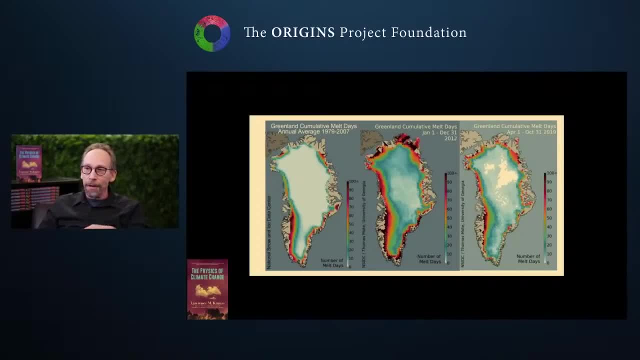 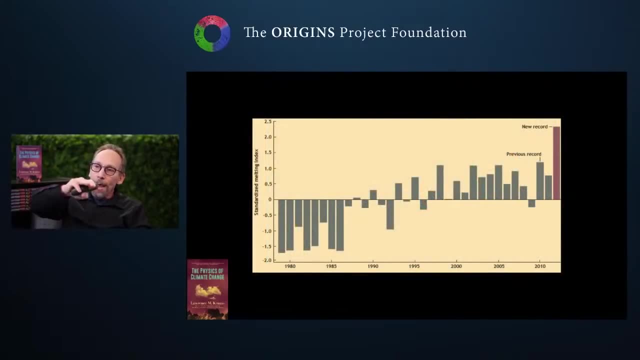 But already in 2012, there's a lot, And 2012 is a big year. 2019 is an equally big year. There's a lot more ice melting And this is maybe this is a standard index to show you again, if you look at, 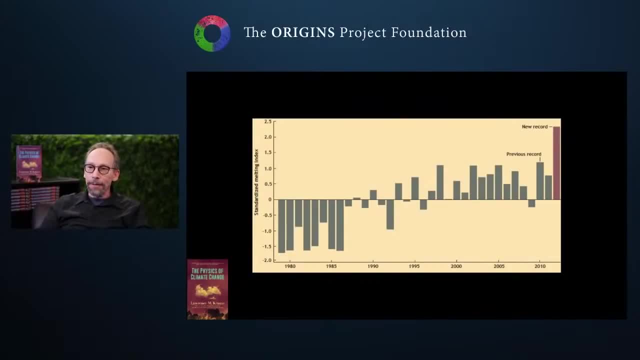 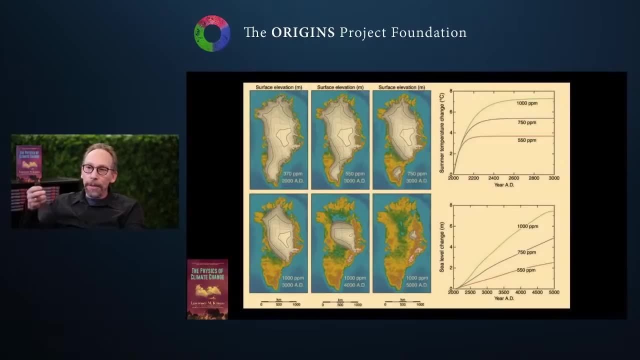 that it's clear that Greenland ice is melting at an accelerating rate. Now you can do some predictions and say well, how much in the year 3000 AD, in 2000,. at 370 parts per million, that's the amount of ice. 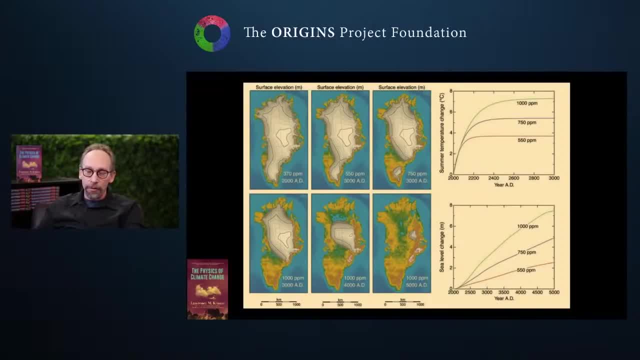 in Greenland. How much ice will be in Greenland in 3000, a thousand years? if we do business as usual and we turn things off at 2100 at about 500 parts per million, Well, the Greenland ice sheet will have decreased. 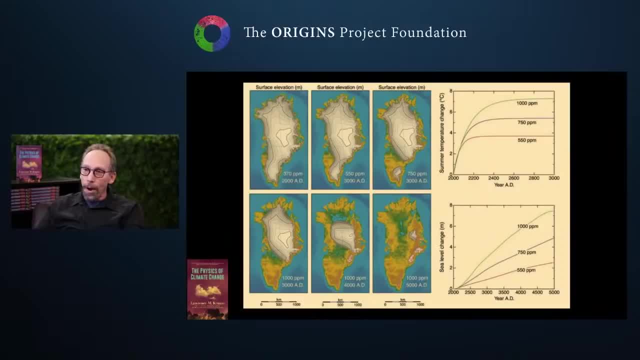 by that amount which will have, if you look at the sea level rise, it will have corresponded to that will be around several meters. If we increase it to 750 parts per million by 3000, then more of it will have melted And 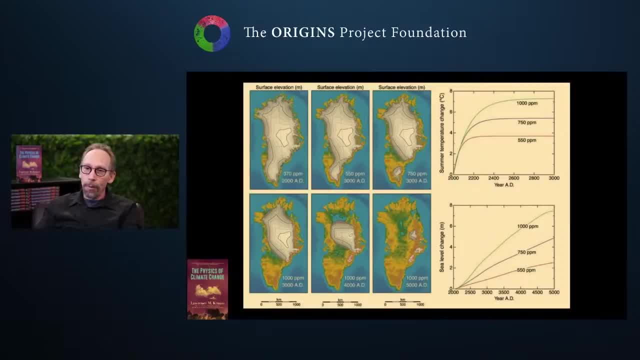 you can see now you've got three or four meters ultimately of sea level rise And it turns out- we know for certain- that if we go up to somewhere between 750 and 1000 parts per meter, there's a tipping point That nothing you can do is going to stop. 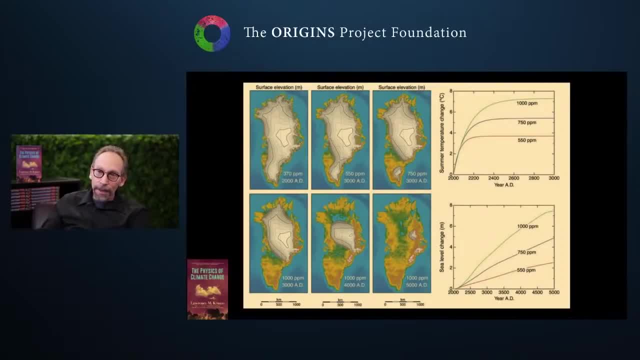 the Greenland ice sheet from melting. And over several millennia the Greenland ice sheet will melt. And if the Greenland ice sheet melts, that's seven meters of sea level rise. And it's happened before. it's happened more than once before, as I'll show you. Let me just go. 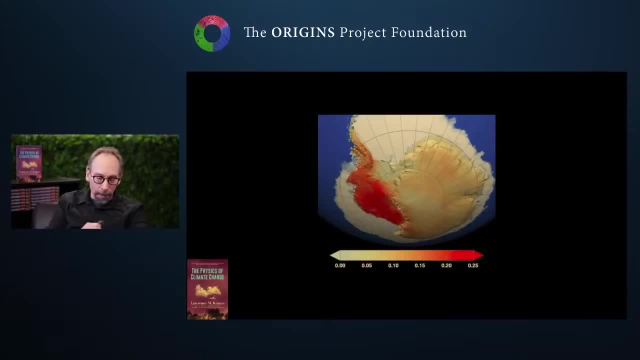 to Antarctica. before I show you some of these, before I try and summarize. This is the average temperature change in Antarctica and you can see the West Antarctic ice sheet has heated up a lot In recent times and my wife and I were fortunate enough. 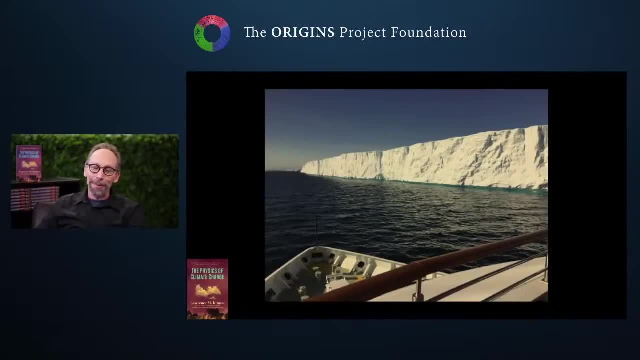 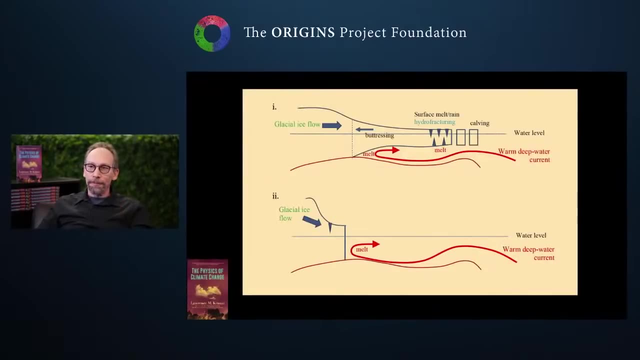 to go there. this is a picture I took from our boat. This is a small iceberg, you can see, and the effects of global warming are significant in Antarctica for the following reason: This shows you: there are these big. there are these big. 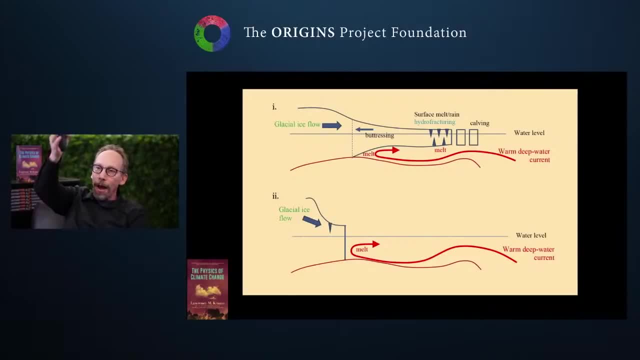 icebergs calve off these large ice sheets floating on the ocean. Now, when the ice sheets calve off into an iceberg, sea level doesn't rise because the ice sheet is already floating, But what happens is, as warm water melts, that that ice sheet itself disappears. 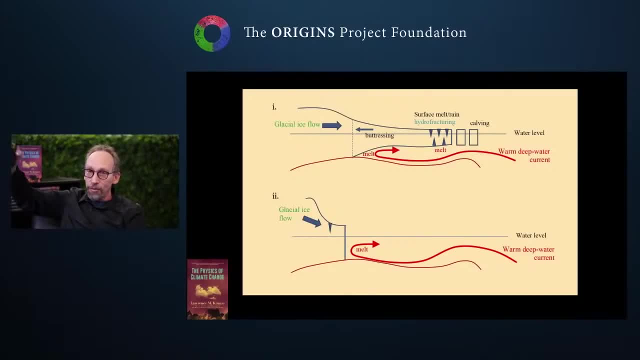 and a huge, basically all of that ice shelf disappears, And we've seen that happen a few times in Antarctica in recent years, And when that happens there's nothing to hold glacial ice black. It was flowing but it was buttressed before. 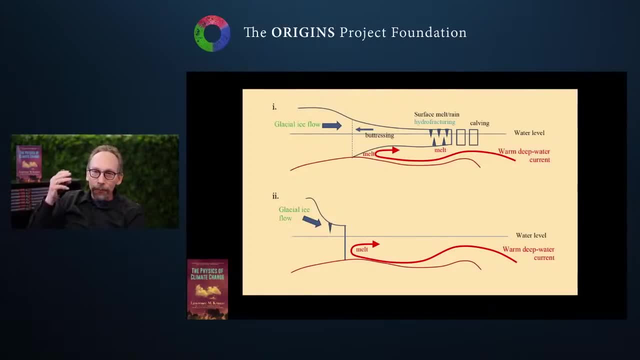 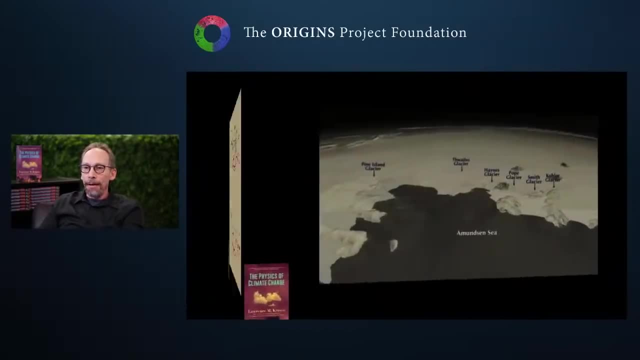 by the ice sheet? Now it's not. and then it flows and that flow has been accelerating in Antarctica, And when that ice goes into the ocean, that raises sea levels And unfortunately we're seeing that happen in a variety of places and in fact it's quite 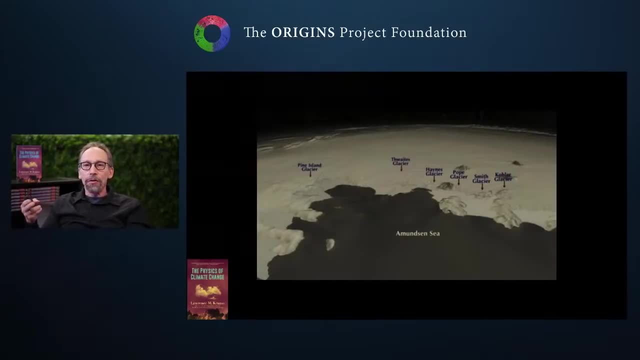 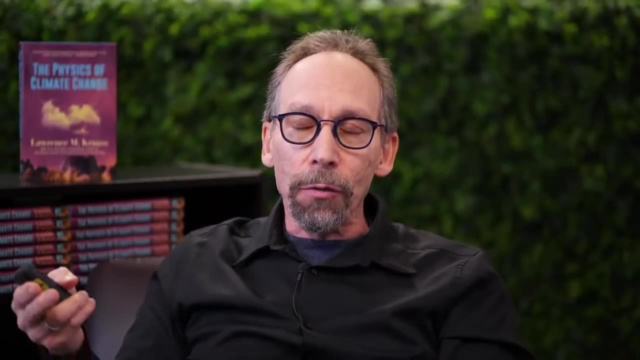 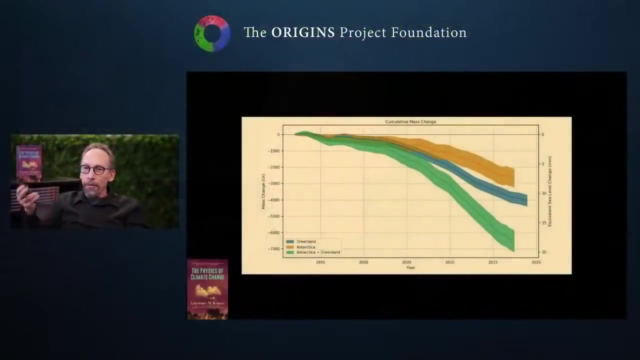 people argue, we're already at a turning point where the ice sheets are disappeared and these large glaciers are going to flow into the water and could produce, over the course of centuries, a two to three meter sea level rise. You can see. here is a summary of 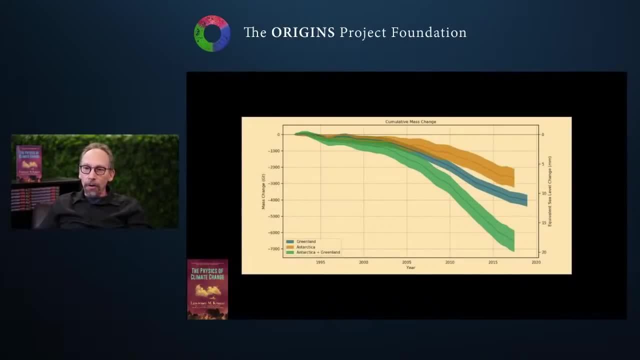 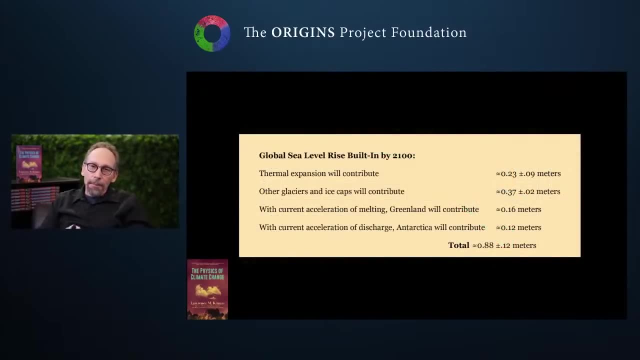 the mass change in Greenland, Antarctica and the two, and you can see that basically it's accelerating, It's melting down And here is a summary now from the National Academy of Sciences of basically what we expect for sea level rise. It's built in No matter what. 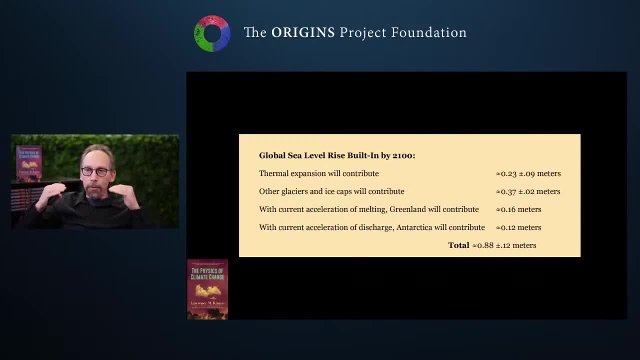 we do basically what we've done already. the heat we've already put in, thermal expansion is going to produce about 0.23 of a meter. Glaciers and ice caps will do 0.37.. If the current acceleration of melting 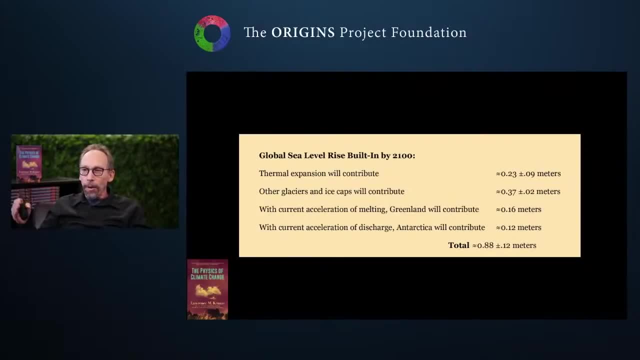 that we see in Greenland continues at its current rate, it's going to produce 0.16 meters about, and similarly in Antarctica. the total you get is about 0.8 meters, So more or less close to a meter of sea level rise. 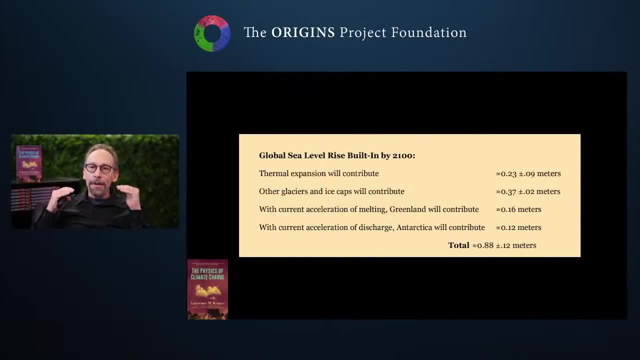 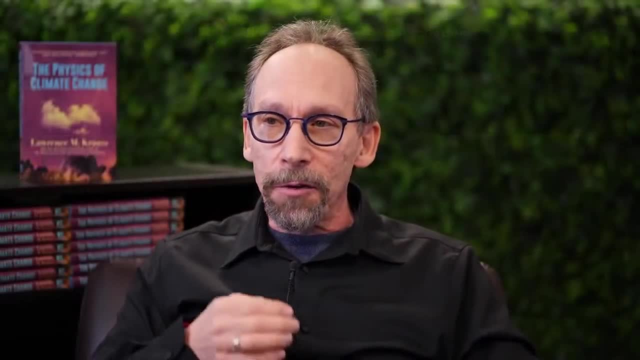 is built in. This is not speculative. It's going to happen Somewhere between half a meter and a meter. Now that may not seem like a lot. Half a meter, a meter sea level rise by 2100.. Why are we worrying? 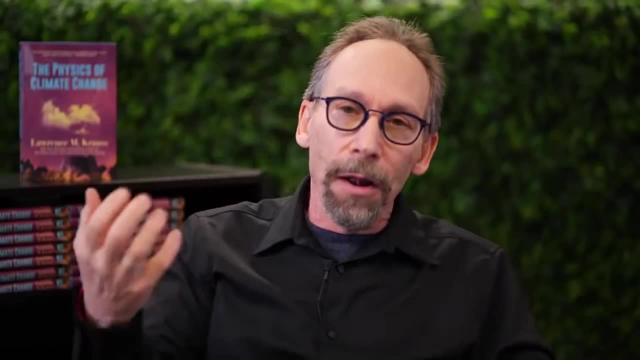 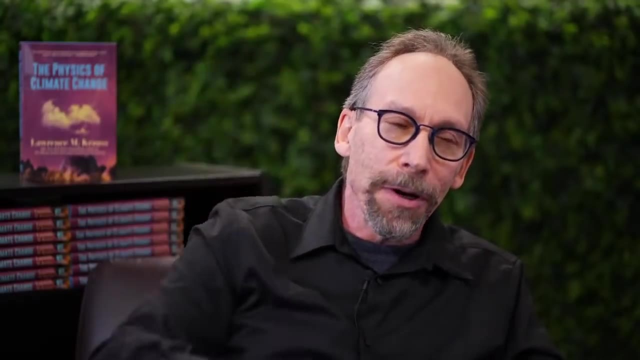 about that. Well, it depends where you are. It's all relative. A meter may not seem very high, but if I take a bowling ball and hold it a meter above your foot, it seems pretty high. And this before I go back. I want to say that 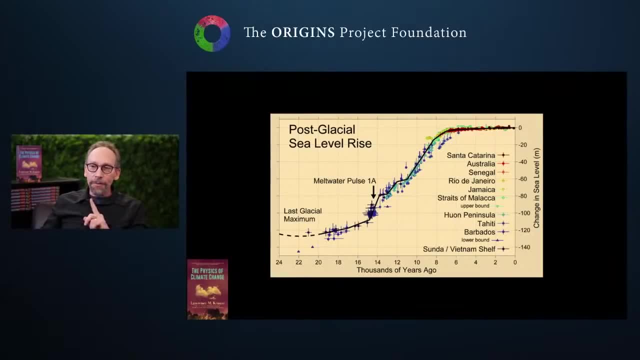 this meter is one thing. If Greenland melts, we'll see 7 meters, And sea levels have already been known to change by much more than that over even thousands of years of history. You can see around 15,000 years ago as we. 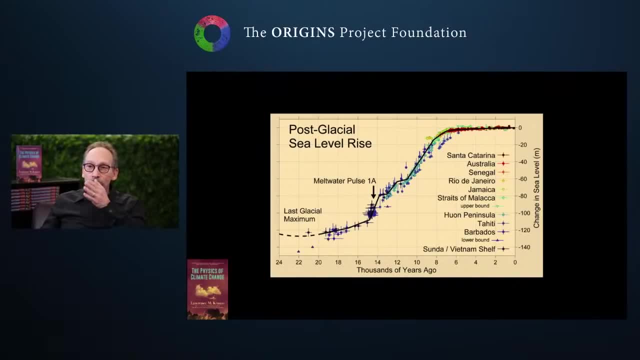 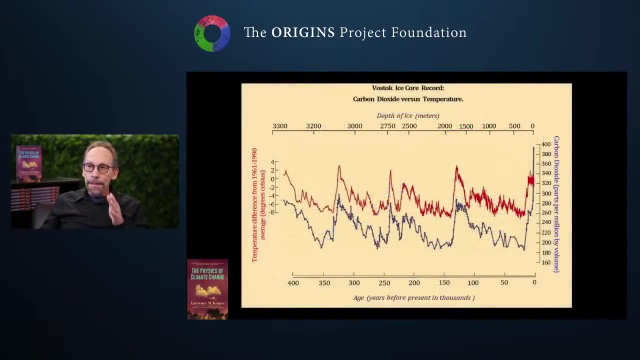 left a glacial period and heated up. there was a huge melt, motor pulse and actually sea levels rose by 20 meters over the course of several centuries. So sea level rise that's large, can happen over centuries And I want to show you a curve that. 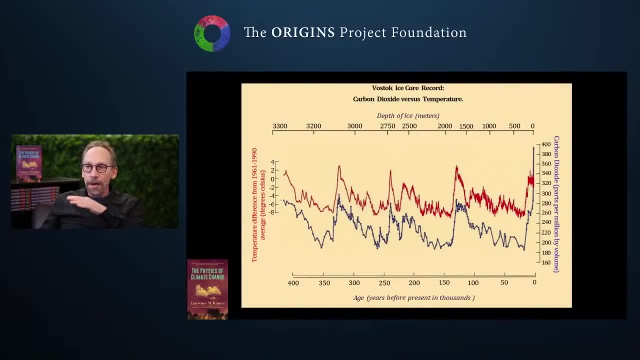 really woke me up about 10 years ago when I started to think: how serious is this? This is what I showed you earlier. This is basically a correlation between carbon dioxide and temperature as measured from ice cores down to 400,000 years ago. 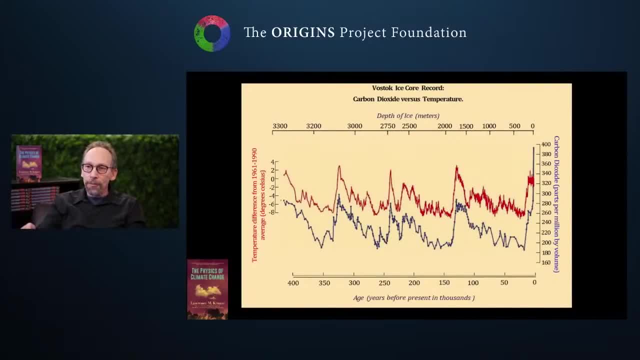 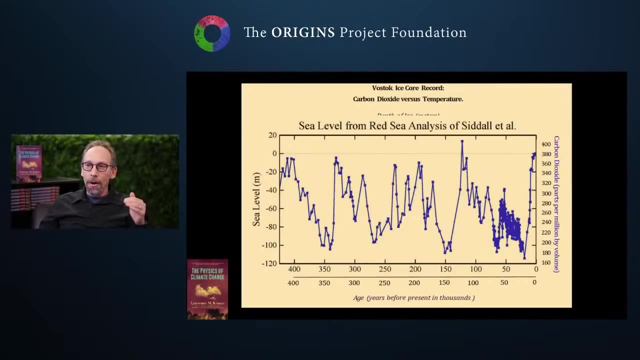 Now let me exchange for that from the Red Sea measurements of sea levels, And you can see a correlation between those things and sea levels on Earth changed by not one, not 10 meters, but 120 meters, as temperature and carbon dioxide changed. So we're talking about 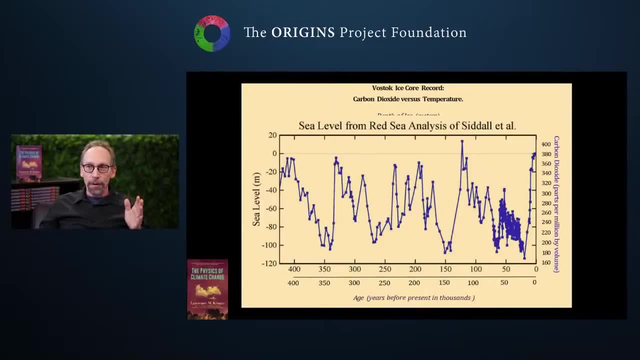 a change that's unprecedented in the amount of carbon dioxide in the atmosphere, temperature changes that are unprecedented, potentially, in the last few 400,000 years. and one meter may, in the end, seem like it's very small compared to what might happen, And this was the figure. 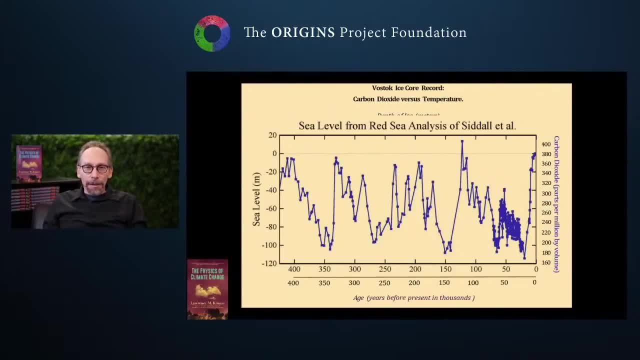 that reminded me of that Clint Eastwood movie where he says: are you feeling lucky, kid? Because ultimately, when you ask yourself what are the likely risks, What's possible And what can we do, Well, you say this kind of thing may not be written. 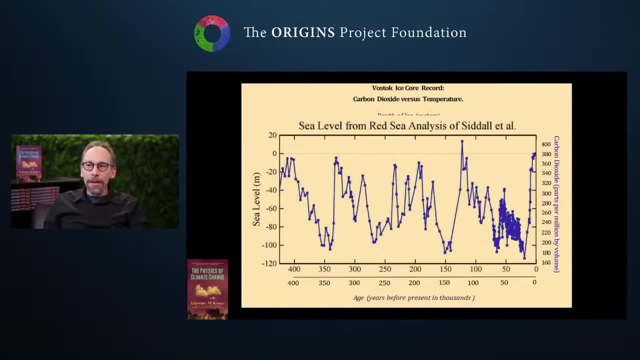 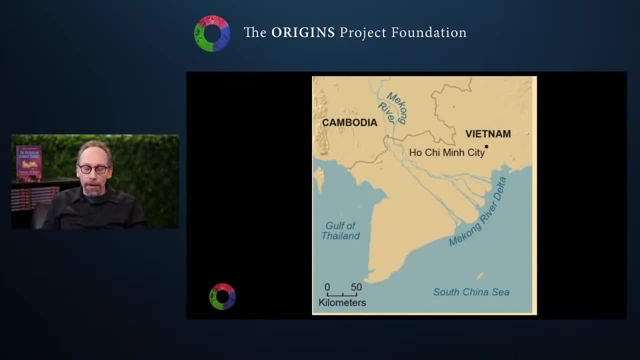 in stone. one meter is written in stone. but is it worth the possibility that we may have something much more severe, or is it worth thinking of innovations that can get rid of that? Now let me, as I wind down here now, let me end by: returning to the Mekong River, because I just want to summarize what's going to happen there in the near term. The Mekong is the richest density of freshwater fish in the world. in that river, Over a thousand species of fish expected, some not yet discovered. 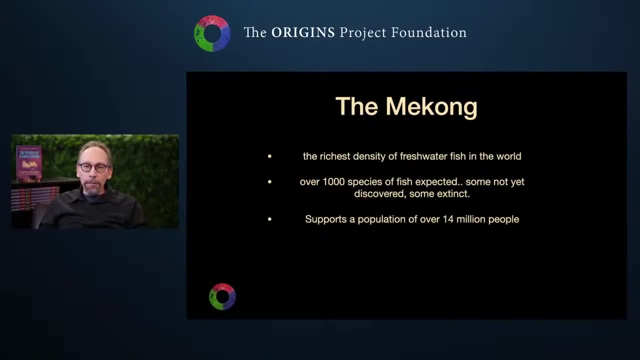 and some extinct. It supports a population of over 14 million people directly, and then rice growing will be even more. A greater volume of freshwater fish is harvested from that Mekong than all the rivers and lakes in the United States combined Now. 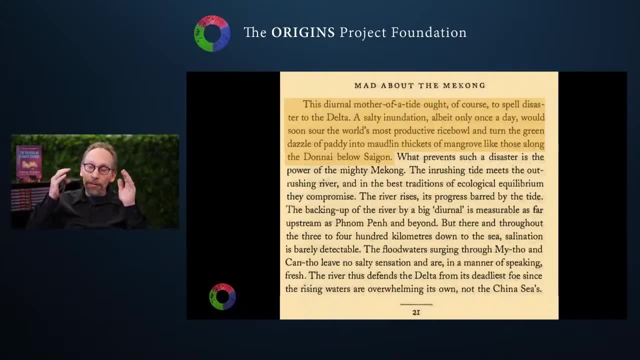 here is the problem. There's a large tide. it turns out once a day, and at the beginning of the Physics of Climate Change book I explain how you can get a once a day tide instead of a twice a day tide. That would spell disaster. 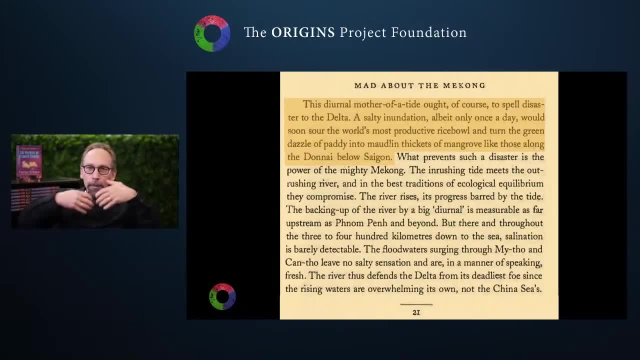 if it wasn't held off by the river, because if it produced a brackish water, if there was salt water coming in, that the richest rice harvesting region in the world would become brackish and instead of having a rice bowl, you'd have mangroves. 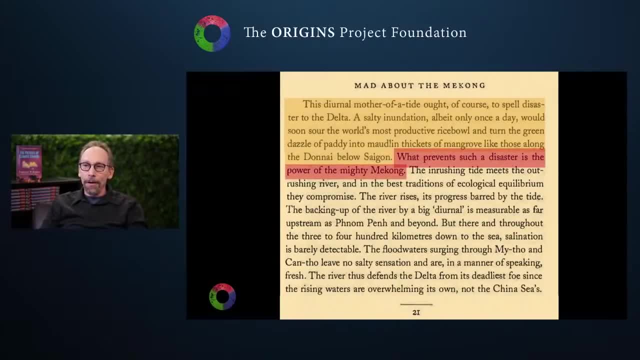 What prevents the disaster is the power of the mighty Mekong. This is not from my book. this is a book called Mad About the Mekong, about the first time the Mekong was mapped in the 1860s by a French. 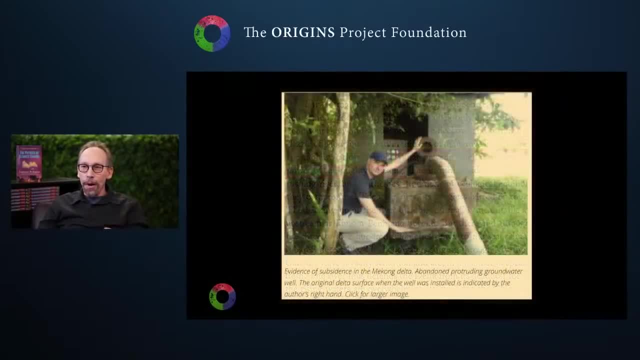 group And the problem is sea levels are rising. Philip Minderhoud was the first person to basically realize that the actual elevation level in South Vietnam has two problems. First of all, it's subsiding due to water usage and due to the fact. 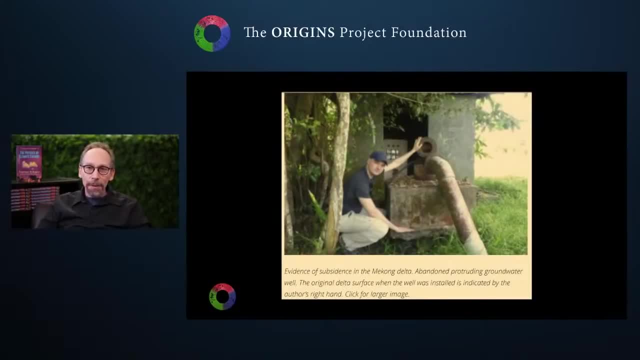 that the Mekong River is being. a lot of it is being. the depth of the Mekong River is going down because sand is being taken up. He shows with his hand where the zero level was when, at the time, that pumping station was built, and you can see it's. 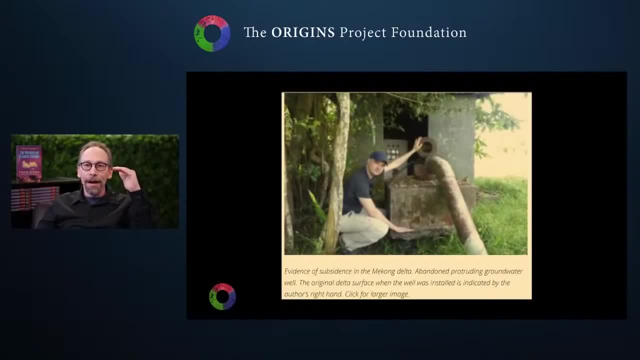 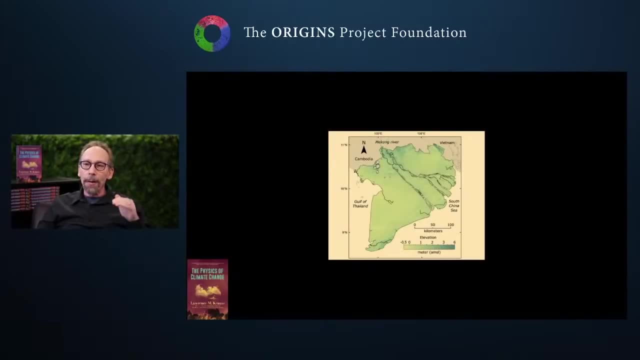 much lower than that now. but he also realized that satellite data of the elevation of South Vietnam was wrong And in fact, 95% of South Vietnam is less than one meter above sea level, So that, if you look, this is a paper that came out in Nature earlier in the year. 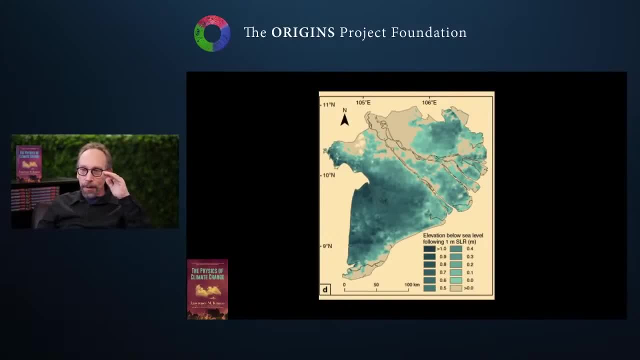 if you look at the dark regions here- regions the amount of South Vietnam- that'll be more than half a meter below sea level. if there's one meter of sea level rise, 95% of South Vietnam will be below sea level And, interestingly, 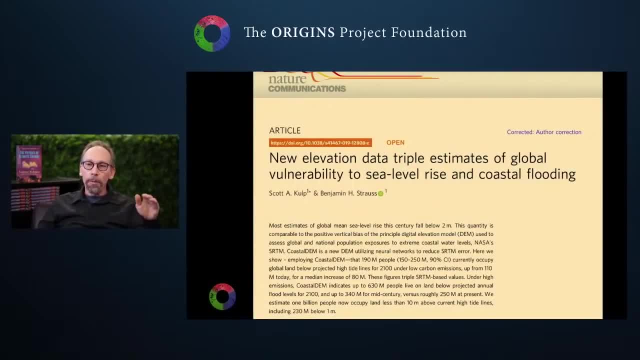 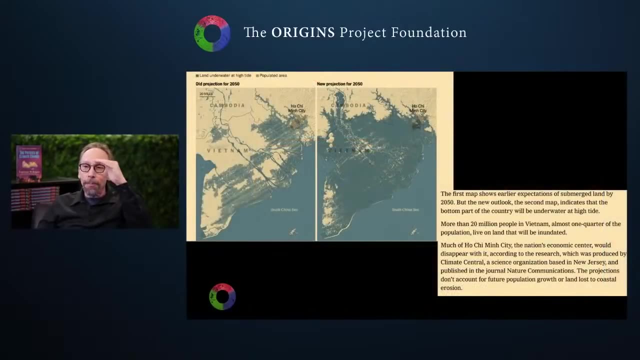 enough. independently, another group looking at satellite data and realizing that satellite data of the surface of the earth was wrong, was systematically in error, gave new estimates of the elevation of much of the earth's surface, and then they came up with a number that's exactly the same as Minderhut in. 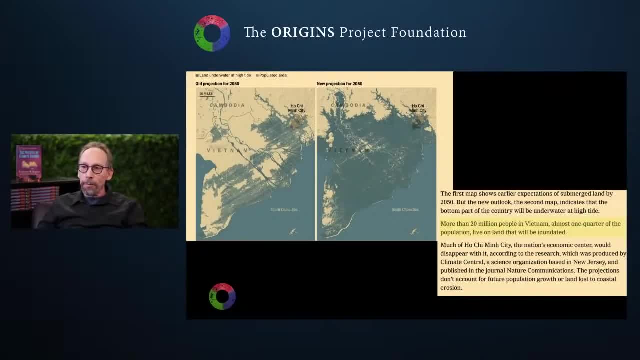 South Vietnam, And they said more than 20 million people- one quarter of the population of Vietnam- will live on land that's going to be inundated by 2050 in high tides. Much of Ho Chi Minh City, where we visited last year, will be below sea level. Of course, 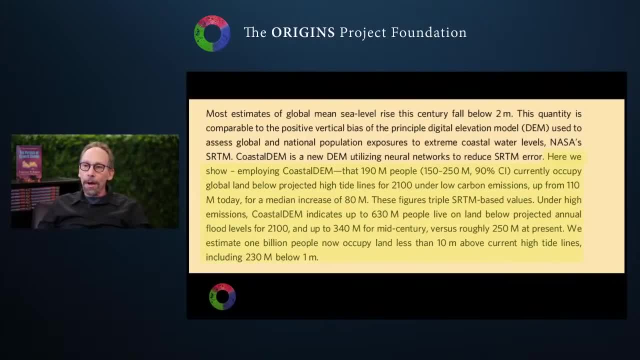 unless we do something. But this isn't just South Vietnam. If you look at it, if we turn things around and don't emit much carbon dioxide in the atmosphere, stopping it around 2020 to 2030, 190 million people around. 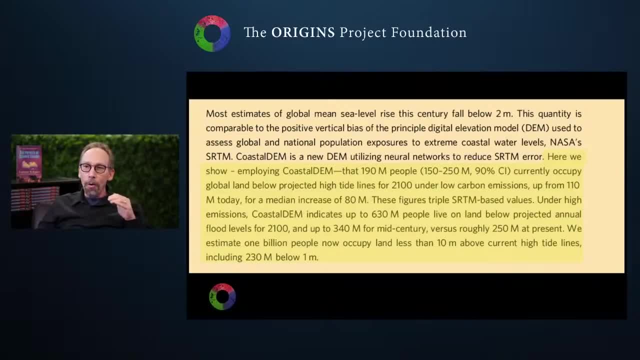 the world currently occupy global land that's going to be below high tides in 2100. And if we don't stop things in the next decade or two, we have business as usual. then up to 630 million people live below land, on land below. 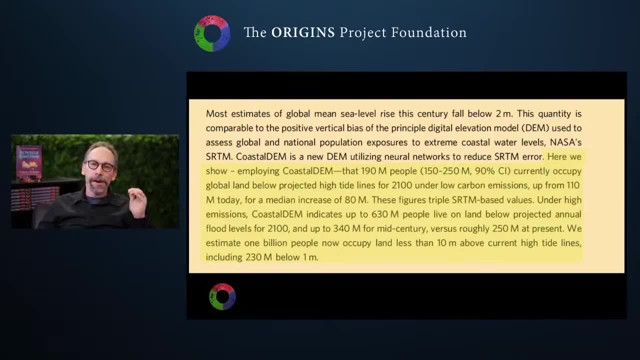 sea levels in 2100.. This is a global effect. No places in Ireland, And it's sad that the most significant impact is going to be in, probably in places that are least likely to be able to do something about it. South Vietnam is now getting richer, maybe. 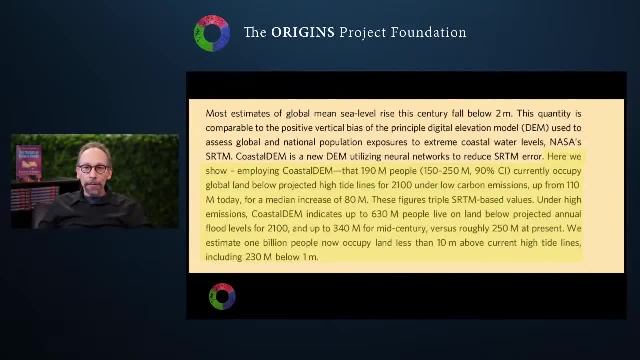 with enough anticipation they can build dikes to put this back. After all, much of Holland is below sea level. But a lot of the world's population won't have the resources unless the industrialized world helps. And when I was a kid my parents had a little store. 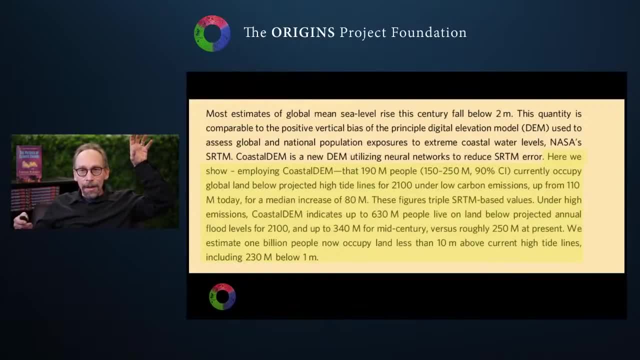 and there were trinkets and I used to work there and there was a sign saying if you break it, it's yours, And in some sense, the carbon that's already in the atmosphere was produced by the industrialized world and maybe 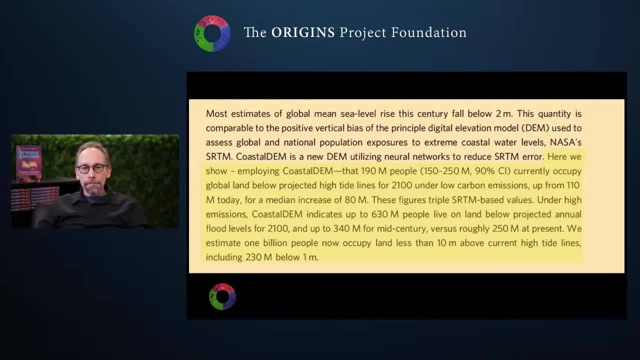 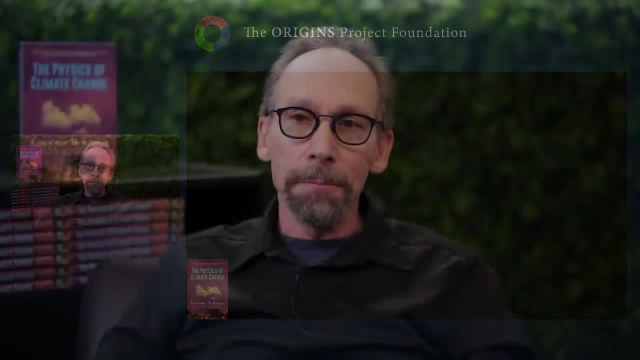 you could argue we have an ethical motivation, or maybe obligation, to help those regions of the world that are going to be affected because of the built-in effects of climate change. Now, I don't want to end this on a downer. There are some various impacts. 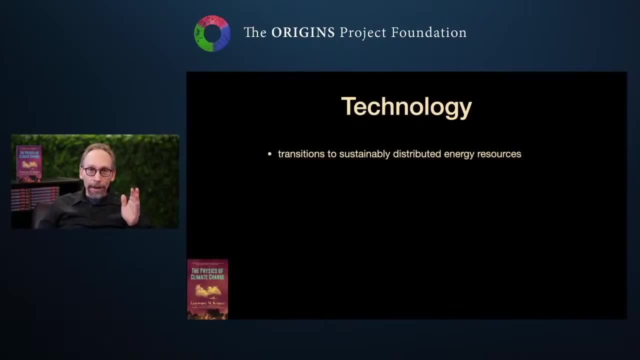 but technology allows us a great deal of possibility. Technology can help us. We can make transitions to sustainable energy. We can do infrastructure improvements in South Vietnam and other places around the world if we want to. There are already climate refugees in South and Central America that are coming up to the. 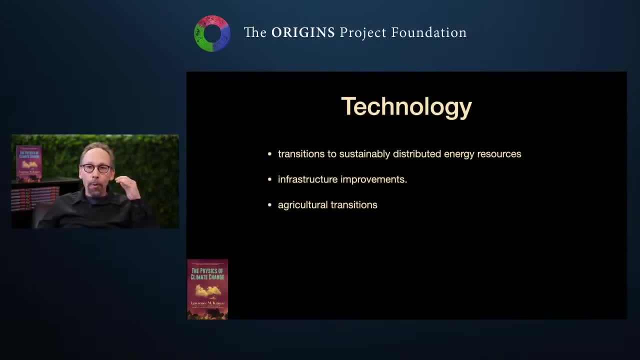 United States because of the likely effects of climate change. But one of the ways we can help stop that flow of immigrants is to provide industrial tools that we already know how to grow more with less In the industrialized world. if we export those techniques, then we can. 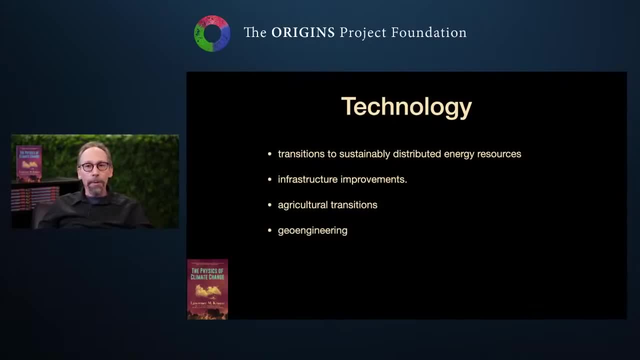 mediate the effects of climate change a lot. One possibility that's been suggested is geoengineering, and that is to basically put aerosols in the atmosphere that will potentially absorb or reflect sunlight. It used to scare me a lot, but my friend Dan Schrag, who I did an 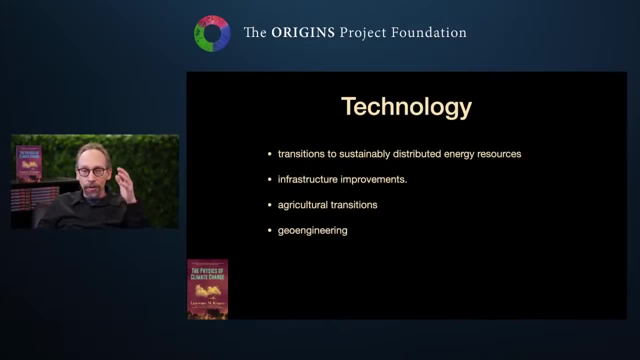 Origins podcast with who's a climate scientist has pointed out to me that those aerosols remain in the atmosphere only about a year or so. So even if we screw things up, it only lasts for a year. Or maybe we could try global carbon capture, I know. 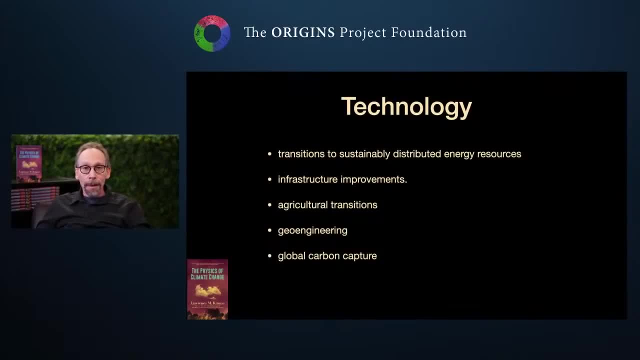 that Elon Musk has made a big prize and I've been involved earlier, at my last university, in a project looking at global carbon capture. It's quite a challenge And maybe in the question and answer period I'll talk about what a challenge it is, But I've already gone. 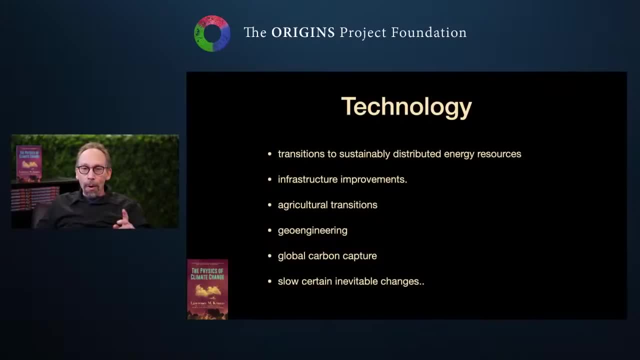 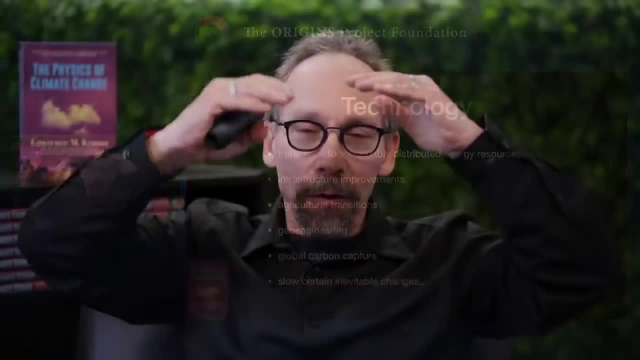 an hour and six minutes, so I want to end up here. But what we can do is slow inevitable changes. If we decrease the rate of carbon increase in the atmosphere, we can stave off sea level rise- We can stave off. 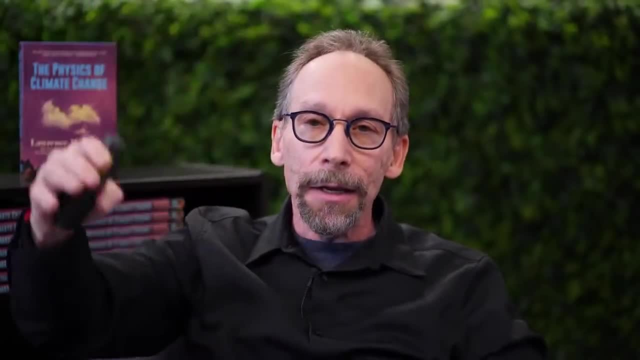 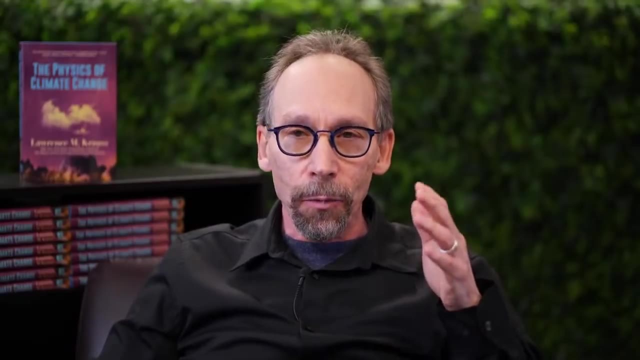 Greenland melting for not just centuries but millennia, giving us time to react. So technology is not the problem. The problem is probably politics, And that's the reason I'm giving this lecture, That's the reason I've written this book: Understanding the science of climate change and its 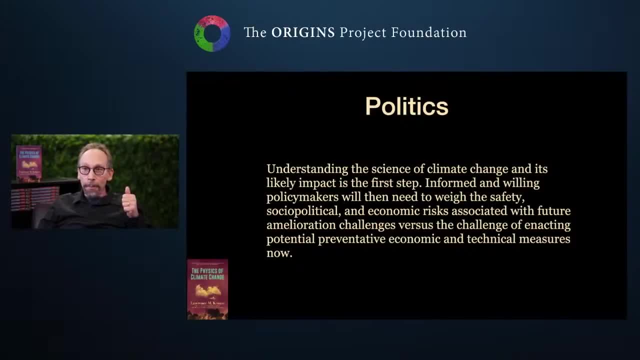 likely impact is the first step, And informed and willing policymakers will then need to weigh the safety, socio-political and economic risks associated with future amelioration challenges versus the challenge of enacting potential preventative measures now. And politicians don't lead, They follow And the 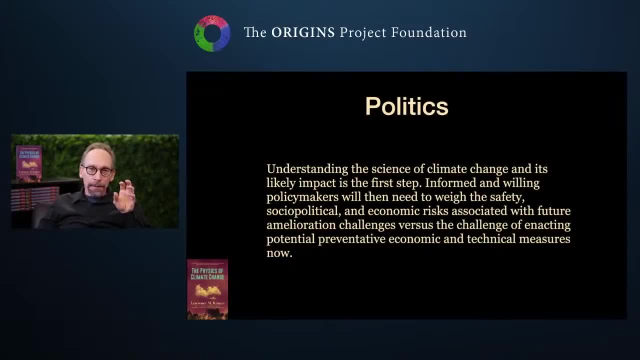 only way they're going to act is if we all demonstrate that this is a serious issue in the voting booth and in the other things we do. So what I wanted to provide you was the science. You can decide how severe you think the problem is, but 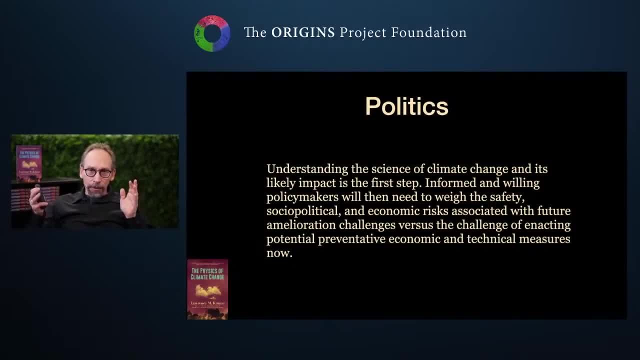 you can see that the science is fundamental, understandable and certain things are inevitable. I talk in the book about, like Charles Dickens, the ghost of Christmas past and the Christmas future, the future as it might be versus the future as it must be. And 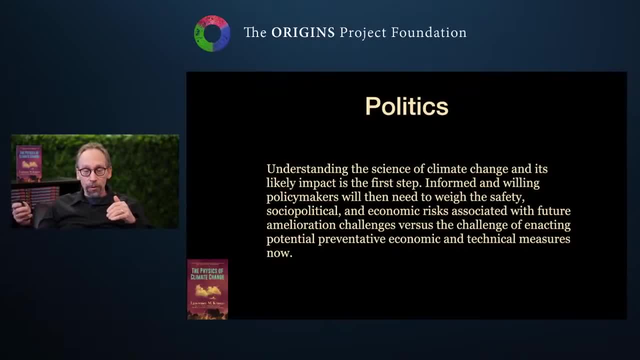 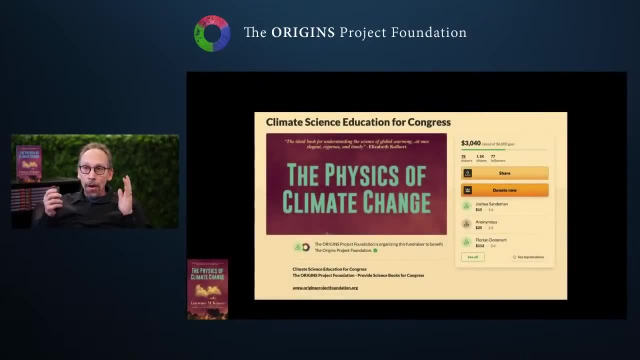 there are a lot of potential things that are much worse than one meter sea level rise, but they're more speculative. The question is, are we feeling lucky? One of the reasons, one of the ways you want to educate Congress, the foundation that I lead has 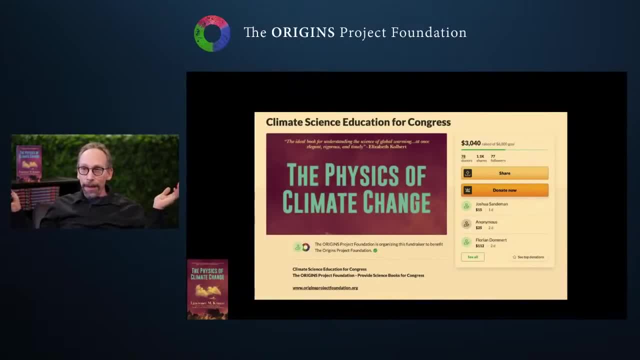 just started and we're planning to. we just got the books here. we're planning to send copies of the Physics of Climate Change, which is a science, to every member of Congress And we're trying to raise money to do that. We've raised 3,000 of the. 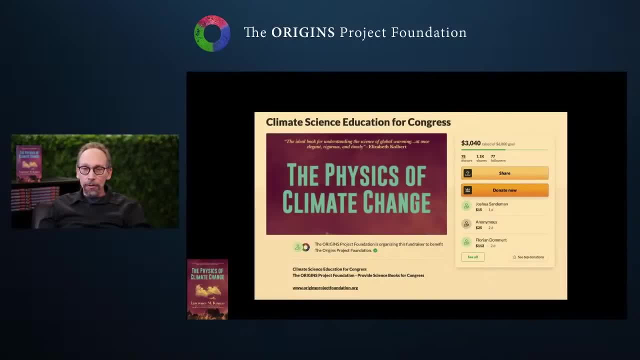 6,000. we need to do that. We're hoping people will continue to donate. We hope in the next couple of weeks to get those 600 books to members of Congress, not to lobby them for policies but just to educate them and hope that they. 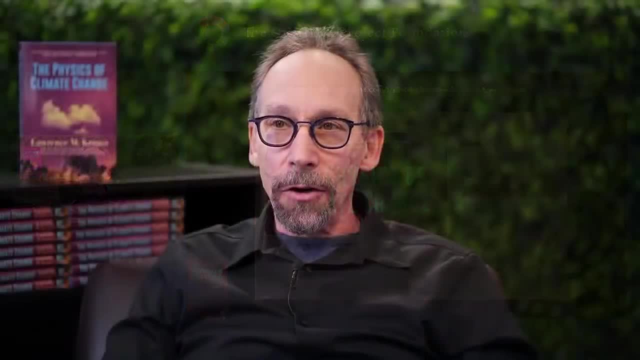 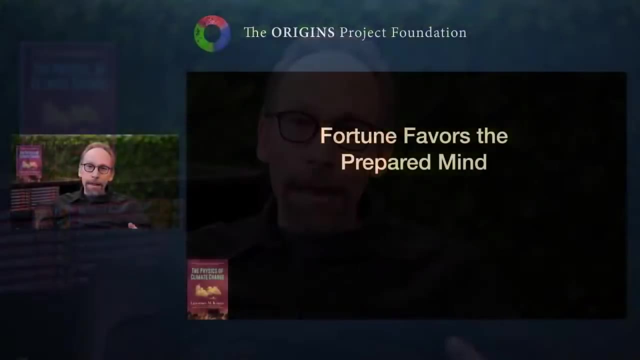 open them up or hope that their staffers open them up, And you can go to the GoFundMe site looking for climate education for Congress if you want to contribute. The epilogue of the book is called Fortune Favors the Prepared Mind. It's a statement by that. 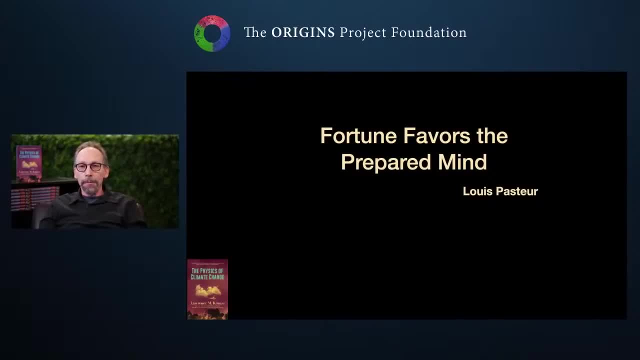 great scientist Louis Pasteur. And fortune does favor the prepared mind. It's one of my mantras. It doesn't guarantee us, It makes no guarantees about the future, It just offers better odds, And I'll take those odds. So, knowing what? 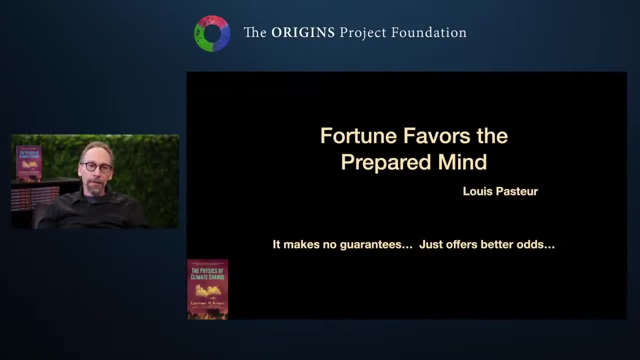 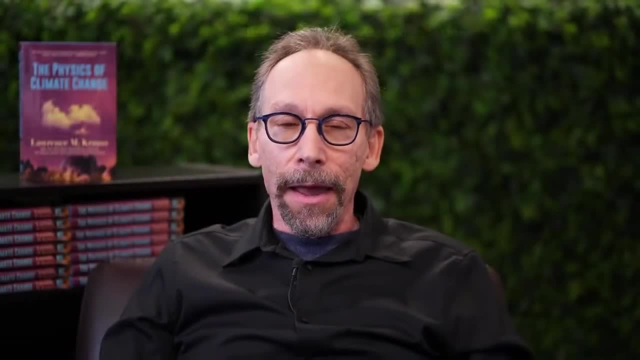 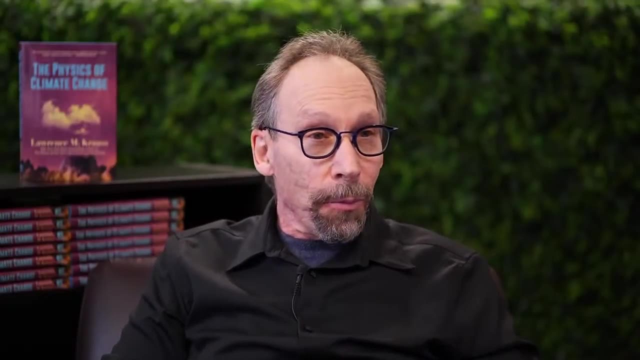 the science is and that will give us better odds to act accordingly to make a better future for us and our children. Thank you, And that's the end of the lecture. And now it's now 7.15 by my watch, And we're going to take a break. 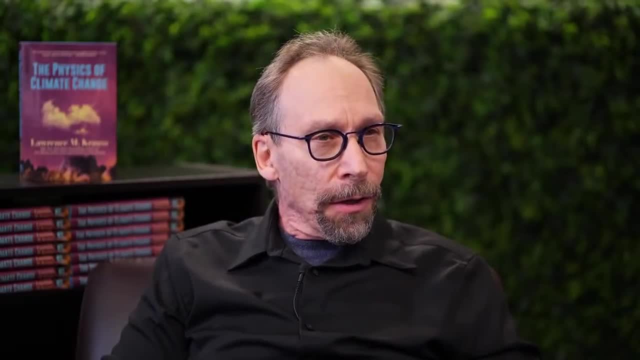 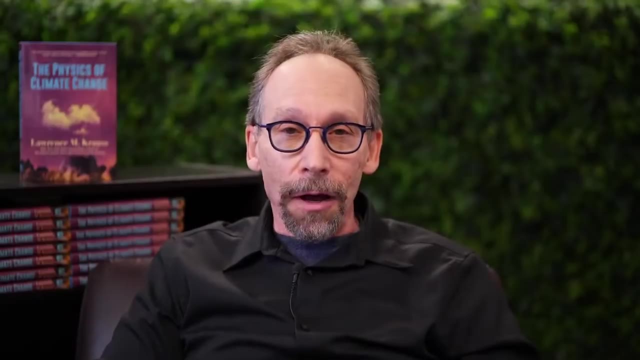 Is that right, Corey? We're going to take a break for about how long? Ten minutes, And some of you I'll see in a Zoom and I'll actually get to see you and we'll have a discussion And we'll go on as long. 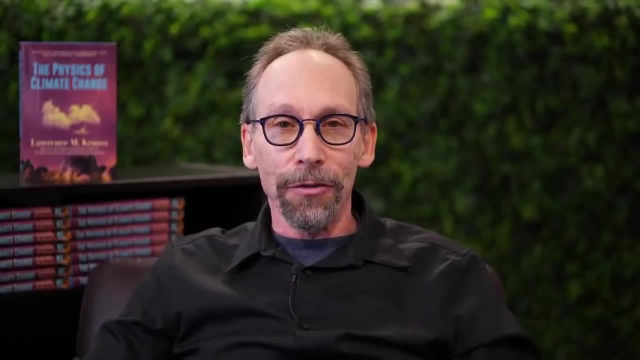 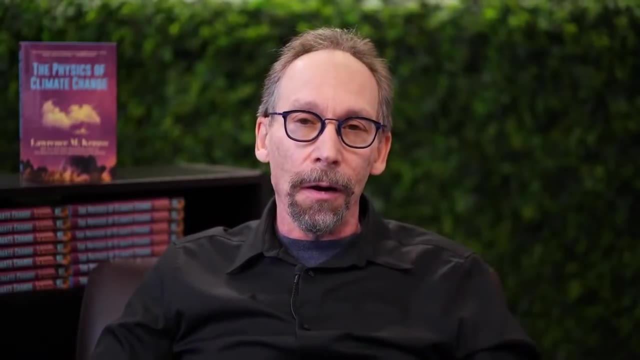 as you want: An hour, an hour and a half or maybe ten minutes, if you don't have any questions. So I hope this has been informative. We will be recording this and eventually streaming it and putting it on our YouTube podcast channel, which is part of the foundation.